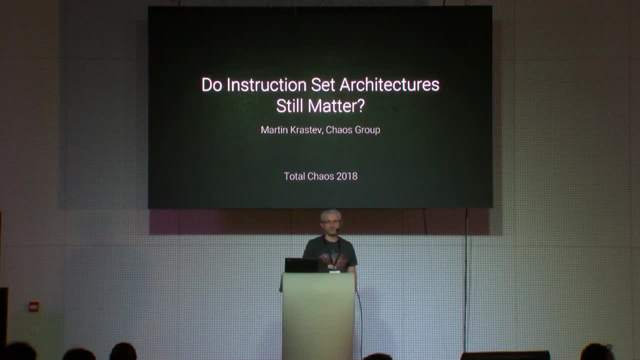 past five or so years And it's been a great pleasure for me to do that. I'm that kind of person. So the topic for today's lecture is, coincidentally, about low-level stuff just as well, And it's a sort of a rhetorical question that goes like: do instruction set architectures? 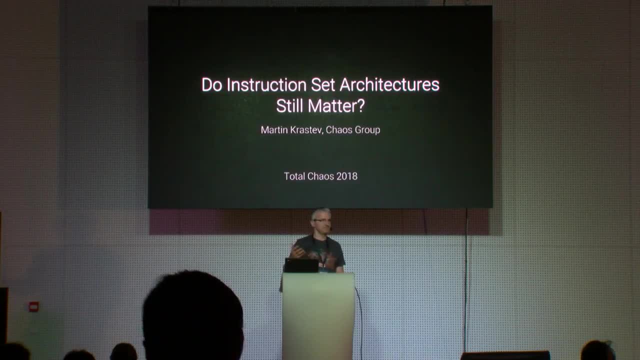 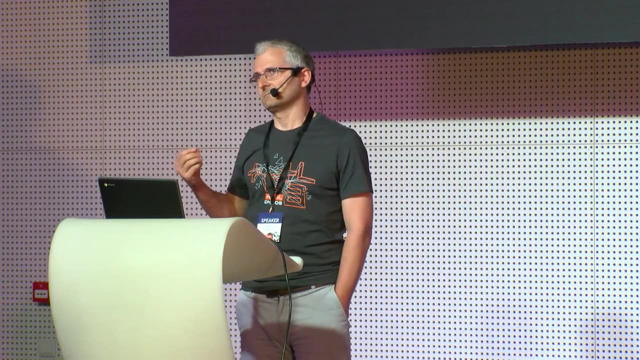 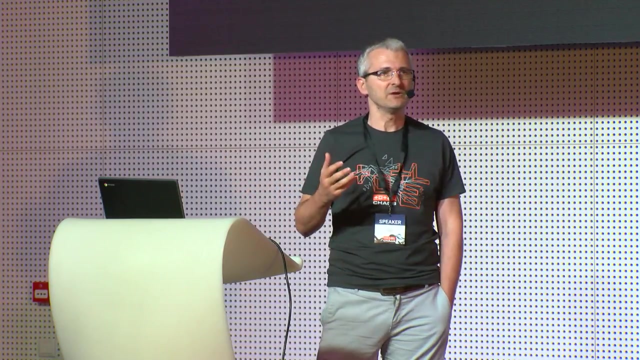 still matter. Now it is in a question form because there has been some kind of in the lecture space. there has been this notion that instruction set architectures have perhaps run out of their importance. I mean, it doesn't really matter The instruction set architecture. 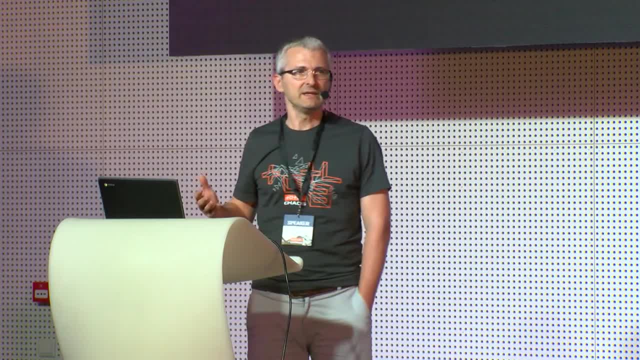 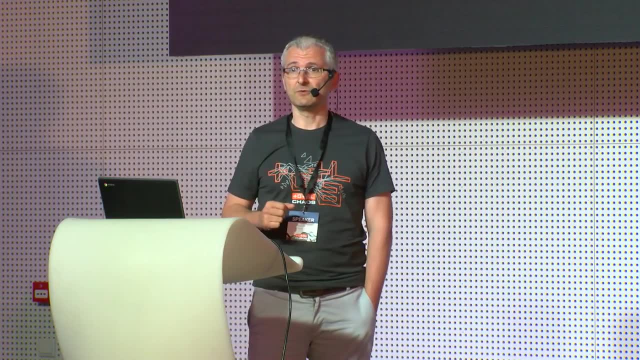 as long as you can parallelize, as long as you have backward compatibility, the instruction set architectures are not important. I'll try to show you whether that is the key So in this case, and leave the conclusion to your own. First thing first. what's an? 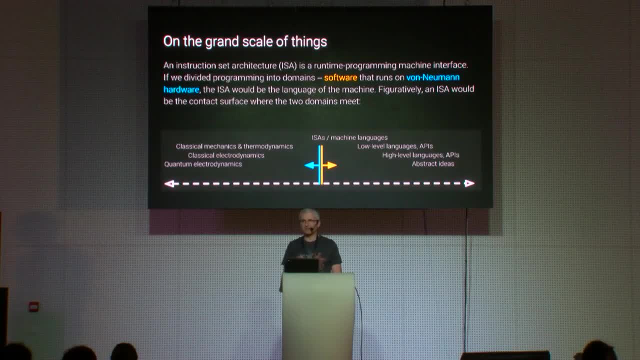 instruction set architecture. An instruction set architecture, or an ISA for short, is a runtime programming interface of a von Neumann machine. How many of you know what a von Neumann machine is? I'm glad that so many people know that fact. So basically, 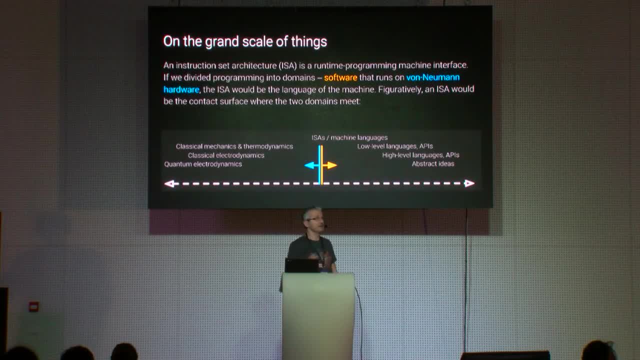 most of the computers around us today, in this age and day, are von Neumann machines, So what we're going to talk about here is related very much about the computers that you use in your daily lives. If we decided to divide programming into two major domains, 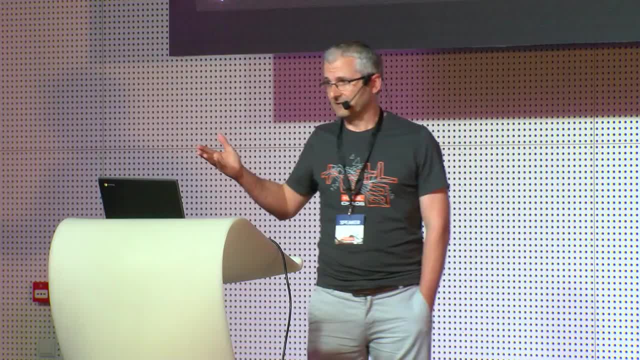 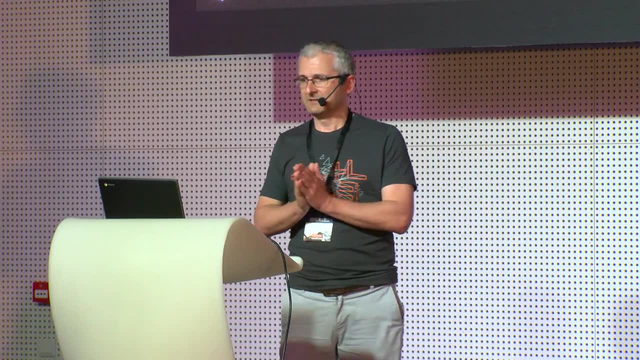 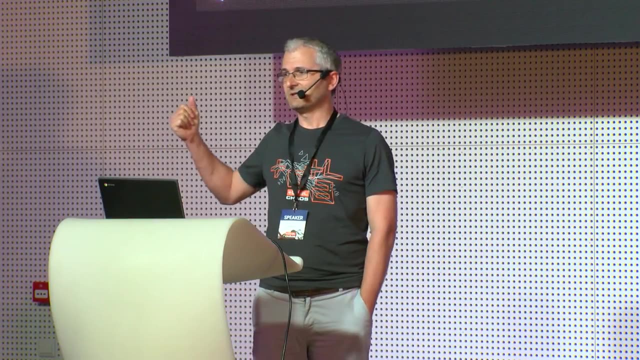 the domain of software and the domain of hardware, again von Neumann hardware, then the ISA would be the contact plane between the two domains. So here on that very simplistic diagram at the bottom, you see that if we start with ID, which is the domain of software, 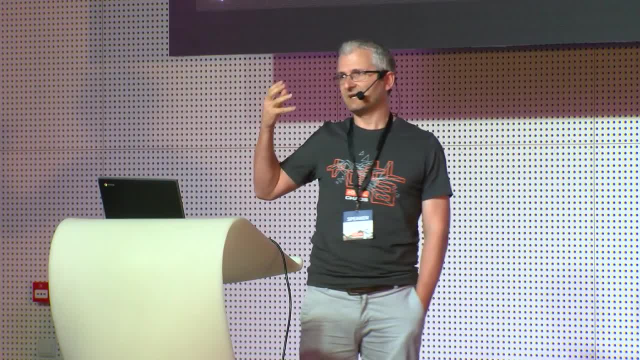 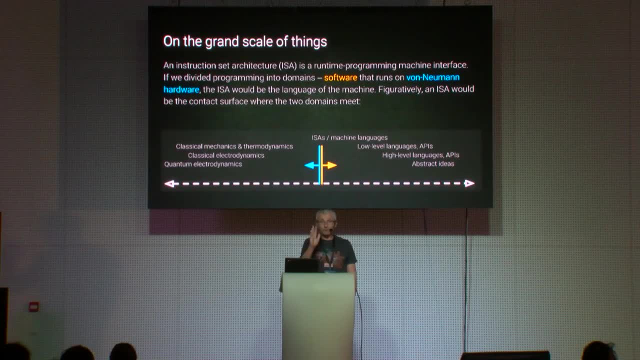 you get some very high-level ideas of the very high spectrum of programming, abstract ideas that we go down with high-level programming languages, some of the APIs, low-level languages and APIs. Then, before we get to the actual hardware, we get through the machine language. 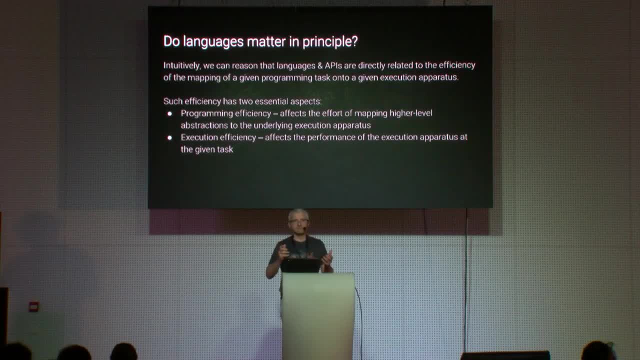 the ISA. Well, and here comes another very meta question: Do languages matter in principle? why do we care about languages in the first place? Well, intuitively, I think that most of us could reason that languages and their APIs are very, very small. That's quite obvious. We understand them very well. In fact, the main thing is that any of them can make a big difference at once and no, So we depend on scores that are important for our optimization, For example ESOs. For instance, what we thirty wirr ly Caran Clouden go to has an X worth. 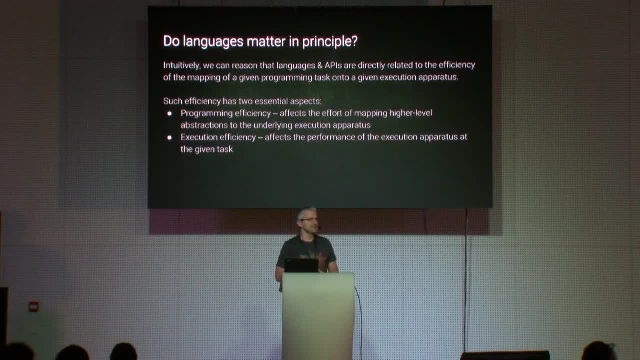 of course, are directly related to the efficiency of mapping high level of tractions to low level execution apparatus. Execution apparatus in this case is a fancy way to say computer. So such an efficiency usually has two major aspects: The programming efficiency and the execution efficiency. The programming: 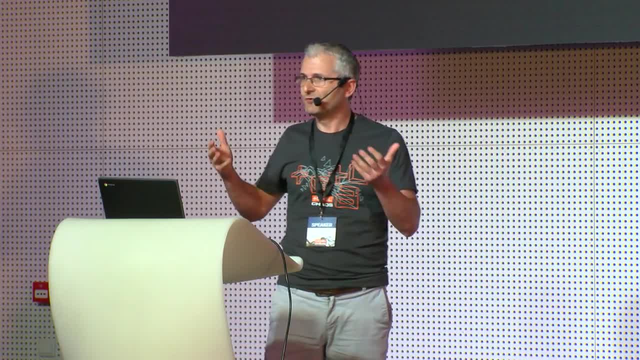 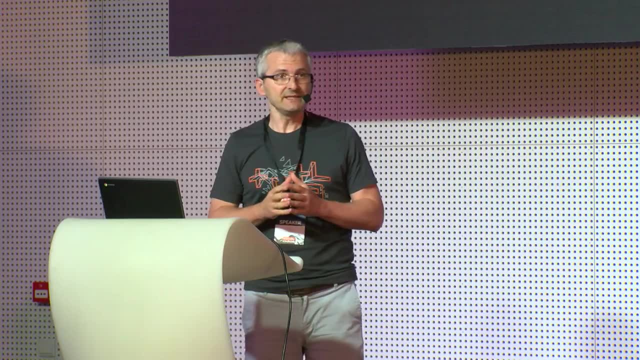 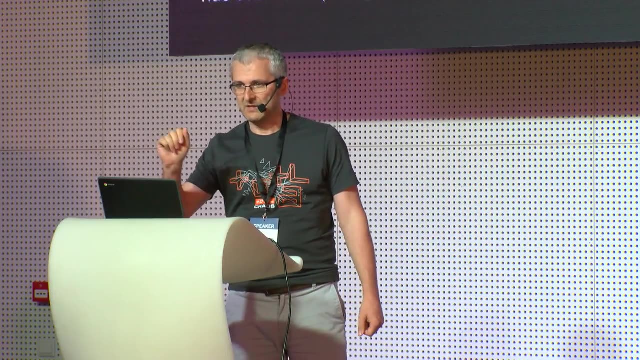 efficiency has to do with the effort that we as programmers have to put in order to get some abstract idea to execute on some piece of silicon. The execution efficiency has to do with how good the silicon is at running our idea. So again about programming efficiency. It wouldn't surprise anybody. 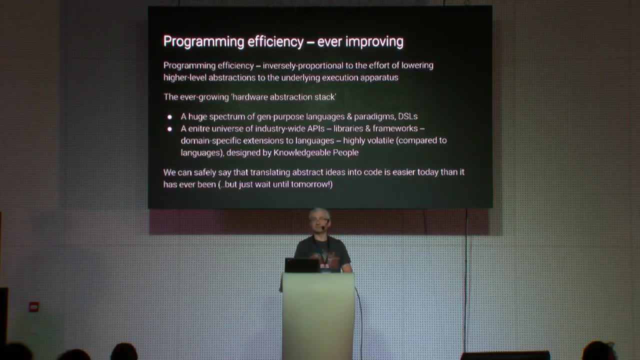 if I said that programming efficiency has been on the rise ever since computers appeared. So there's been this huge hardware abstraction level stack that has been growing and growing over the years, A huge spectrum of general purpose programming languages and their respective APIs, And by APIs I usually mean libraries and frameworks, Some very 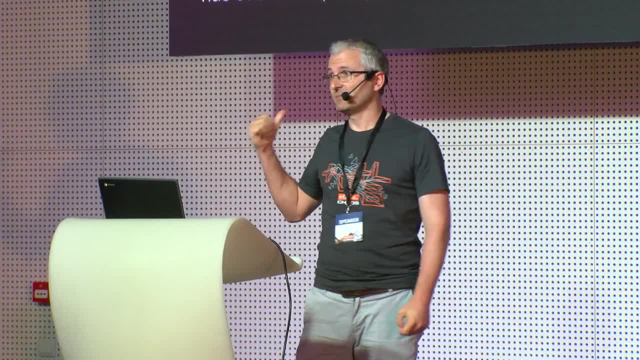 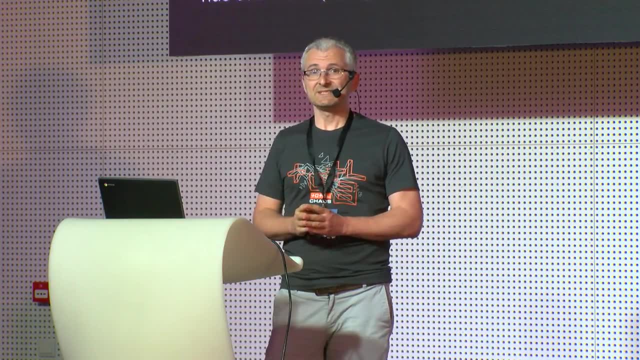 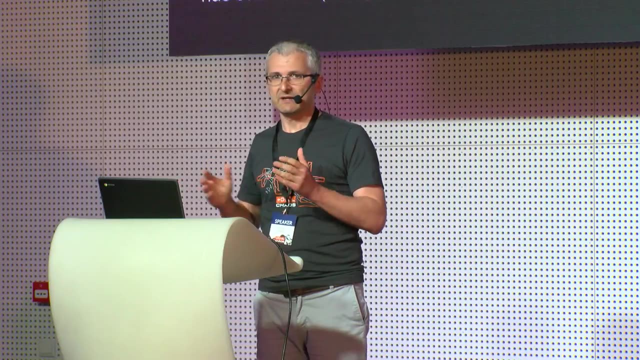 clever domain: specific languages. We just saw one presented by Arsene here in the previous talk. I was really, really fascinated by his talk. Then there is an entire universe of domain specific extensions to those languages in the form of libraries and framework. Now, what's specific about libraries and 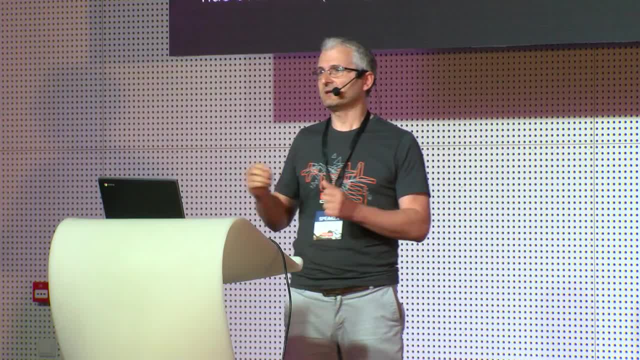 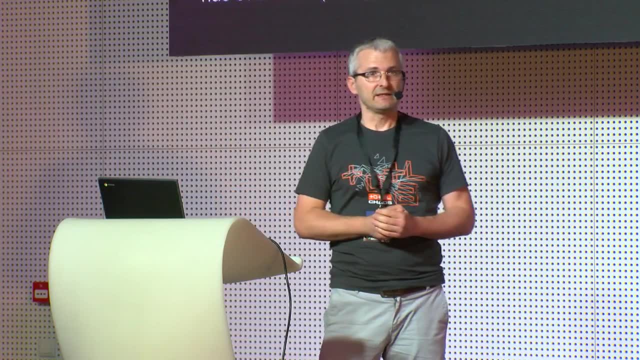 framework. What is a library and framework? What is a framework? What is a framework is that they're considerably highly volatile compared to the languages. Languages change much slower than libraries and framework change, And the other thing typical about libraries and frameworks is that they're usually written. 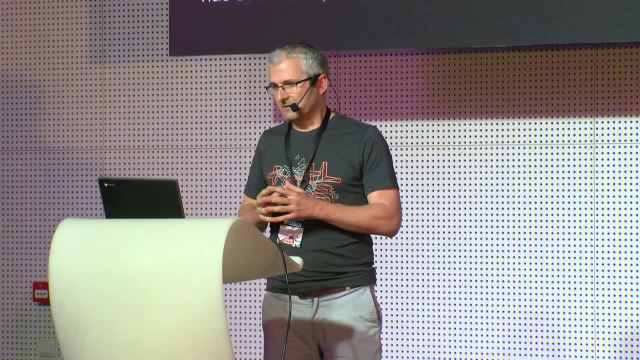 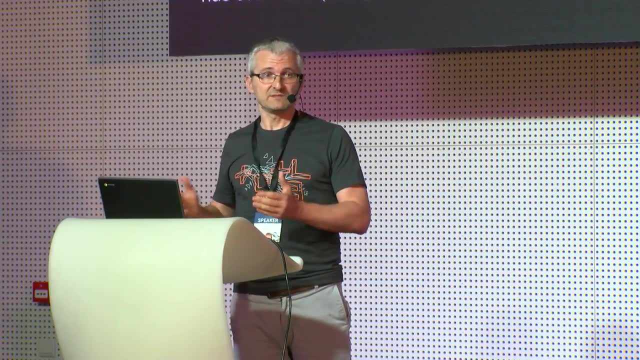 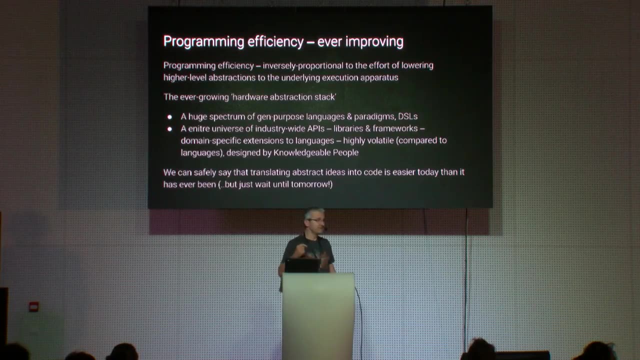 by highly knowledgeable people, experts in the field, I mean. that's the reason that such APIs and frameworks become industry-wide in the first place. So it wouldn't be again a stretch to say that programming efficiency has been on the rise ever since programming became a thing, and today it's easier to translate abstract. 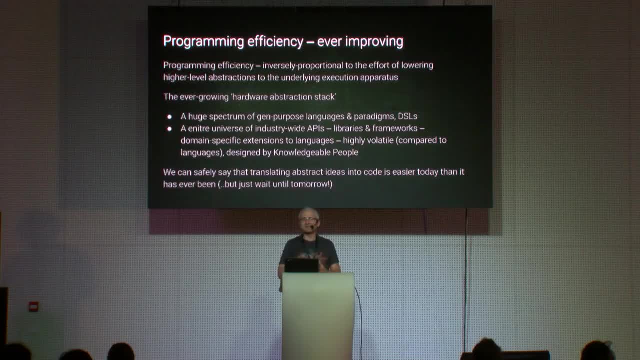 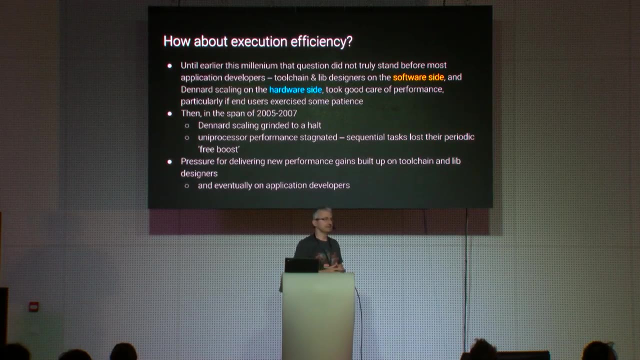 ideas into running code on a piece of silicon than it has ever been in human history. Moreover, we can expect that tomorrow, this will improve even further. Well, how about execution efficiency of the hardware? Is perhaps the situation likewise? Not really So. until earlier this millennium, there were two forces that were really pushing performance. 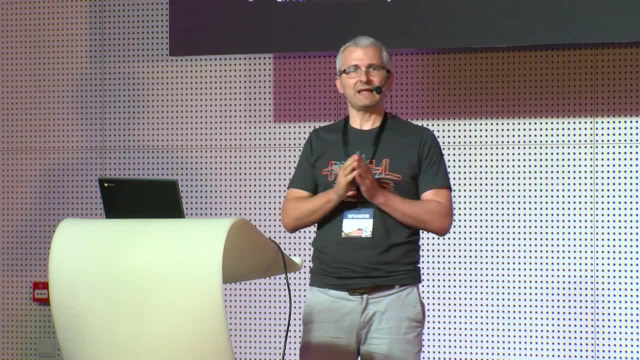 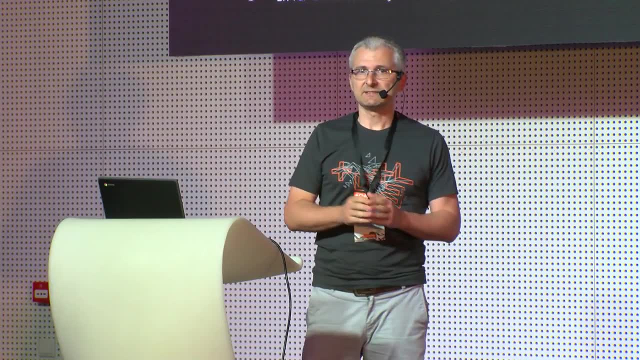 forward Again on the software side. we had the effort of all the software developers working on language toolchains, And by toolchains I don't mean just compilers and linkers. I mean compilers, linkers, debuggers, static and dynamic analyzers, profilers. 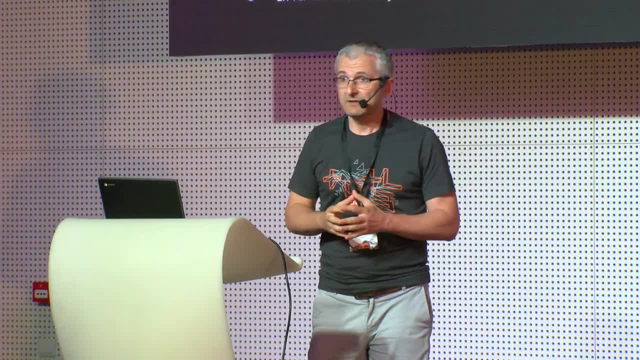 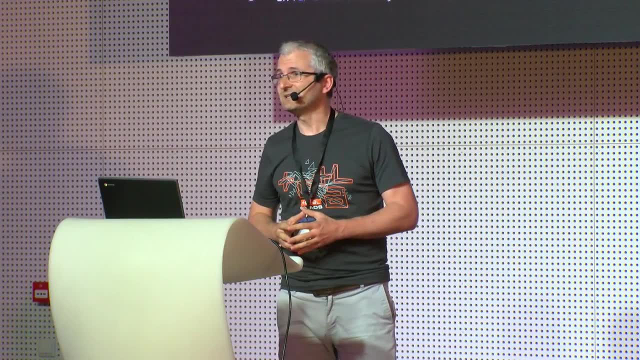 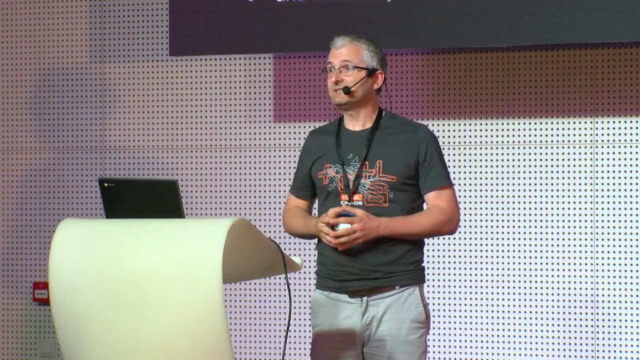 So all that helps us as programmers to extract optimal performance after our code. So that's the first thing. So that was on the software side. On the hardware side, there was something that was known as Dennard scaling. Dennard scaling was an empirical law devised in the middle of the 70s. that, basically, I 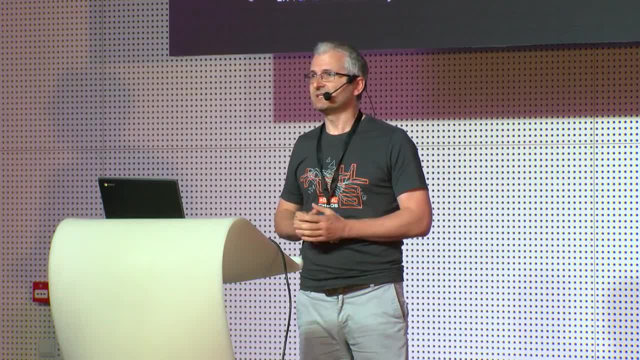 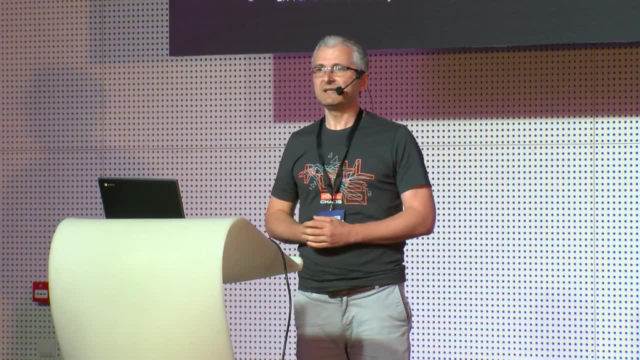 will not delve into details about Dennard scaling. I would just mention that what came out of it as a final benefit to the end user and to developers was that Dennard scaling promised that electronic transistors, as used in computers, would be able to run on the same network. 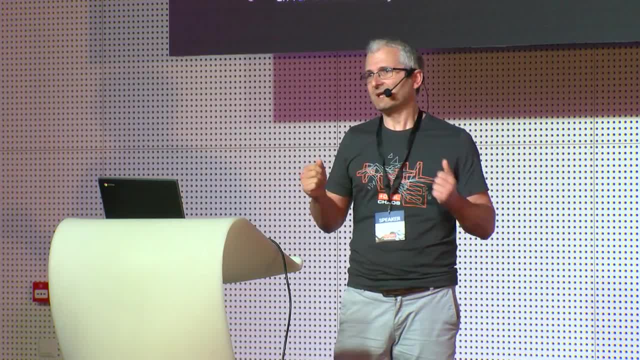 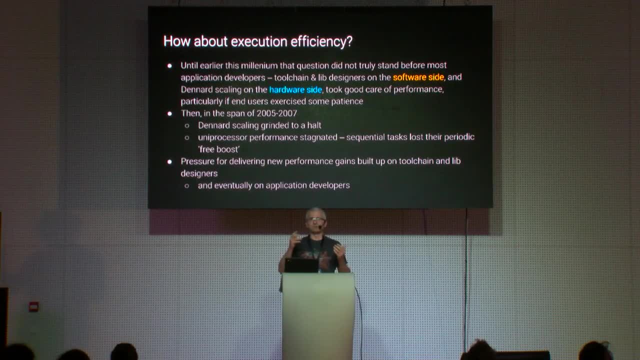 That is roughly double their electrical performance characteristics every roughly two years. So every two years we would have twice better electrical efficiency transistors And that actually translated to the end user in exponential rise of clocks, of CPU clocks. Now that was very fine and dandy until one day. well, one day, figuratively somewhere. 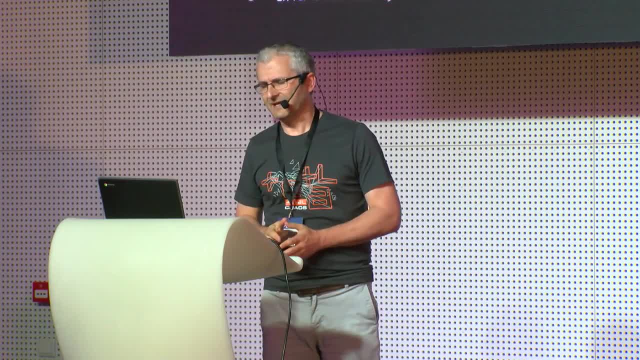 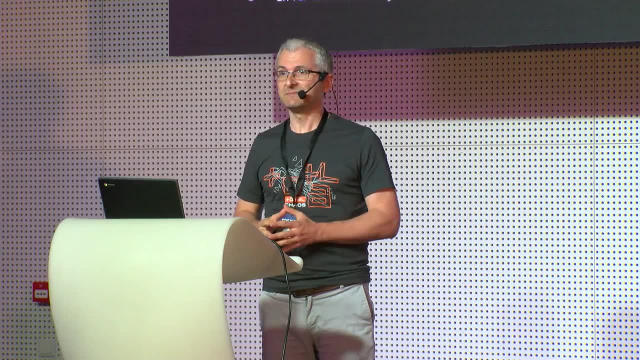 in 2005, through the span of 2007.. Or 2009,. perhaps Dennard scaling grinded to a halt. There was no Dennard scaling at play anymore. Something had happened in lithography processes, in fabrication processes of chips, so Dennard scaling stopped working. So what happens? when two forces are working together to pull a big boulder of weight and one of the forces dies off, the other force gets all the weight to pull. So all the pressure for delivering further adoption Advancements in performance fell on language developers and tool chain developers and API. 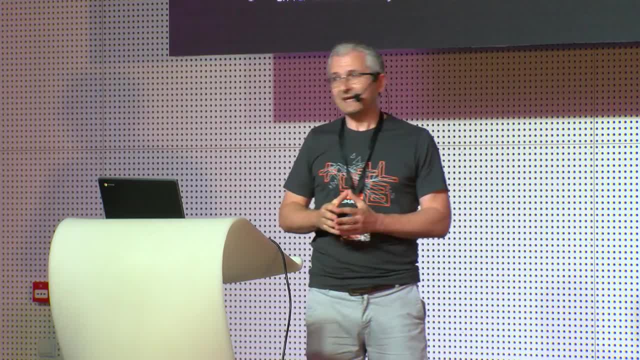 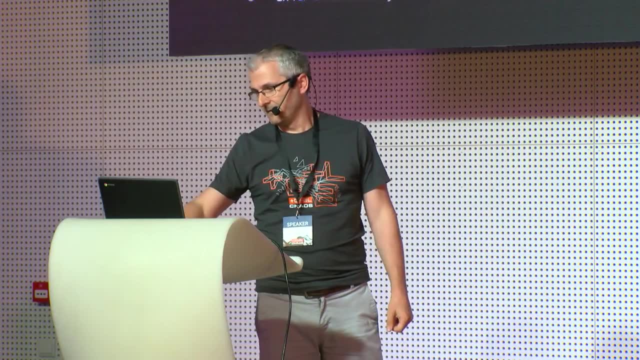 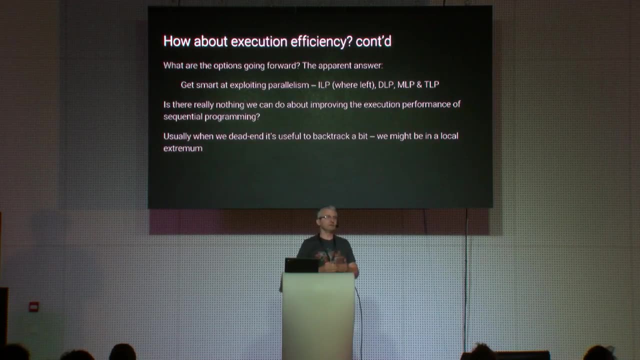 developers. Of course, that situation could not last for indefinitely long, and that pressure translated on application developers eventually. So what were, back then, the options, and what are still the options of going forward? Well, the very apparent answer to this question is: get smart at using parallelism. 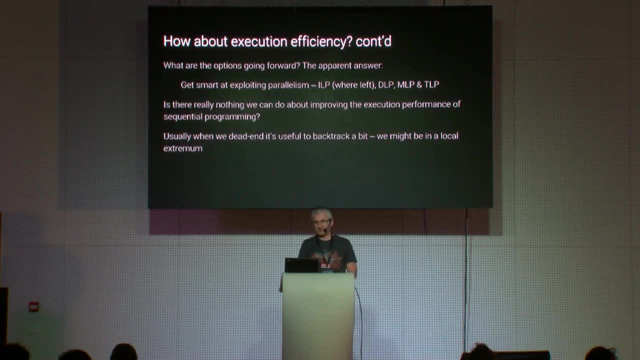 Luckily, there are various levels of parallelism. Listen of parallelism, starting with instruction-level parallelism, if there is such available for us, data-level parallelism, memory-level parallelism, as well as task-level parallelism. Now, today, I will not be talking about those kinds of parallelism. I will be talking mainly 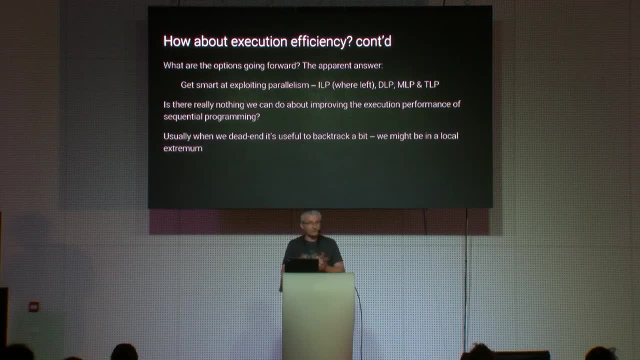 about something else. So is there really nothing else that we could do about improving sequential programming? Are we at the dead end? Is it the end of the road? Usually, when somebody gets to a dead end, the normal behavior in such a situation is to backtrack, backtrack. 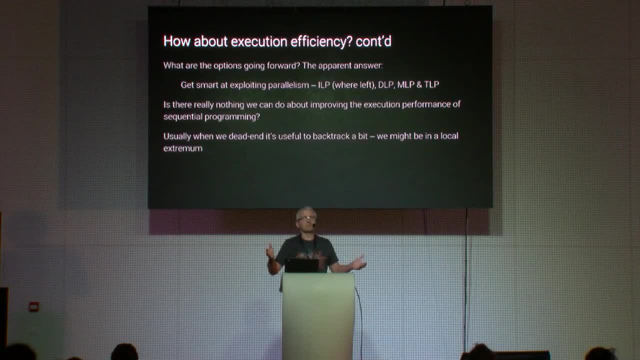 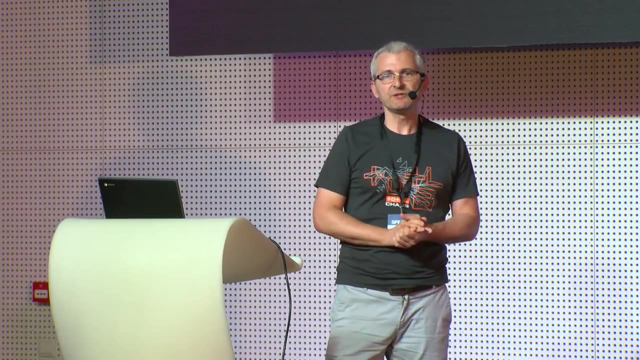 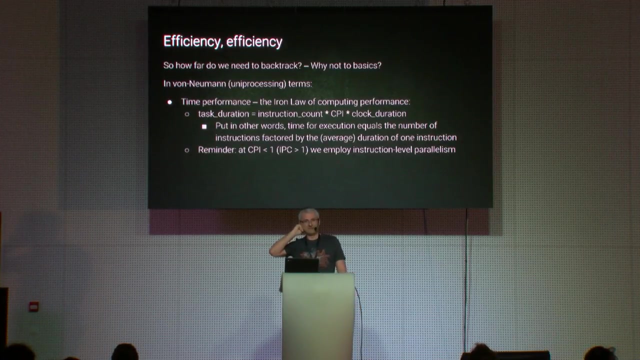 a bit and see whether they didn't get into some local extremum of their search function. So when we backtrack we usually go to a last known good position and in the case of CPU architectures that could be pretty much the start of our journey. And at the 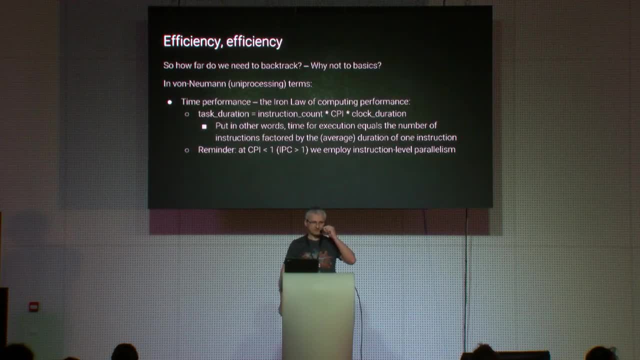 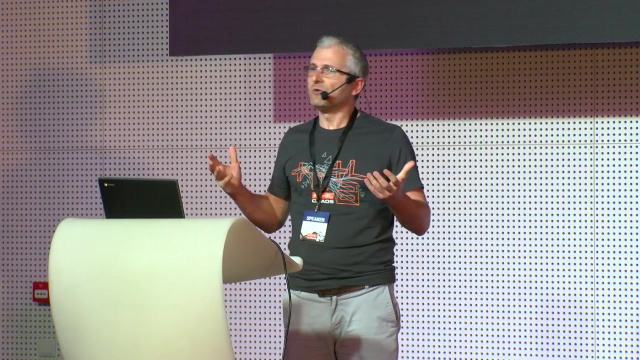 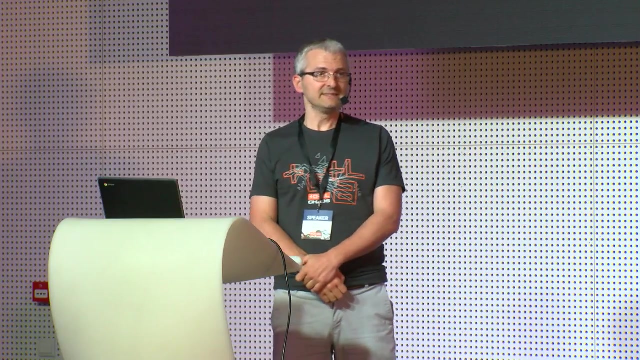 start of our journey. in CPU architectures there is something Sorry. There is something which is generally referred to or known as the fundamental law of performance of sequential computing. This is the iron law of computing. It's called iron law for a very good reason: It's absolutely imperative. The iron law basically states that the task 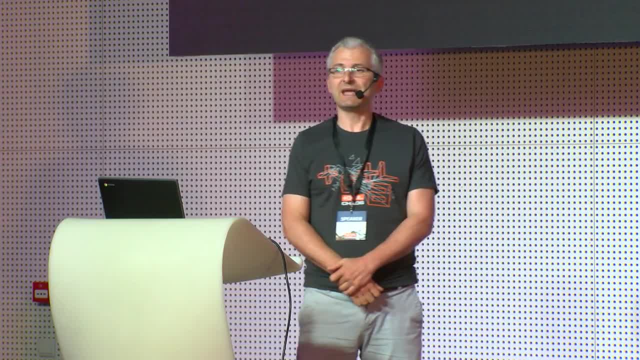 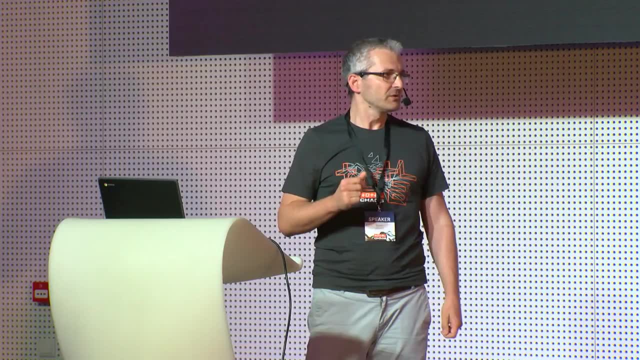 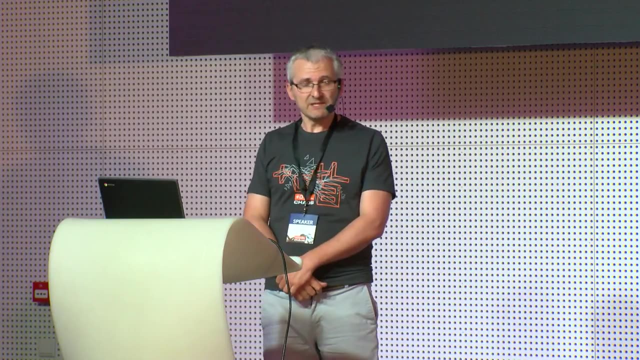 duration equals the instruction count, the active instruction count that the task takes to execute. The instruction count is multiplied by the clocks per instruction multiplied by the individual clock duration. Or put in plain English, that means that the time our task takes to execute equals the dynamic instruction count multiplied by the average duration of each. 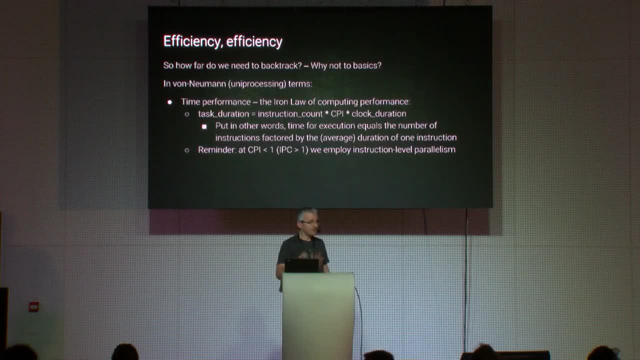 individual instruction. Now here we should put a remark that at clocks per instruction less than one, or its reciprocal instructions per clock greater than one, we are already taking advantage of a certain level of parallelism, which is known as the instruction level parallelism. 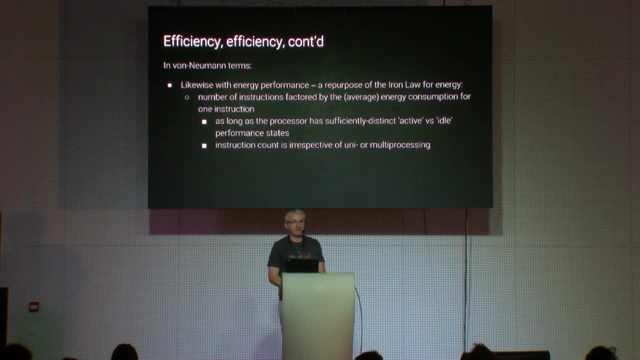 Again, we could actually repurpose the iron law of performance for energy performance just as well. We could just as well say that the energy performance of a given task executive on a given apparatus equals the number of dynamic instructions multiplied by the average energy consumption of our instruction for that architecture. Now, that is true only when. such a processor has distributed some monumental parts. Again, I don't go in deep talk about how much pulse is built into the structure or dialogue, right, The structure comes out into things. But we can at least be clear afraid and open our minds about the times they are. 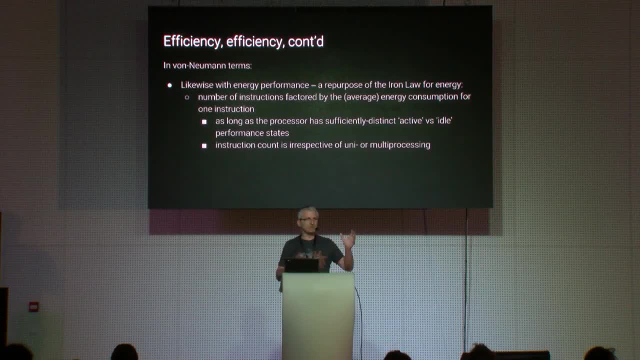 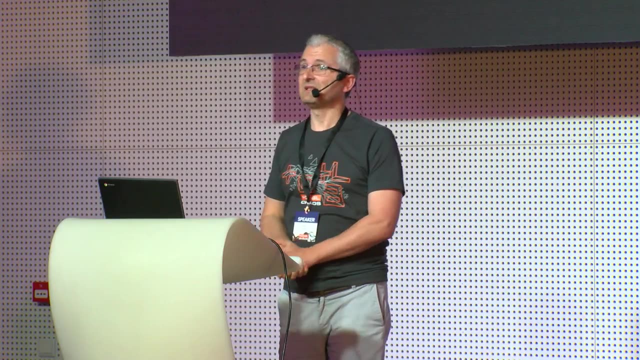 used to, And we can, wouldn't be so wise. but unfortunately, every time we set them up for something distinctively different states between active, actively executing instructions, and idling or passive state. Now, luckily for us, all processors have been lately moving in that direction. They all have power states, power levels where the CPU 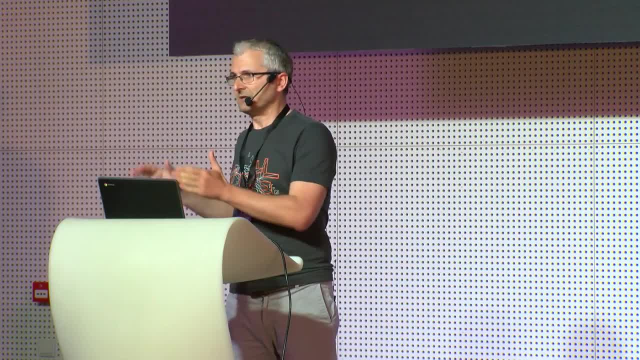 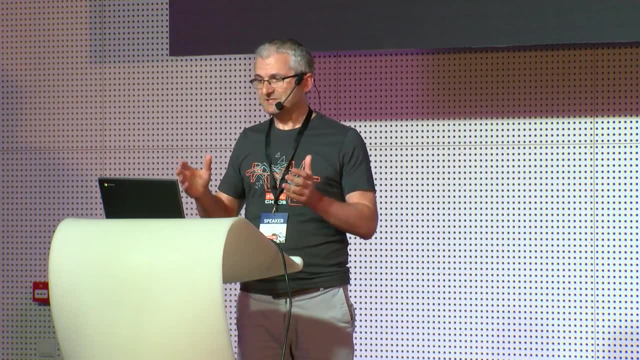 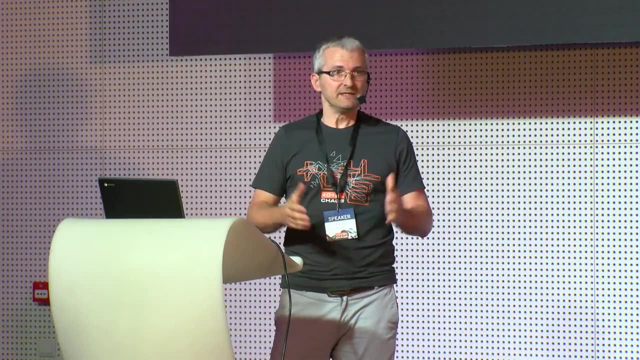 would consume one amount of energy executing instructions and then consume much less energy when idling. And here another remark is that this repurposing of the Ion law of performance is actually true regardless where we do uniprocessing or multiprocessing, Because instructions just accumulate. we. 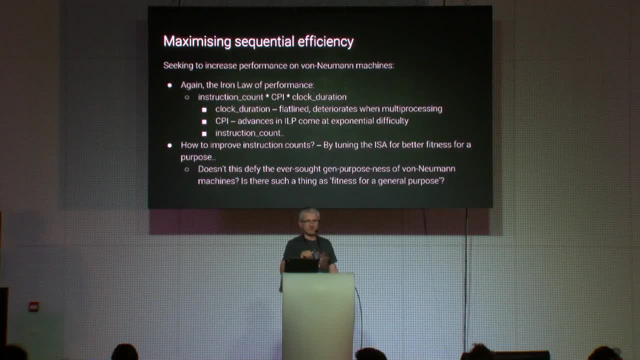 don't care where they arrive from. So seeking to improve the performance of von Neumann machines, again focusing on the Ion law of performance, term by term, Let's see what the options are before us. Well, we said that the clock duration, it didn't exactly flatline. I've put a very strong word here. it didn't exactly. 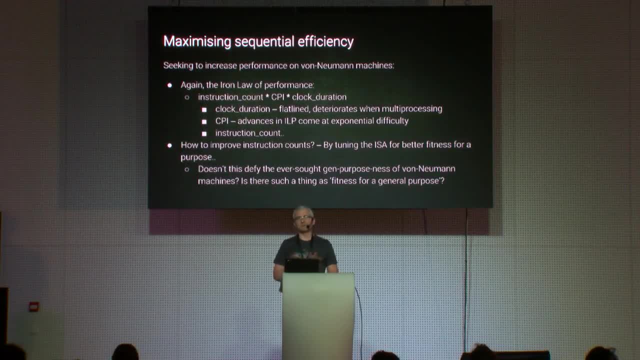 flatline, but it exponential growth- died Somewhere back in 2005.. The worst news is, though, that when we do multiprocessing, our instruction clock drops. Why? Because it takes more energy to run end processors at the same clock than it takes to run one processor at the 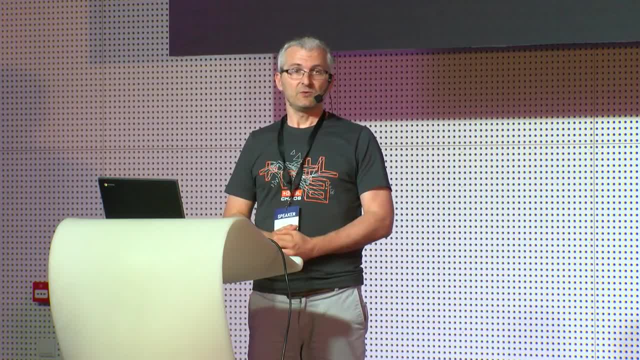 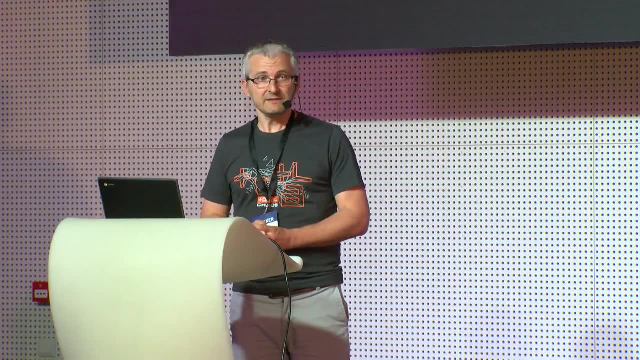 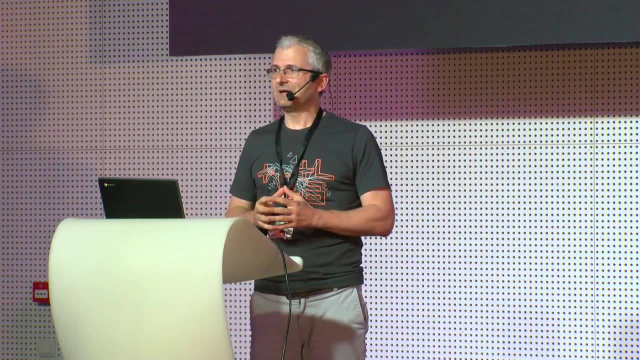 same clock and that energy has to be dissipated, etc. So when we do multiprocessing we inevitably get a drop in clock compared to uniprocessing. So what is a multiprocessing? Well, it's a function of instruction level parallelism. Now, advancements in instruction level parallelism usually come at exponential. 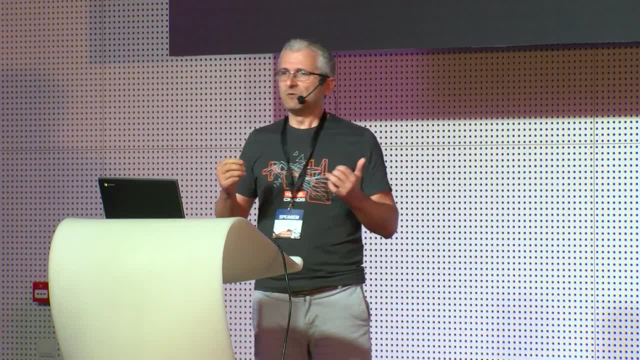 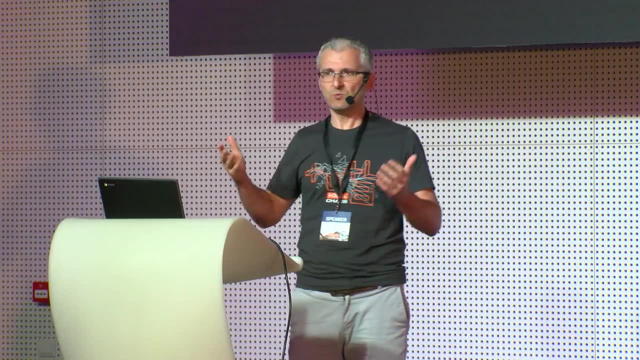 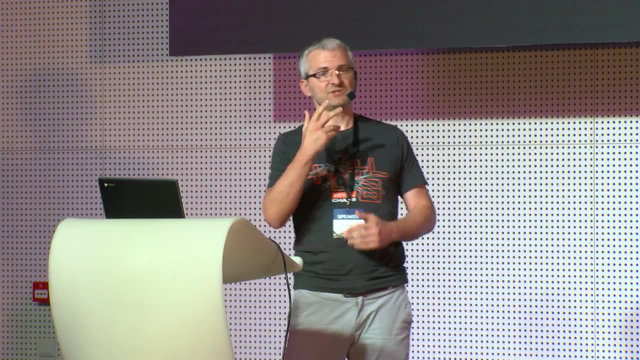 difficulties. What does that mean? That means that we know pretty well how to turn a one instruction per clock processor into two instructions per clock processor. It's a well-known fact. Now it's slightly more difficult to get the two instruction processor into a two instructions per clock processor, and it's much, much more. 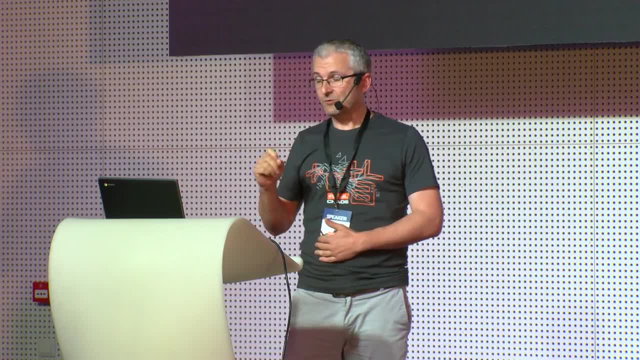 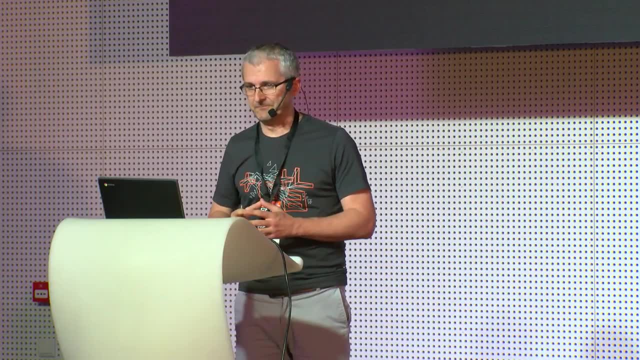 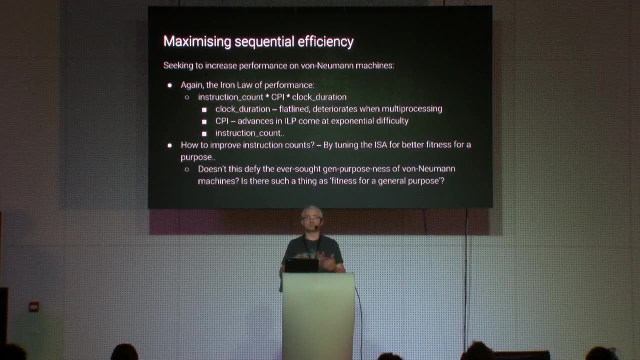 difficult to go beyond that, So that increases in that term of the law come at exponential difficulty. And the last thing that remains here in the instruction count: Is there a way that we could improve instruction counts in our code? Well, here we could say that we could improve instruction counts by: 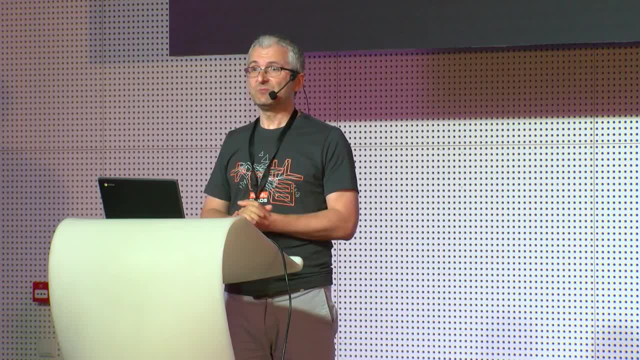 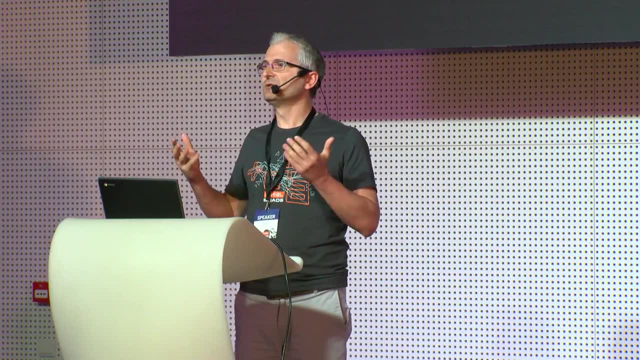 making the ISAs, the instruction set, architectures to be better fit for our purposes. What does that better fit for? This is basically another way to say that they're useful. Now, when we say that something is useful, though, we could say that a stone is useful for breaking. 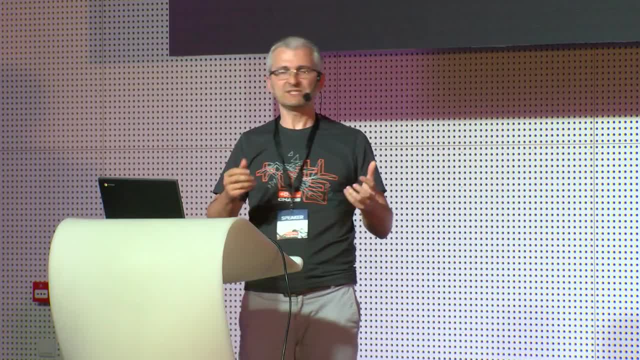 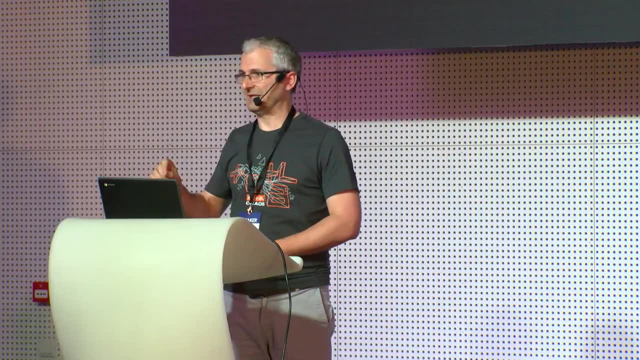 stuff, But it wasn't designed for that way, right? We just accidentally found the use for it. When we say that something is fit for purpose, we actually imply that somebody deliberately made it useful for that. And the difference between a stone that we used to break stuff with and a hammer that was designed to break stuff. 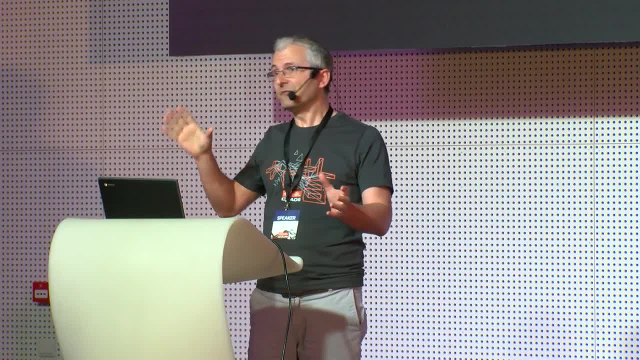 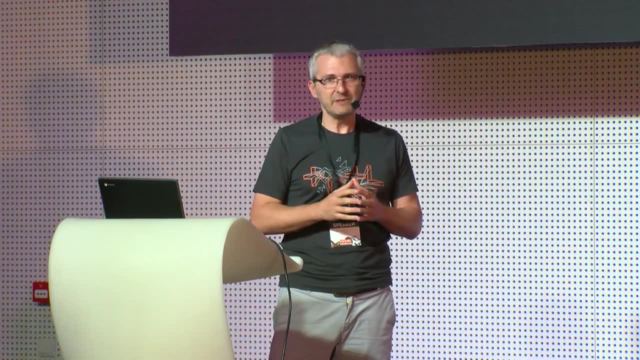 with is we could say that one is useful and the other is fit for the purpose. So can we make our instruction set architectures fit for general programming purpose? Now, that's a bit of a cliffhanger here, because what does fit for general purpose programming mean? I mean general purpose programming, the 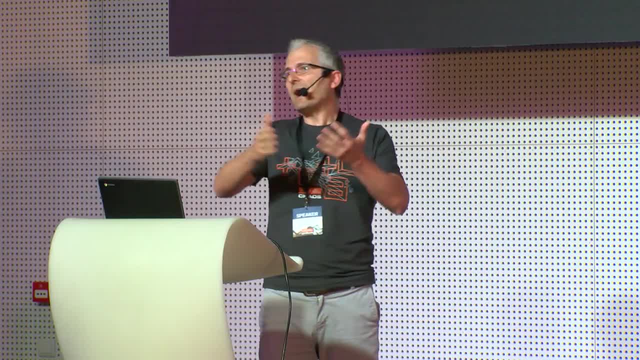 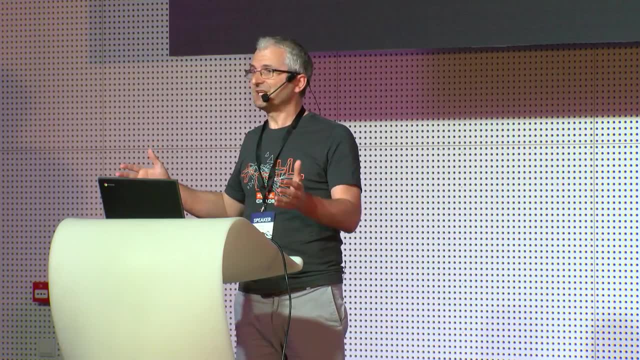 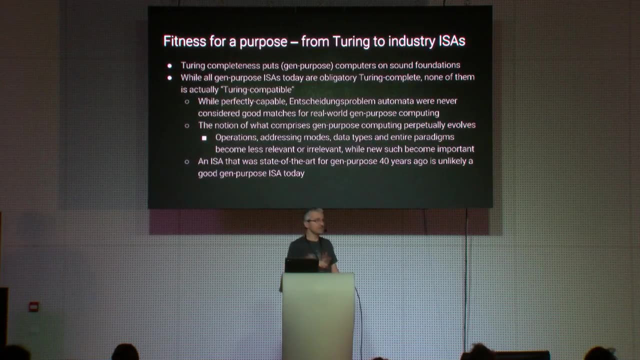 very idea of general purpose programming is that it's a wide range of applications. So how do we actually make something specialized for a wide range of applications? Isn't that an oxymoron in the first place? Well, let's see. Let's start with Turing completeness. Well, Turing completeness is something that 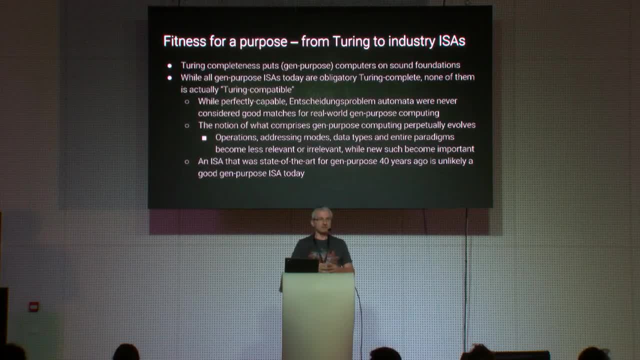 gives us a very, very good fundamental for us to start and develop instruction set architectures. It guarantees certain mathematical properties of our computers. Now we can say that while every general purpose ISA today has been Turing, designed, deliberately designed to Turing complete, none of them is really Turing compatible. And by Turing compatible I. 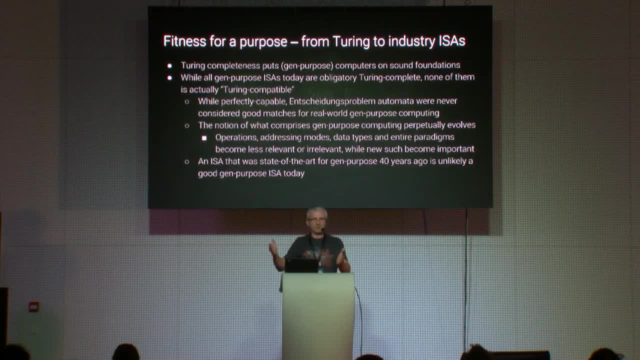 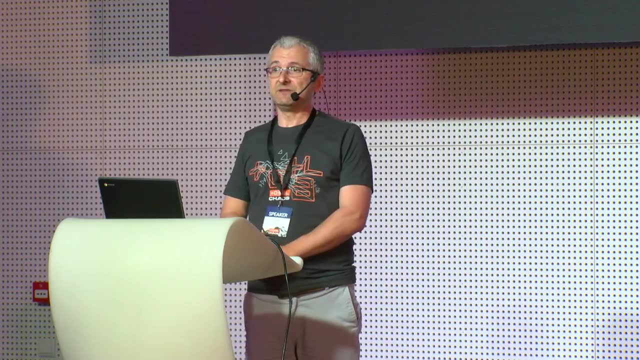 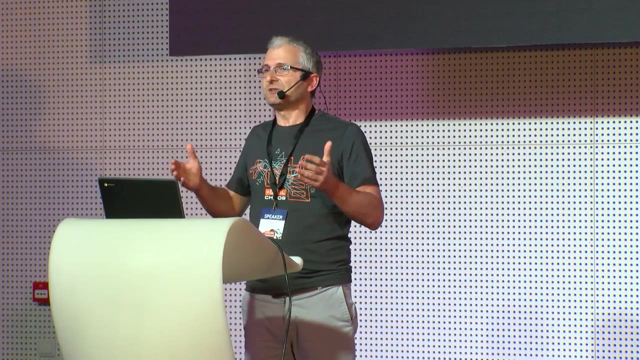 mean that they don't really try to process code the way Turing machines were designed. Why? Because Turing machines were just a mathematical abstraction. The Scheidungs problem automata devised by Alan Turing were made to prove certain properties of a mathematical problem and nobody really meant to run code on them. 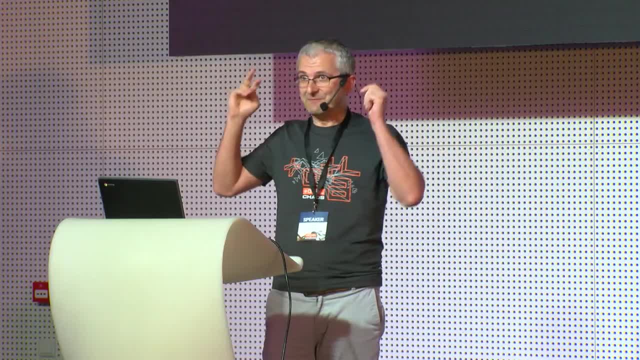 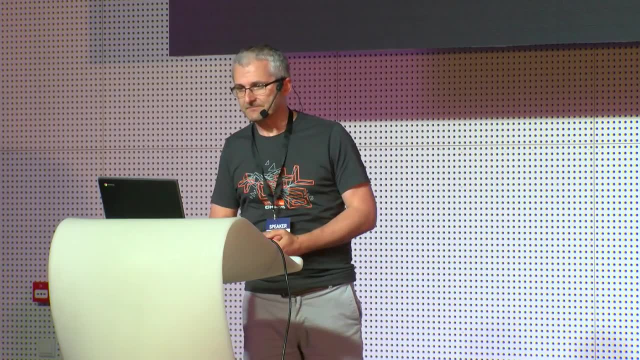 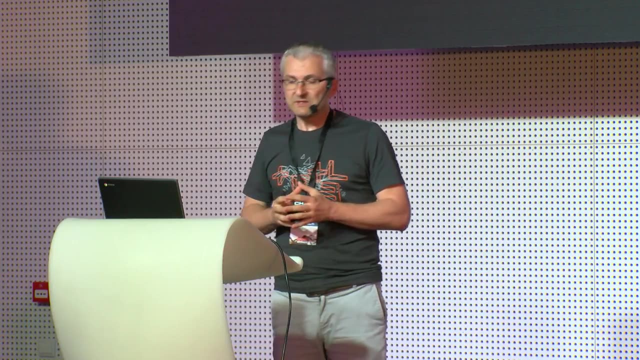 back then. Ergo, none of the current architectures are Turing compatible. It makes no sense, Even though Turing architectures are self-sufficient, to be general purpose machines. Actually, the very notion of what comprises general purpose computing evolves with time And, as a result, operations addressing modes, data types and entire. 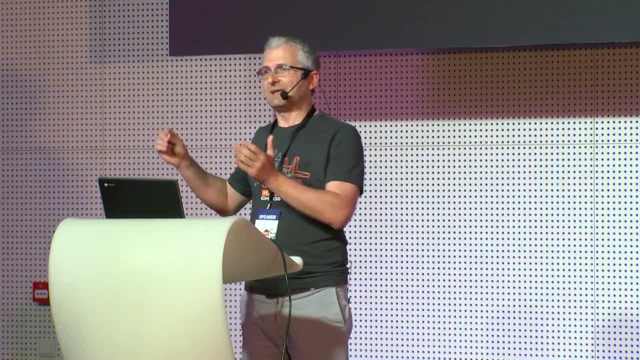 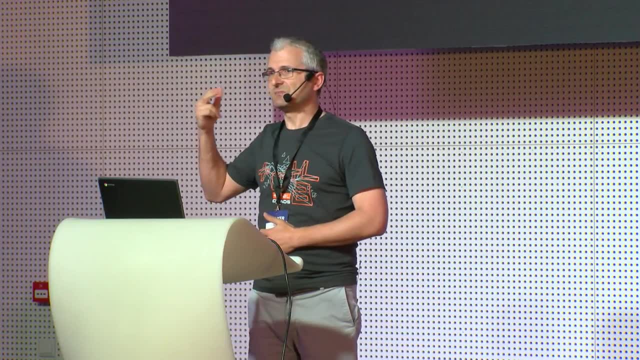 paradigms become less relevant with time, and other such instructions addressing modes and data types become more relevant as we move on forward, because our understanding of general purpose computing evolves As a result. an ISA that was a state-of-the-art for general purpose computing some 40 years ago is a. 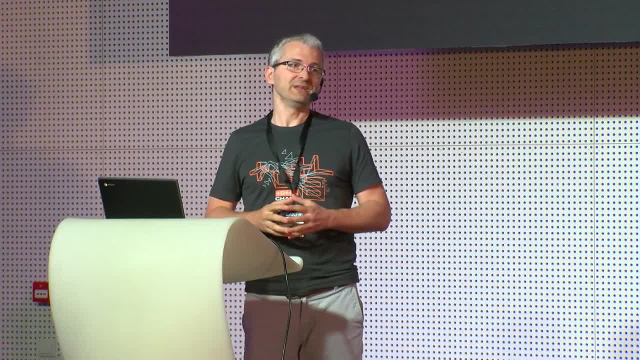 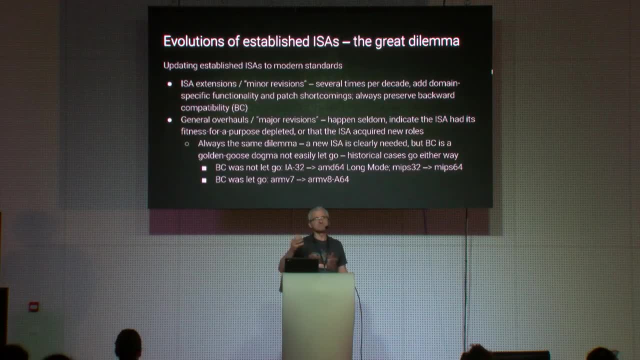 very unlikely candidate to be a state-of-the-art general purpose computing ISA today. So what happens to ISAs? What comprises the lifespan of an ISA? Well, usually ISAs. here I'll make a difference between two major ways of ISA evolution. One of 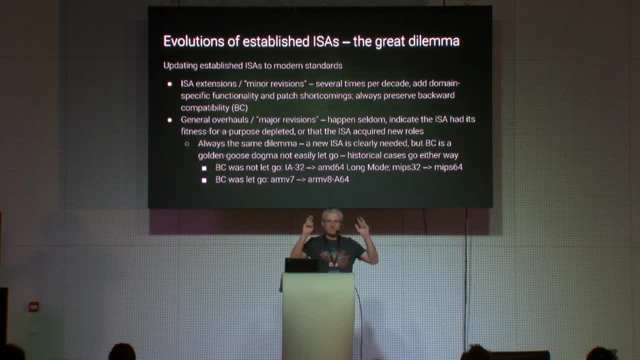 them I'll call minor revisions and the other I would call major revisions. Minor revisions usually happen several times per decade for most active ISAs and they usually add domain specific functionality to an ISA. Sometimes they fix shortcomings, but mandatorily such minor revisions always keep backward compatibility in the ISA. 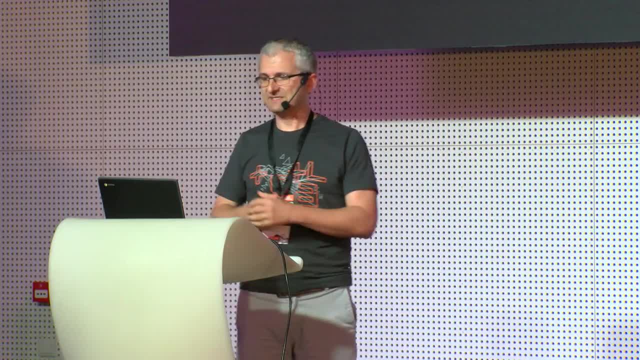 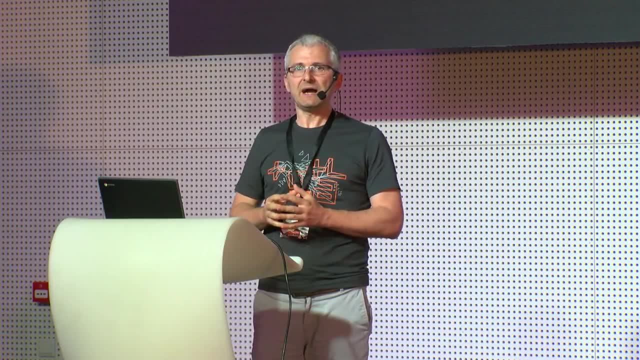 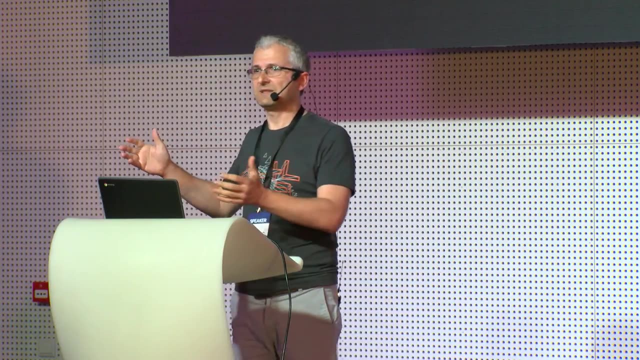 Now, the other kind of evolution of established ISAs is when major overhauls happen to an ISA. That means that the ISA either was running out of usefulness at that stage in time or a new role was acquired for that ISA. Somebody started using that ISA for something else that it wasn't originally used for And at 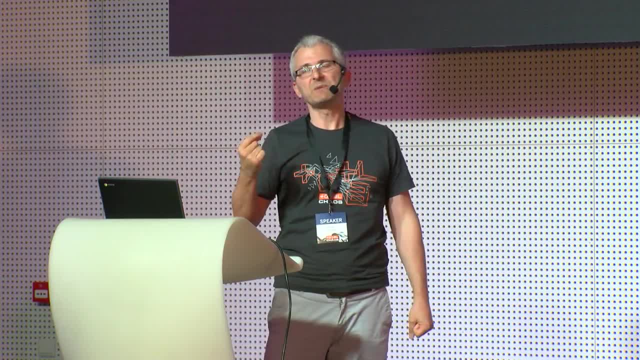 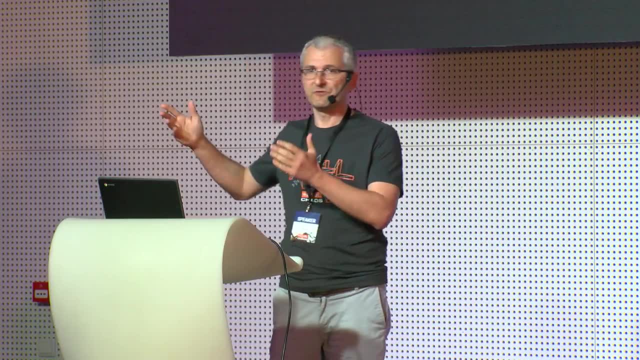 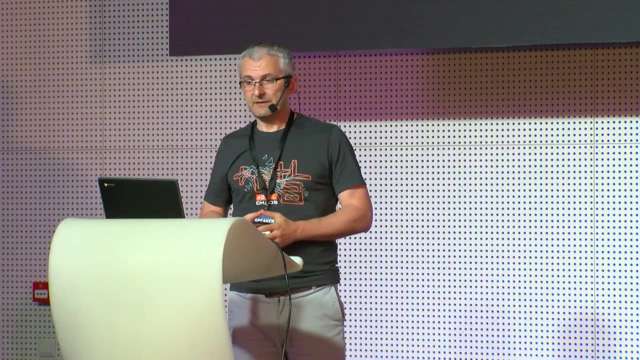 such a major revision. always the following dilemma appears before ISA architects: Shall we keep backward compatibility or shall we drop it and try to produce the best possible ISA going forward? Actually, in history we have examples of decision in going either ways. Two examples: Situations when a 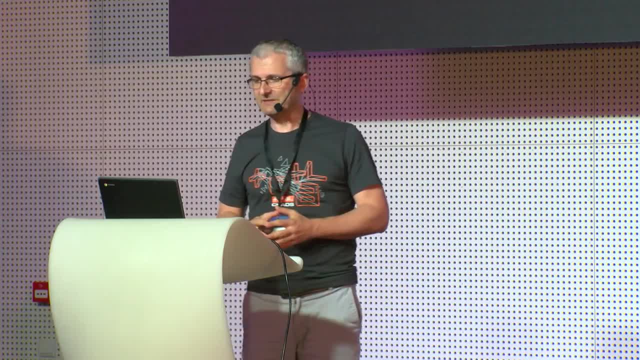 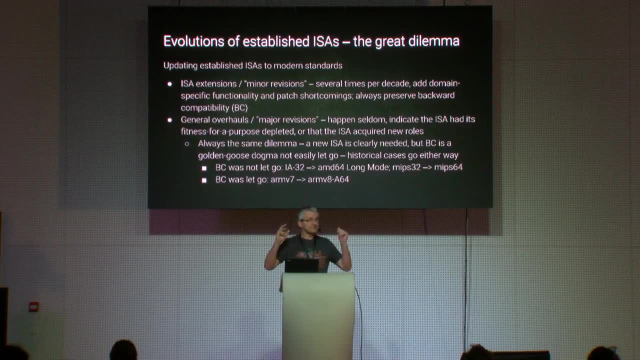 major revision of an ISA. actually effectively preserved backward compatibility is the transition of Intel's instruction architecture, Intel architecture 32, to the 64-bit version of this architecture. There the binary compatibility was largely preserved. Another such typical example in the world would be the transition from MIPS 32-bit to MIPS 64-bits, where the binary 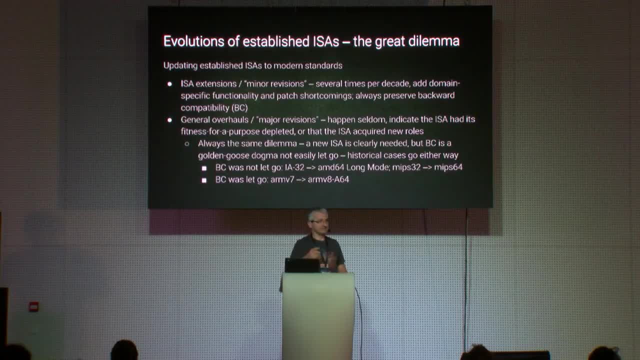 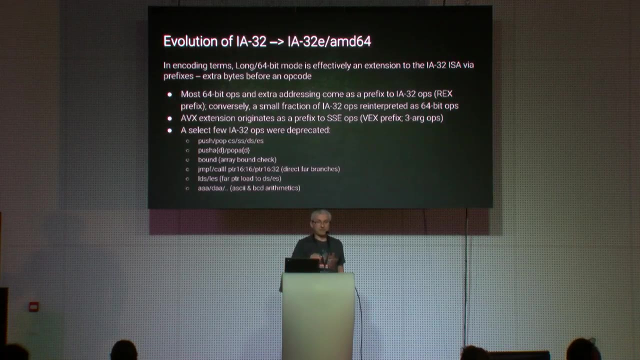 compatibility was also largely preserved. An example of the opposite, where backward compatibility was abolished, was completely dropped, is the transition from the last 32-bit ARM architecture to the first 64-bit ARM architecture. There is no backward compatibility. Now let's focus slightly on the transition of the Intel architecture 32. 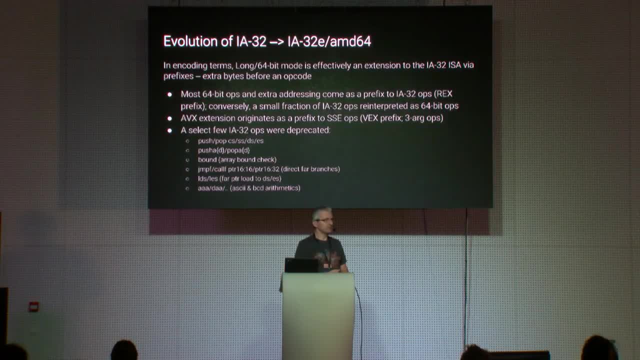 onto the 64-bit version of the Intel architecture. First, when we talk of 64-bit Intel architecture, we have to specify that it's a particular mode of execution in the processor and it's known usually as long mode or 64-bit mode in the documentation. Now that transition on an encoding level on 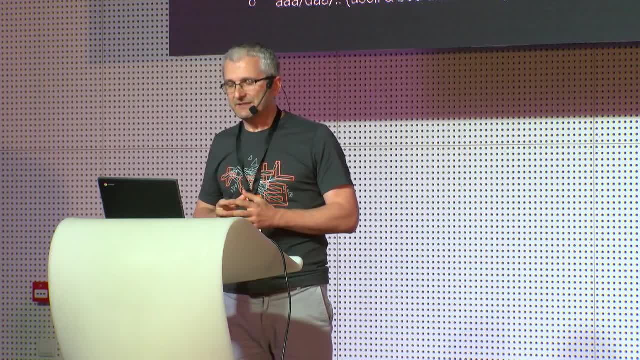 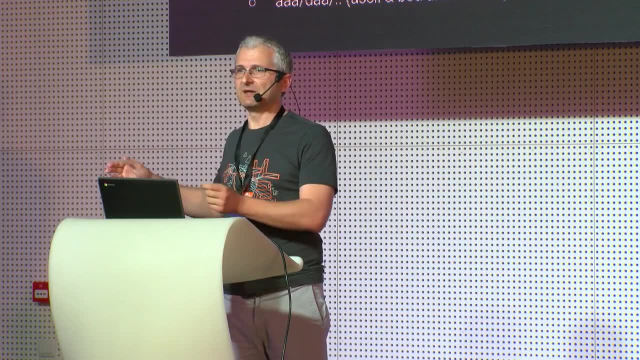 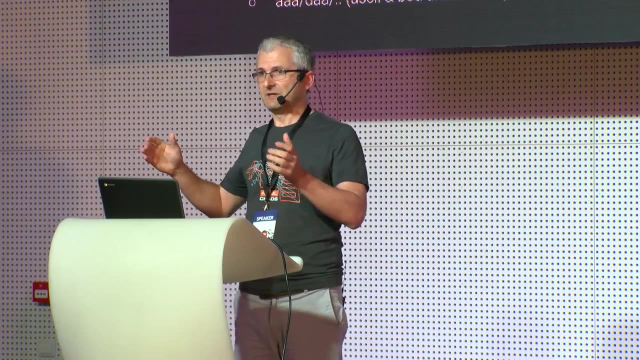 the way that the processor interprets instructions is achieved in a 64-bit Intel architecture as a, usually as an extension to already existing operations, and that extension usually comes in the form of prefixes to the operation. that means extra bytes before an operation encoding so that effectively. 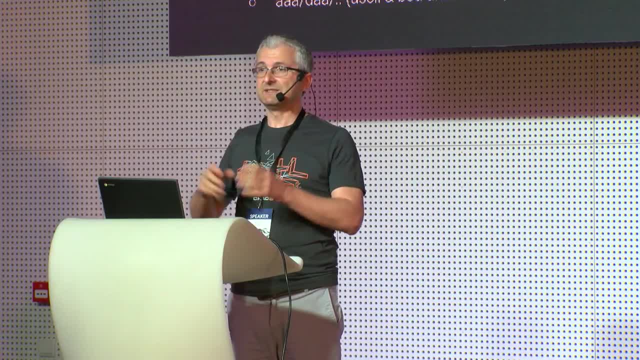 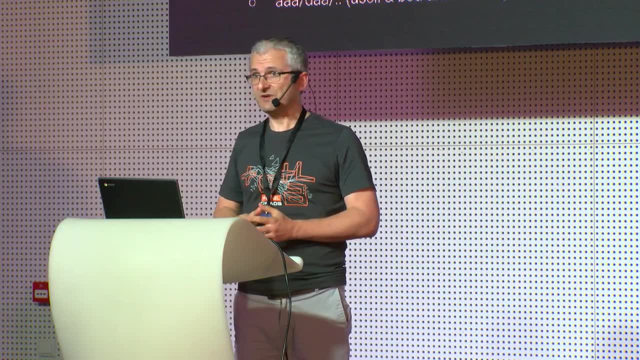 most 64-bit operations and extra addressing modes in the 64-bit Intel architecture actually come in the form of several major prefixes. the most well-known of them is the Rex prefix. that basically says this instruction: we are going to interpret it in a 64-bit architecture and that's the same as the. 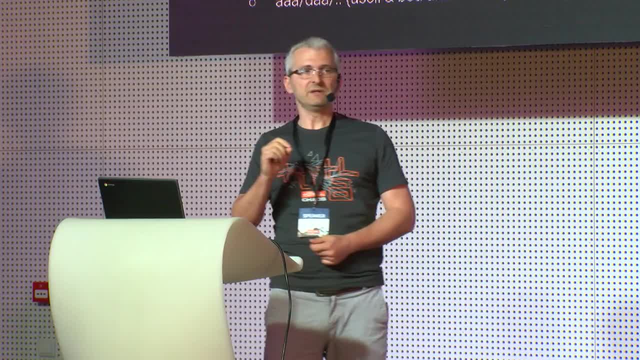 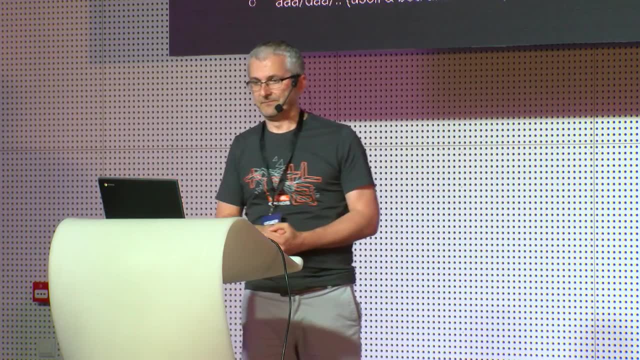 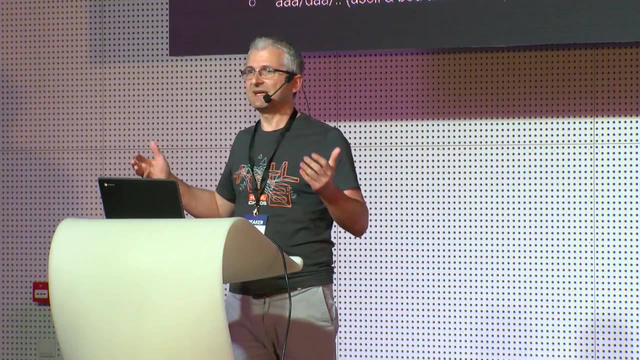 slightly differently Now. conversely, a very small number of instructions were actually reinterpreted in 64-bit mode, from working on 32-bit data to working on 64-bit data. The AVX instruction set also originates as a prefix extension to already existing SSE 4.2 instruction set. Now the interesting thing. 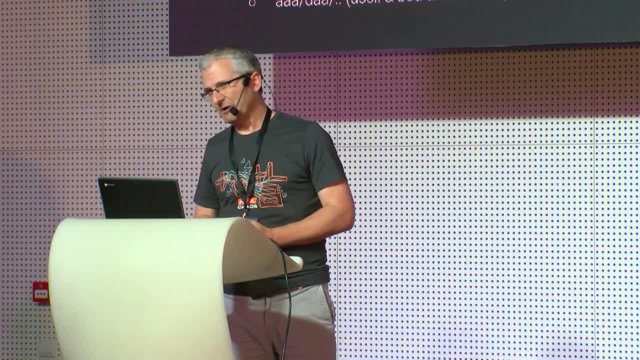 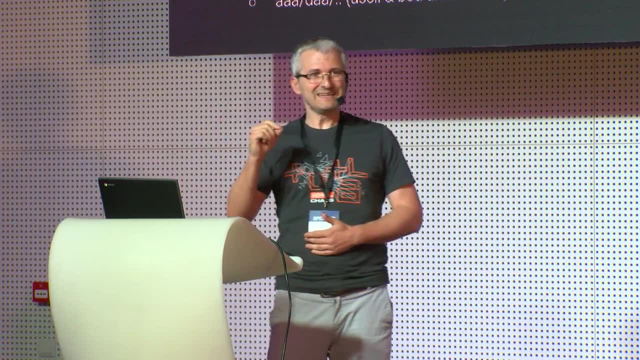 about the. this is the VEX instruction prefix. the interesting thing about the VEX instruction prefix is that it's a three-argument instruction prefix. We'll get to that in a second And finally, a very select few instructions were actually deprecated. That means they were removed from the instruction. 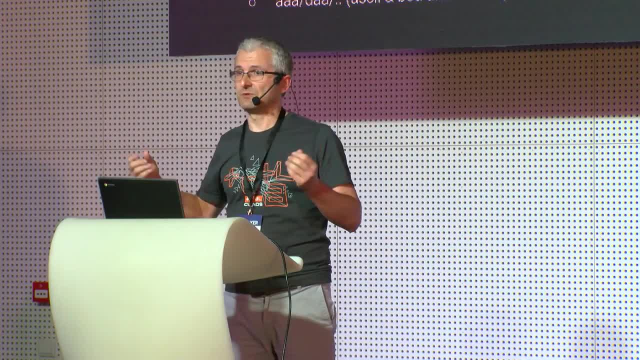 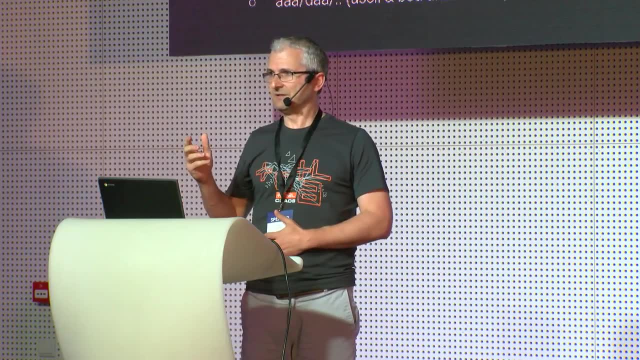 space and their opcodes were used for something more useful. Now, when I say very few, I mean literally six groups. six small groups of instructions were removed from the Intel instruction set, of which the most notable and the larger, the largest group of them is the ASCII. 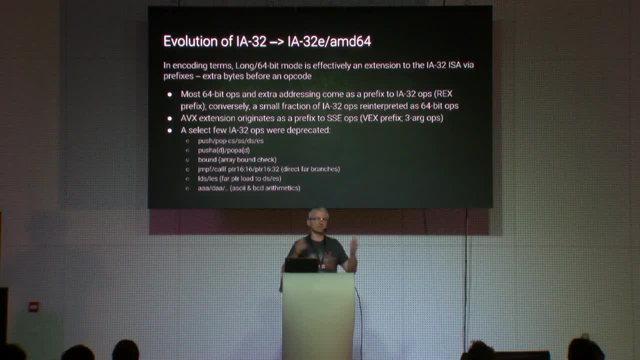 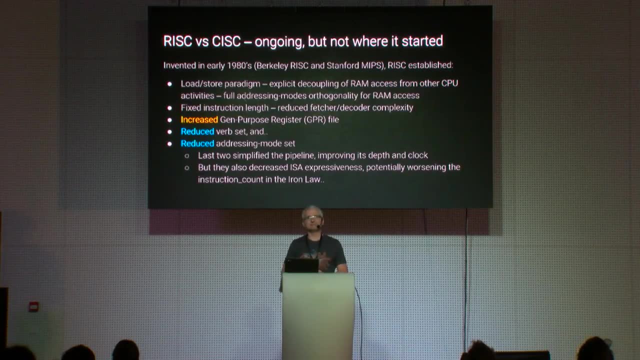 arithmetics and binary-coding decimal arithmetics. They were just abolished Now, somewhere in the middle of the 80s, something interesting happened in instruction set architectures. The dichotomy of RISC versus SISC appeared. Now RISC and SISC are two concepts that appeared with the introduction of that. 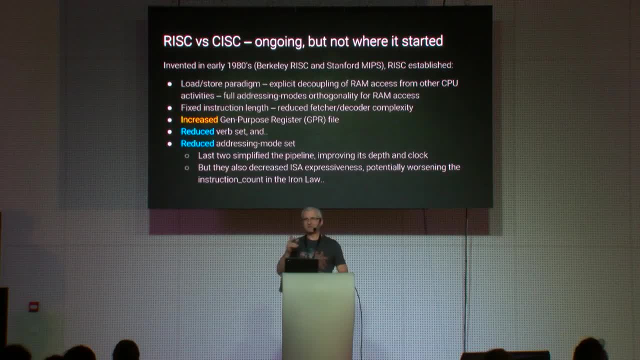 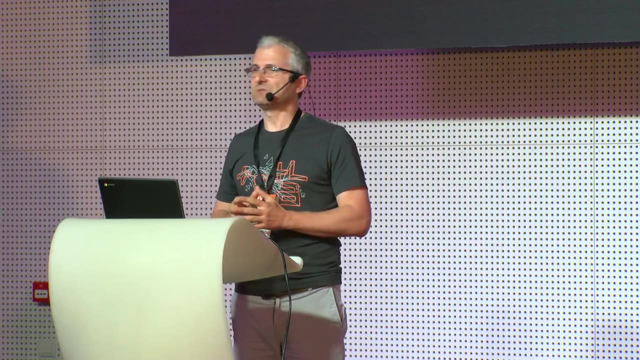 concept. and that concept actually appeared at the same time at two academic centers at Berkeley- both at Berkeley and at Stanford- And there people came to the conclusion that the five paradigms really changed the way ISAs operate. The first and most important paradigm was that: the access. 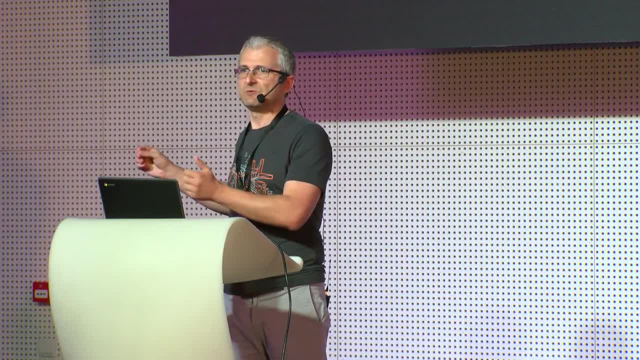 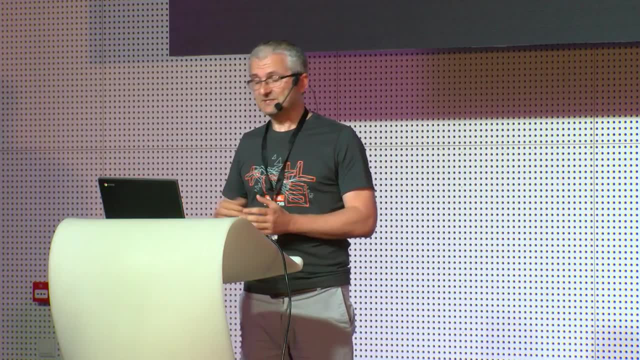 of CPUs to memory should be decoupled from all other possible CPU activities. This is called the load-stall paradigm and all the processors, especially all RISC processors, implement that paradigm. Whenever there is data to be accessed from memory, there would be deliberate instructions that the 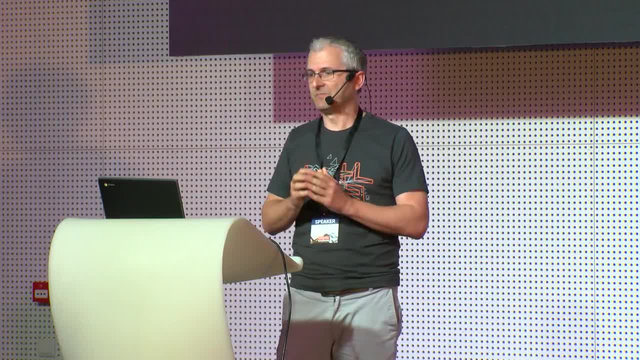 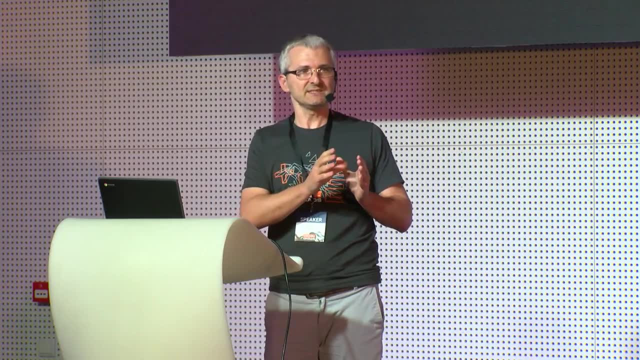 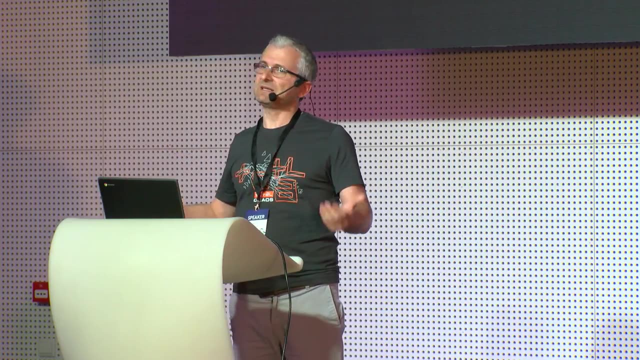 CPUs have to deal only with access to memory and nothing else. That brought to the following effect: Basically, since you have a small set of instructions that only access memory, whether they read or write regardless, all the other instructions don't really have to worry about access to memory. They have to have. 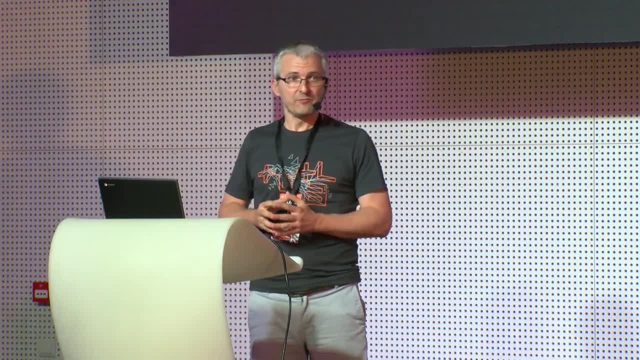 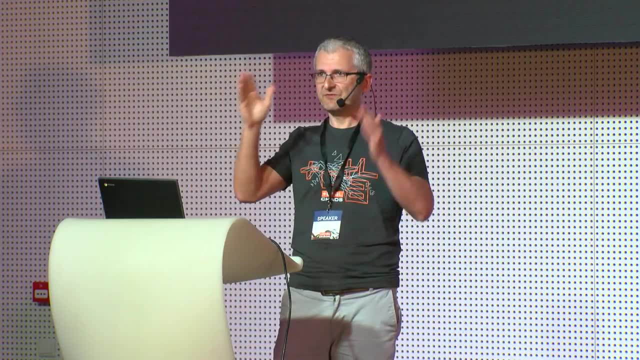 good access to registers. The second very important paradigm that was introduced by RISC back then was the fixed instruction length. That means all the encoding of instructions had to be a fixed length- Some good length for the decoder. That really reduced the complexity of the 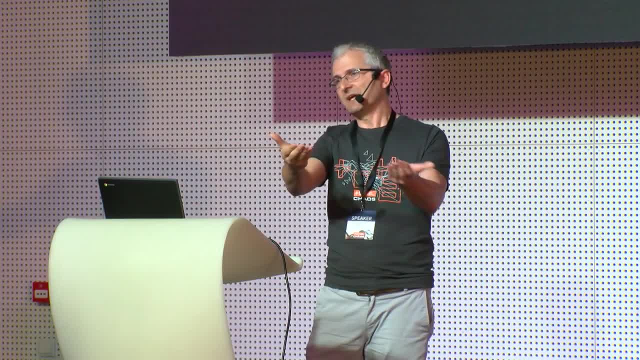 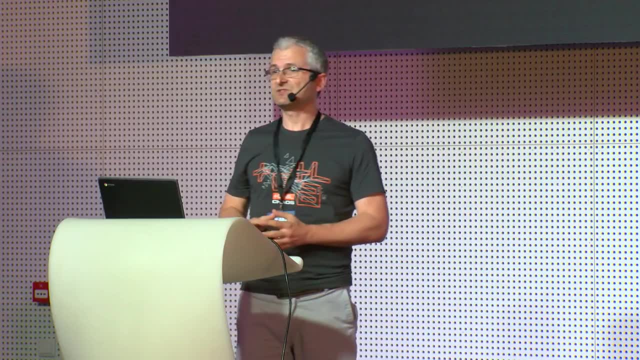 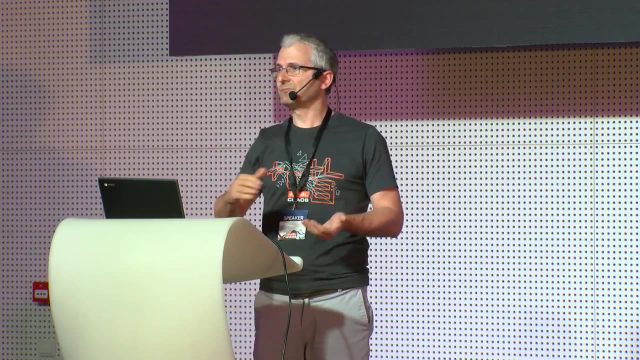 instruction decoder and fetcher, which are the gatekeepers to the instruction pipeline. The third paradigm was the large increase in the size of the general-purpose register file. The general-purpose register file is the in the programming model of an ISA. These are all the registers that the 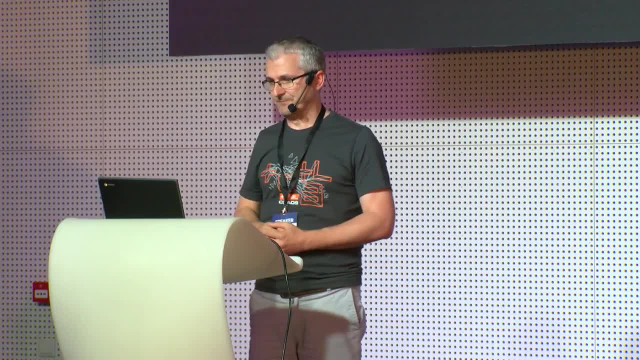 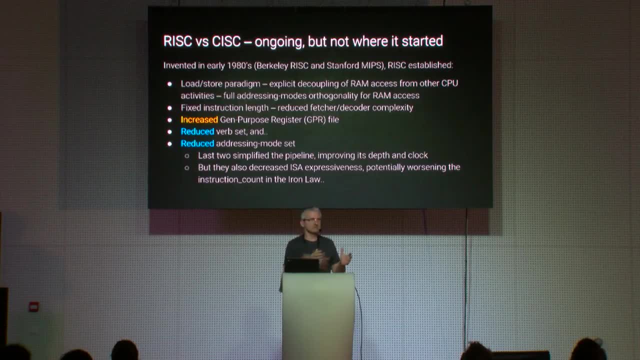 program or a compiler sees when they run on this CPU. And actually the last two paradigms were reductions. Some features of architectures were reduced. What was reduced? There was a reduction in the verb set, and by verb here I mean all arithmetic or logical operations. So RISCs, as an original idea, had fewer. 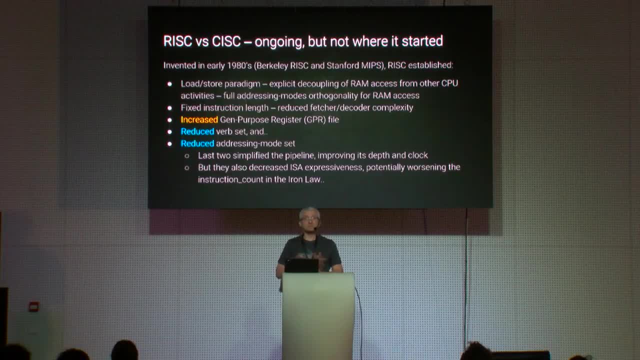 arithmetic operations, and also there was a major reduction in the addressing mode, So the way the processor would be able to access different addresses in memory. Now, the last two were made with the purpose to simplify the pipeline even further and improve its clock characteristics, and it served its purpose fine. Again, of course, that was a 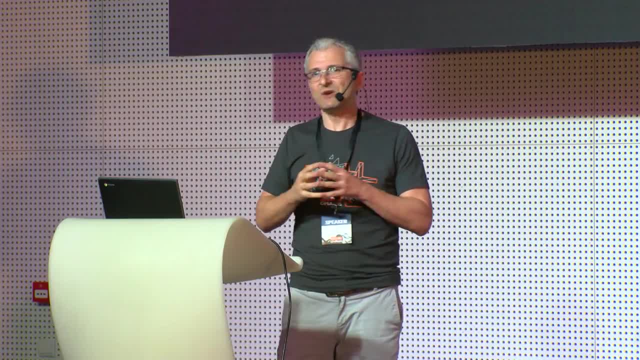 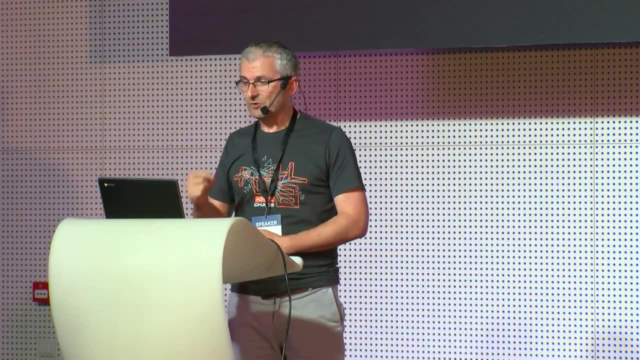 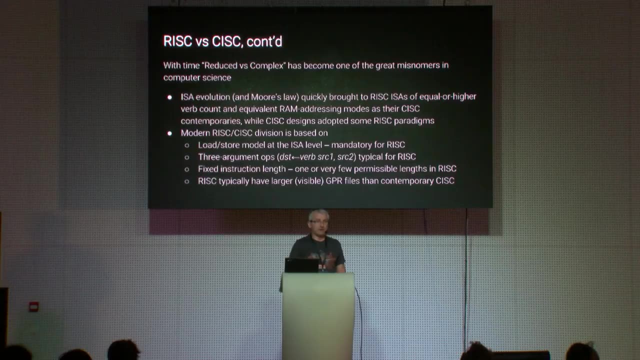 trade-off because there was also a decreased expressiveness of the ISA and from the point of view of the Ion law of computing that would impose a performance hit. Of course things were carefully calculated not to bring to this. So, with time reduced versus complex has. 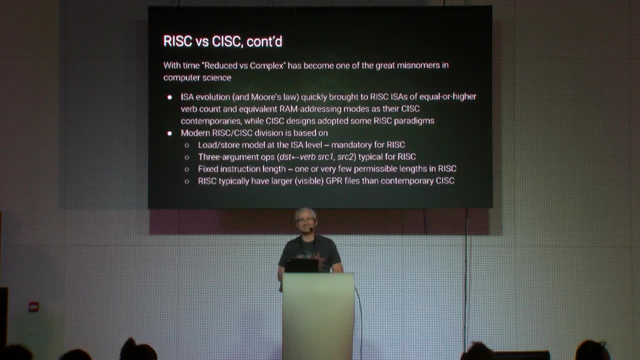 actually become one of the great misnomers in computer science. So when people say reduced versus complex, they usually mean those last two paradigms that reduced the expressiveness of the ISA. But is the case still like this today? No, the case has changed With the advancements in transistor. 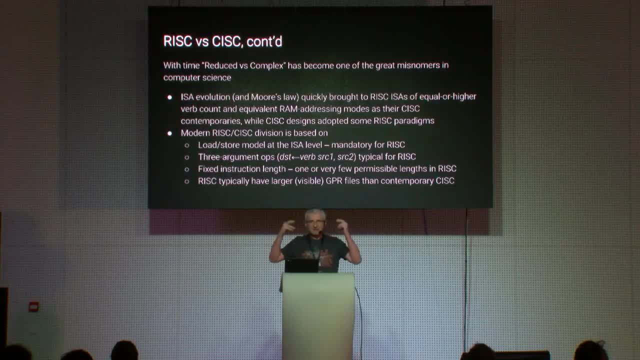 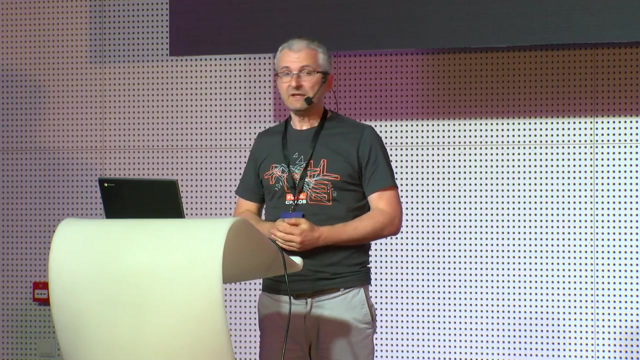 counts. RISC architectures have actually regained their lost expressiveness to a large degree. So today, RISC architectures have as many or even more verbs than contemporary RISC architectures, and they have also regained their addressing mode capabilities. On the other hand, CISC architectures have started adopting. 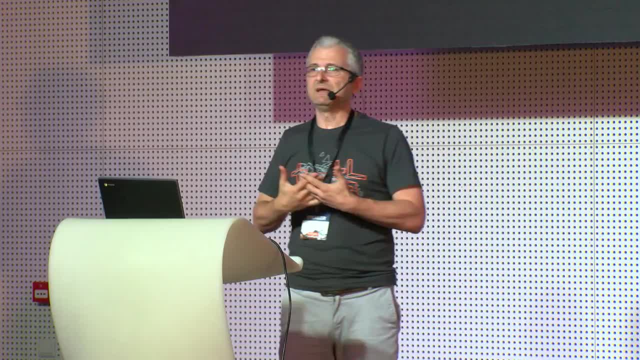 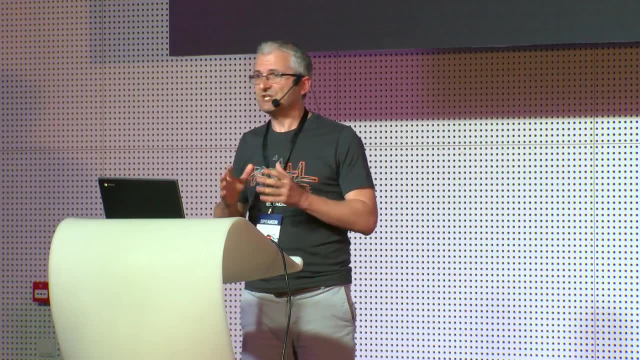 RISC paradigms. So there's been this intermixing of genes between the RISC and CISC paradigms Still in modern days. we can still make the differentiation between a RISC and a CISC architecture by the following four factors. First a: 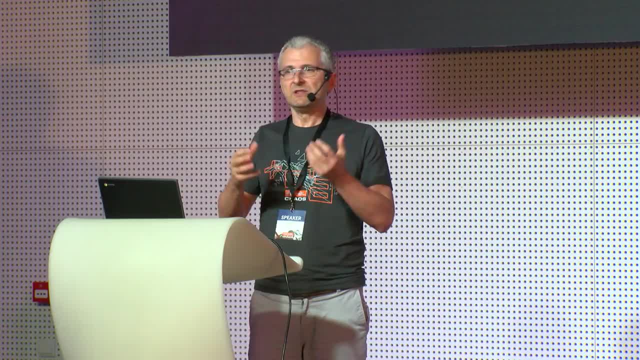 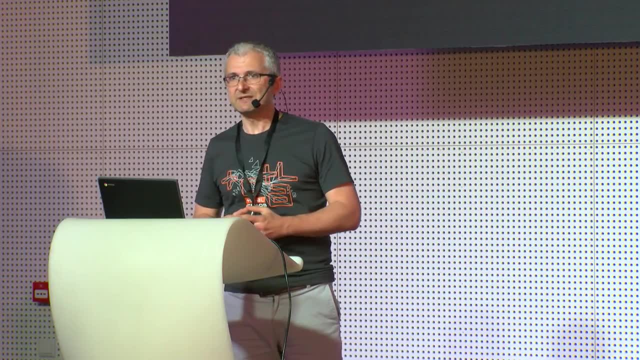 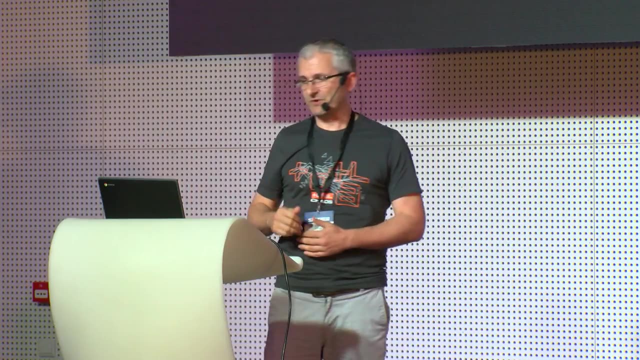 RISC is mandatory a load store architecture. There are no non-load store RISC architectures. Another thing that is very typical for RISC architectures is that they use the three operand encoding, So basically every operation has at least two input operands and one destination operand. That is very typical for 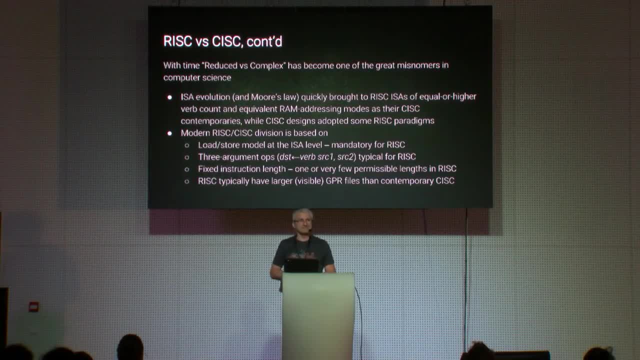 RISC. It's not mandatory but it's typical. Again, the fixed instruction length still remains as a requirement for RISC, but today it's been slightly loosened. So not just one instruction length encoding, but several few instruction lengths encoding. 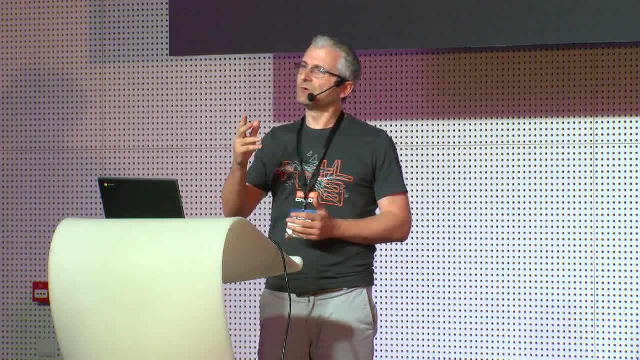 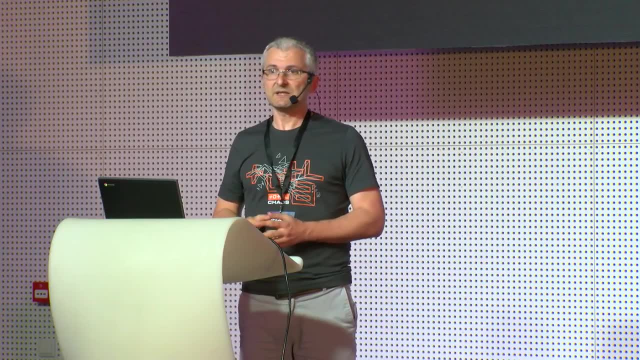 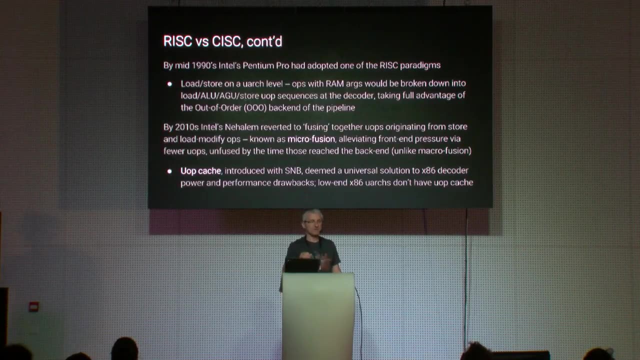 are permissible in RISC, And by few I mean two or three. And the last differentiator between RISC and CISC is that today RISC architectures still have the much larger visible register file compared to CISC architectures. Now, when I said that CISC architectures started adopting RISC DNA, I mean 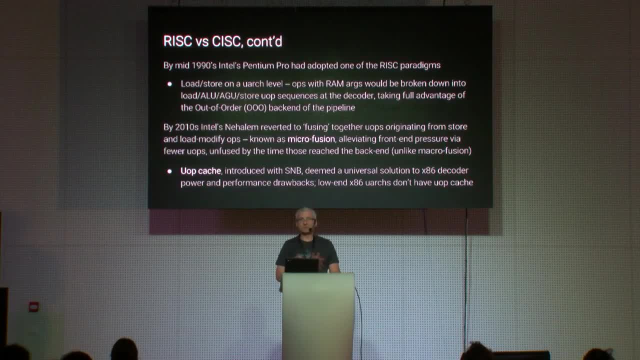 the following: By mid-1990s, the most performant Intel CPU, at that time, the Pentium Pro, actually adopted the most essential RISC paradigm, the load-store paradigm. But the way it adopted it, they didn't break their ISA, their backward. 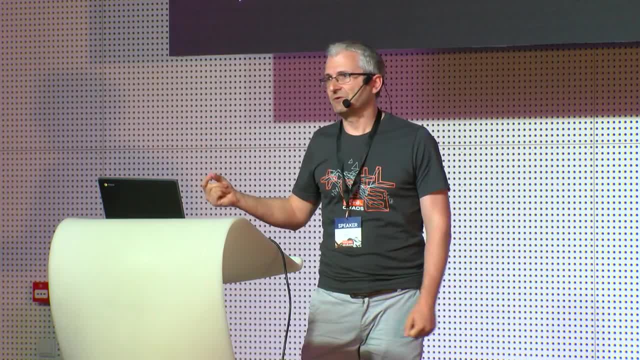 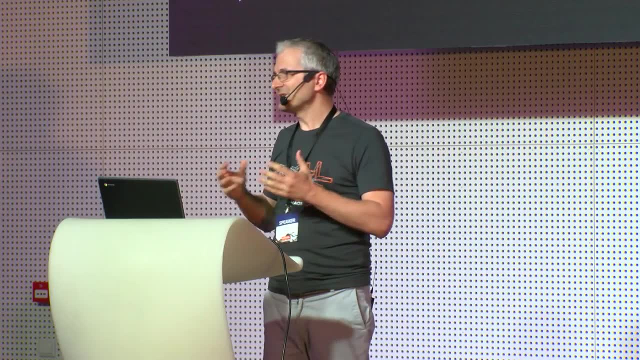 compatibility. They implemented it on the micro-architecture level. Now, what's the difference between an architecture and a micro-architecture? An architecture is just a contract. It's a programming contract. The micro-architecture is the actual implementation of that contract. in silicon, A micro-architecture has 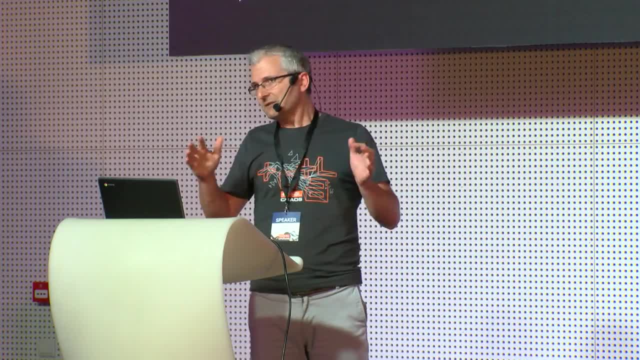 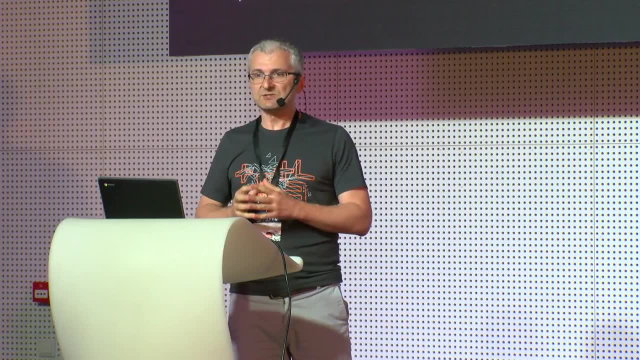 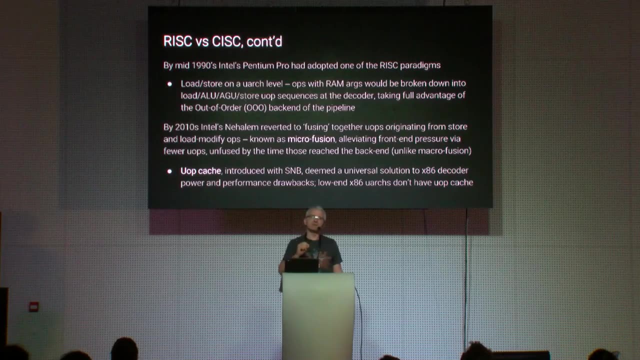 performance characteristics, An architecture not so much Well, at least at first glance. So what happened is that basically any instruction that a Pentium Pro would encounter that had a RAM argument in the instruction would be broken down into micro-operations. That really helped the. 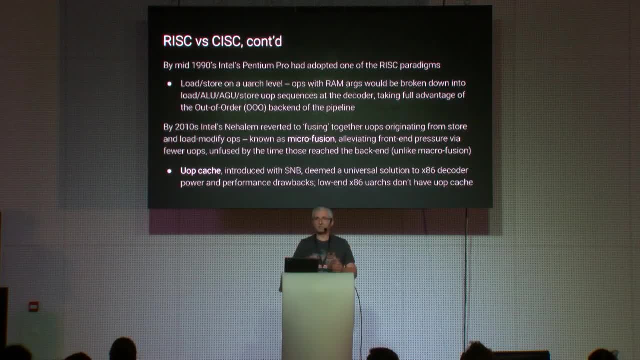 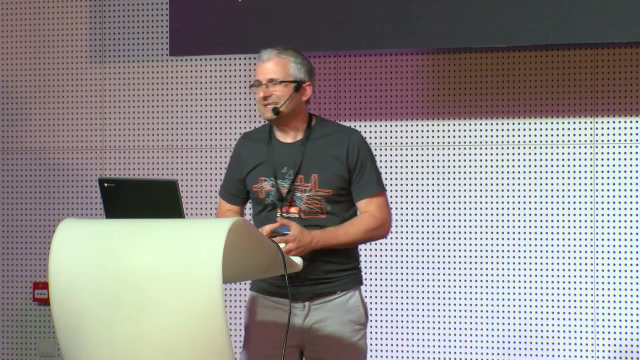 pipeline to make good use of the out-of-orderness of the back end of the pipeline, where the actual parallelism occurs. Now, 20 years later, Intel sort of stepped back on that. They reverted, They changed it a bit And, starting with Intel Neclem, they started implementing a 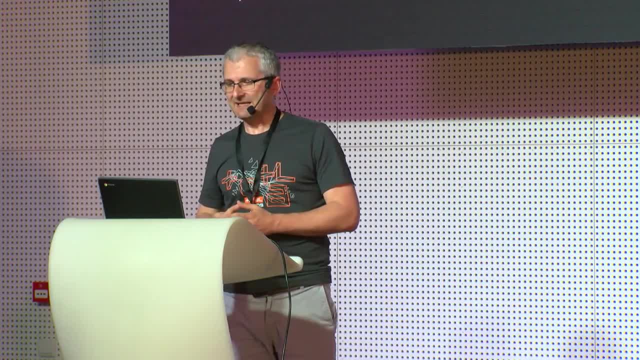 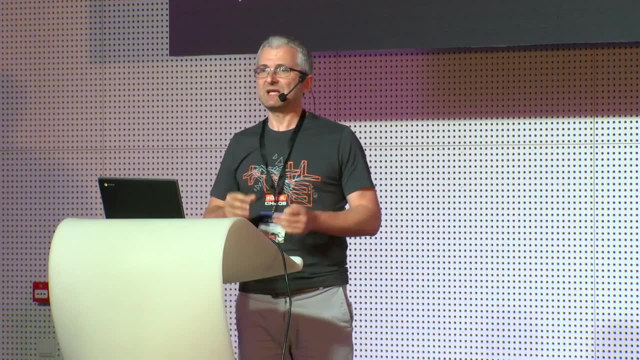 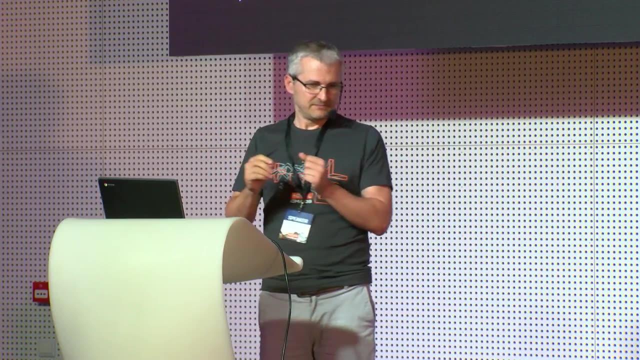 technique known as micro-fusion. What micro-fusion does is that whenever an operation on the front end was broken down into such micro-operations that would have to do with memory access, those operations would be fused together. They would be batched into a single. You can think of a single micro-operation. 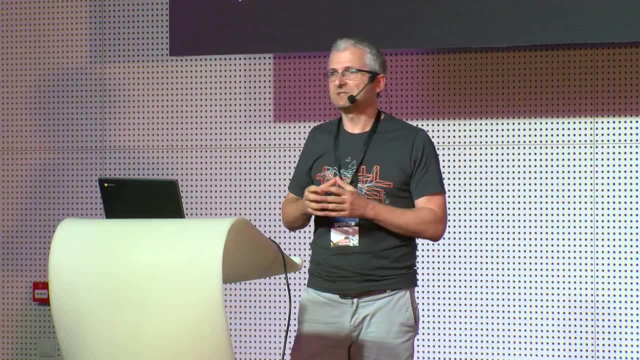 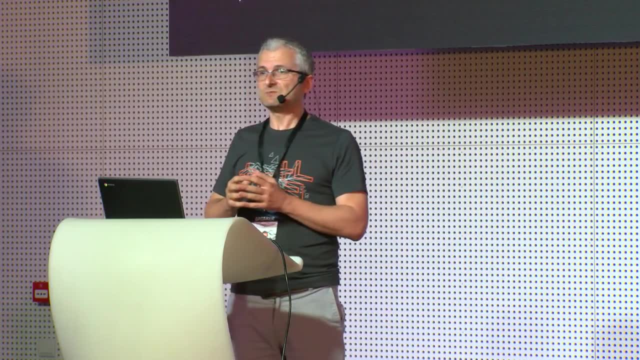 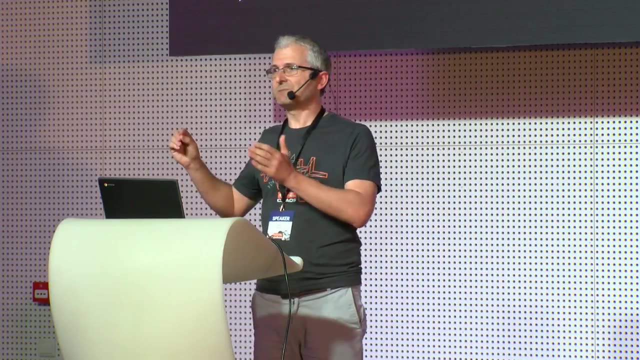 that travels through the pipeline. Now, the whole point of this optimization was that the decoder would not saturate the front end of the pipeline with so many micro-ops, but micro-ops would be fewer. That would alleviate the pressure on the front line. But by the time that such a fused micro-operation would reach the 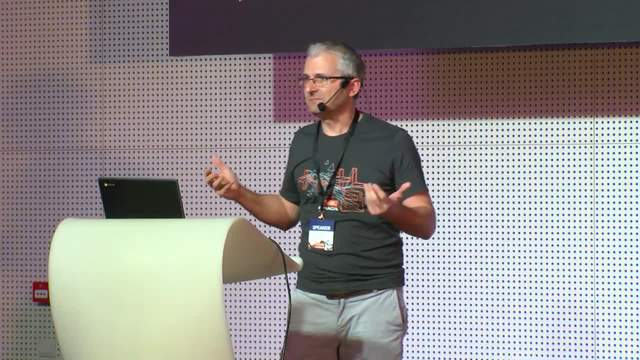 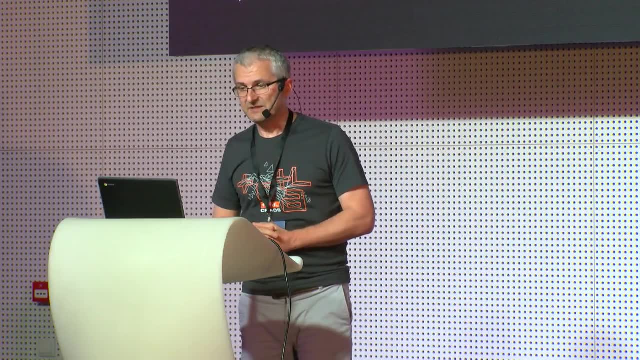 back end it would be again unfused and full use of the parallelism inference. parallelism would be taken advantage of. The next step that happened in the right successor of the Neclem, the Sandy Bridge. was that a micro-op cache? 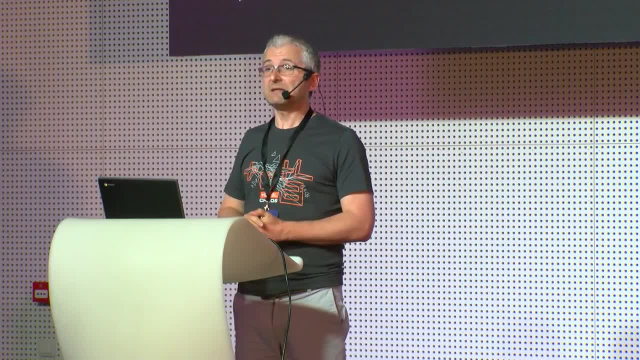 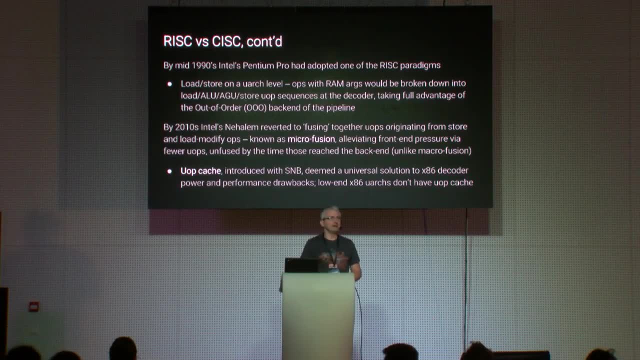 was introduced in the in the micro-architecture. That micro-op cache was deemed the great solver of all x86 decoder and power issues. Ironically, entry-level x86 micro-architectures don't have a decoder cache. They cannot afford it. They don't have the 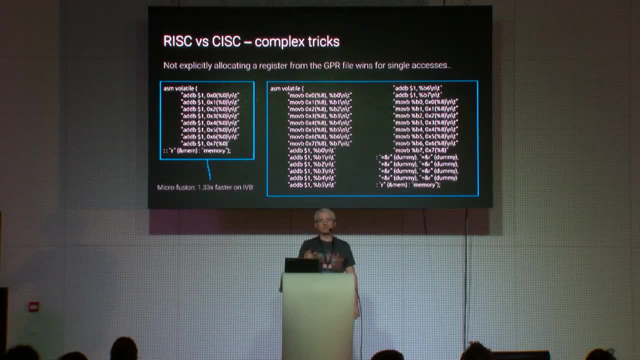 transistor budget. Now, just to give you a taste of what micro-fusion does, on the left-hand side you see a code that is semantically identical to the code on the left-hand side. This is inline assembly- gc inline assembly. so I do apologize for. 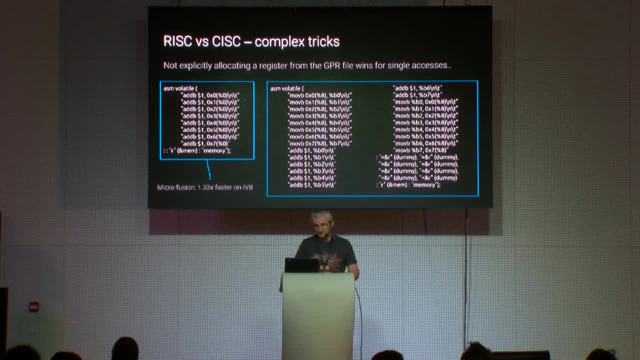 the AT&T syntax that seems many people are not familiar with. But at least you can copy and paste these snippets in the gc compiler and it'll compile. So what we do in the code snippet: We increment eight locations in memory, eight byte locations. 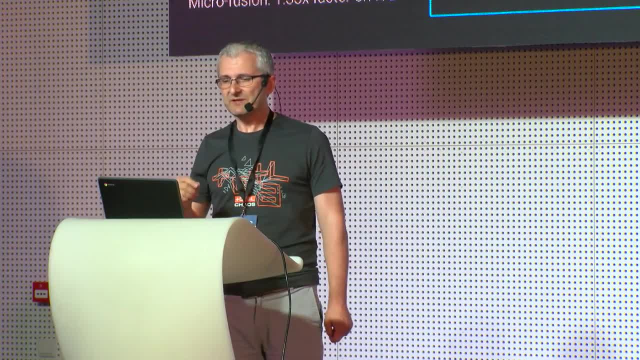 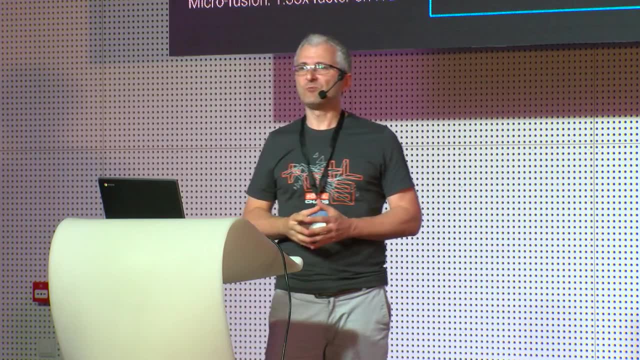 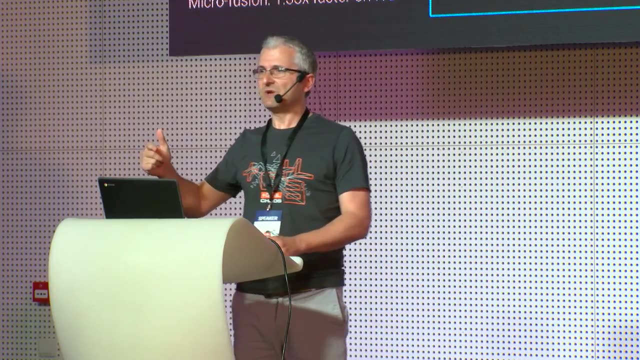 in memory by one, And we on the left-hand side we increment them with such complex instructions that reference memory addresses. On the right-hand side we have broken this down into more micro-op-like code. We deliberately go and read the addresses from memory into explicit registers. Then we do the addition onto the. 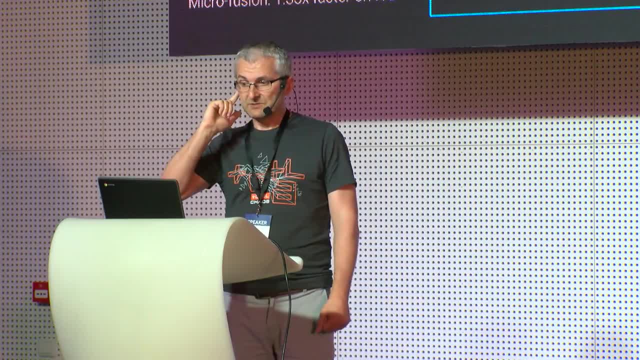 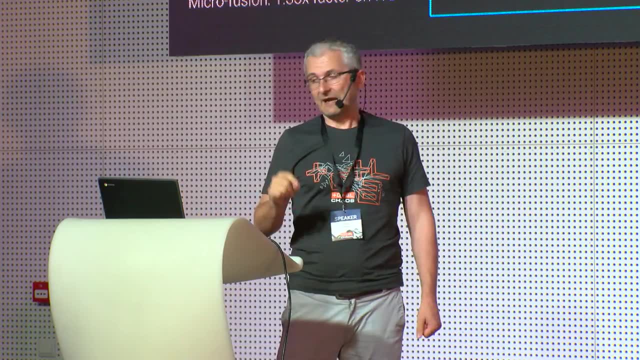 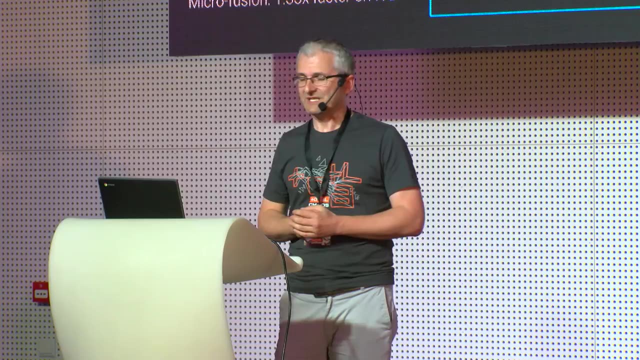 registers and then we store back the registers in memory. So before Necklem that code would perform pretty much identically on an Intel architecture. After Necklem the left-hand side would be faster because of micro-fusion. Actually, on an Ivy Bridge the left-hand side code is exactly 33% faster than the right-hand side code. 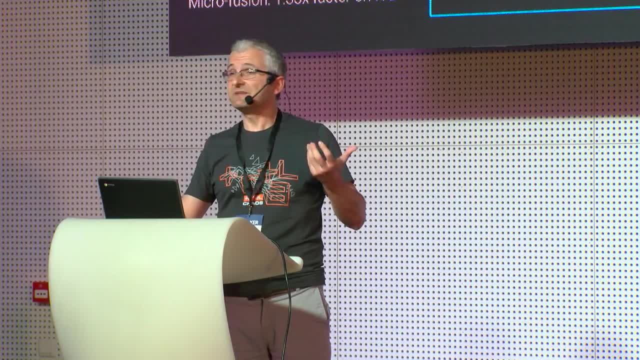 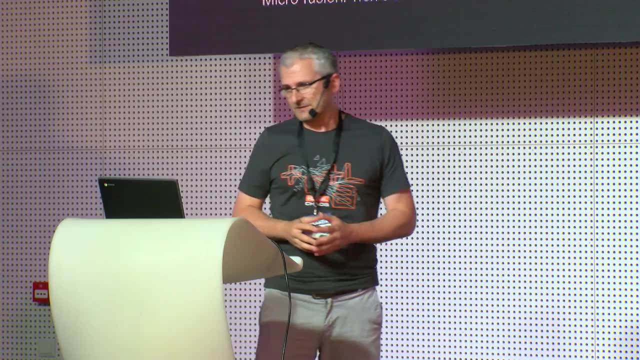 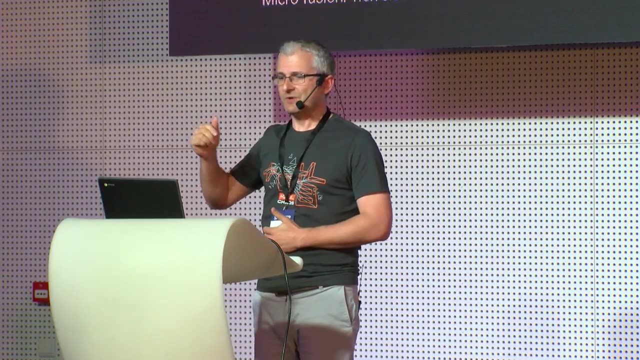 So micro-fusion must be something very, very useful, right? Well, it has its drawbacks. Here on the left-hand side code we have an example of a code that goes and touches a memory address twice in a row. So here we increment the same address in memory twice. 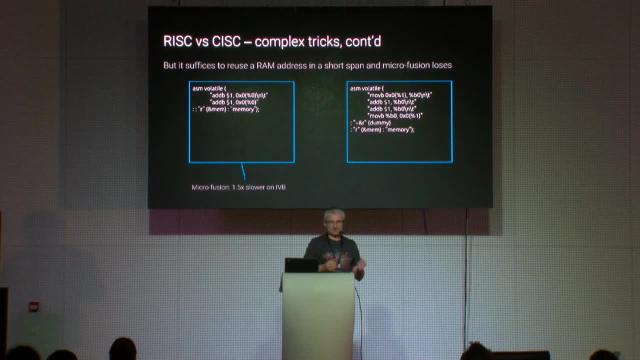 On the right-hand side code we do something that is semantically identical: We load the memory address into a register, we increment the register twice and then we store it back. Now the left-hand side code is actually 50% slower than the right-hand. 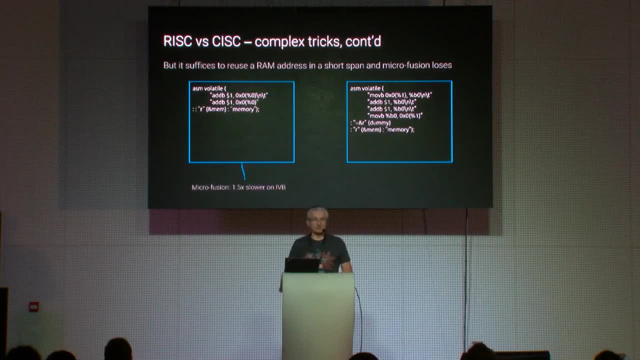 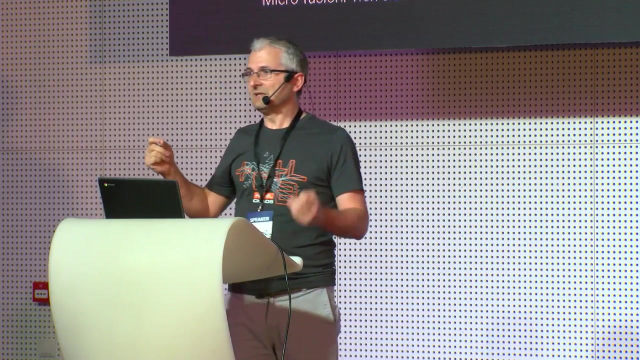 side code on an Intel Ivy Bridge. So that benefit of the micro-fusion works only for streaming type of code. So code that touches memory addresses once and doesn't bother with them anymore. As long as we have a reuse, a memory address in a short span of code, micro-fusion loses. 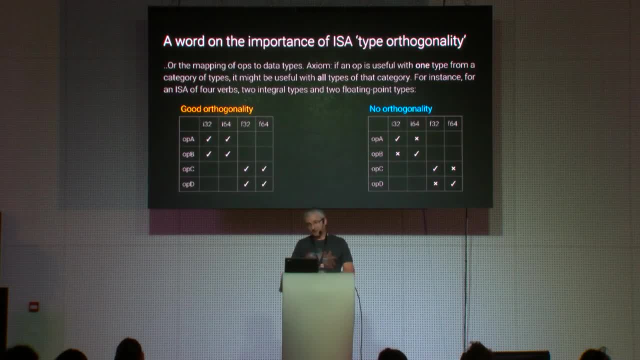 And before we actually move to the interesting part of this lecture, the case studies, let me say a word on ISA type orthogonality. When we say ISA orthogonality we usually mean that the ISA allows the combination of all kinds of operations. 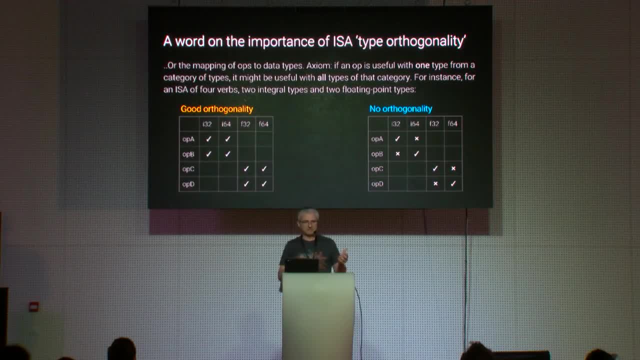 with all kinds of addressing modes. So the higher the capability to combine operations modes, the higher the ISA orthogonality. But we also should mention that type orthogonality is equally, if even not more important. So imagine we had two hypothetical ISAs. One: 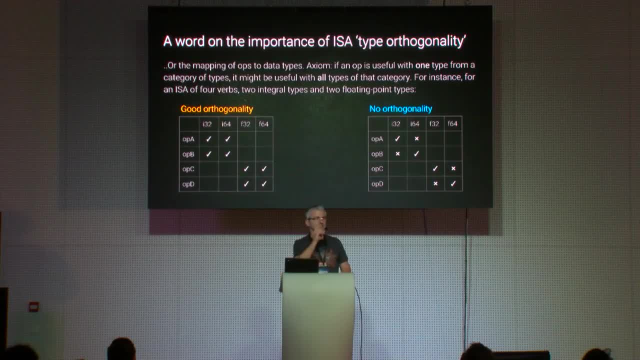 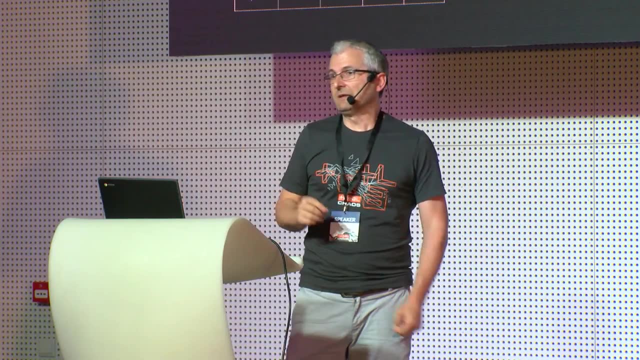 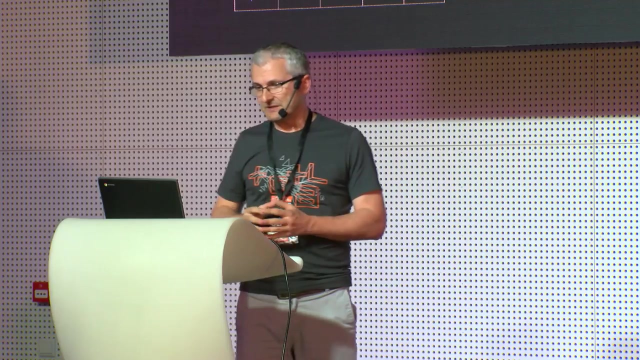 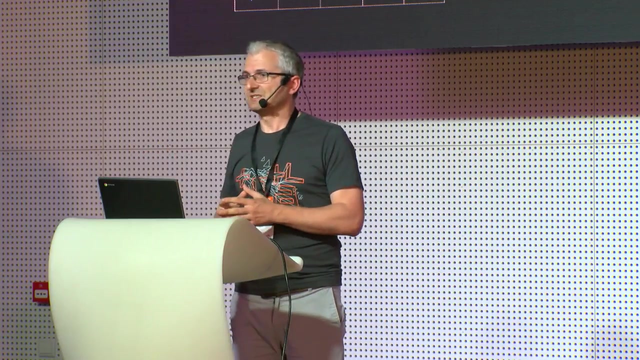 of them had four verbs and two categories of types: Two integral types and two floating point types. So a very good orthogonality ISA would be one that for each integer operation would be available on all integer types, Likewise with the floating point operations They would. 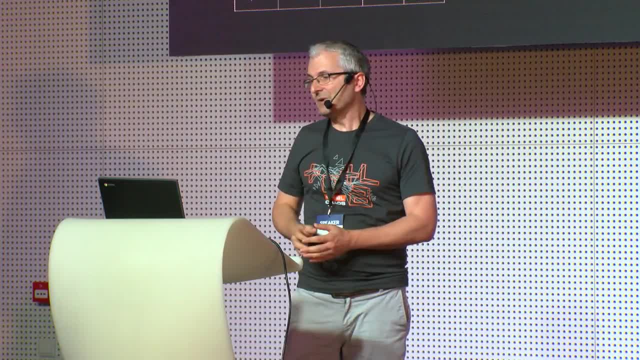 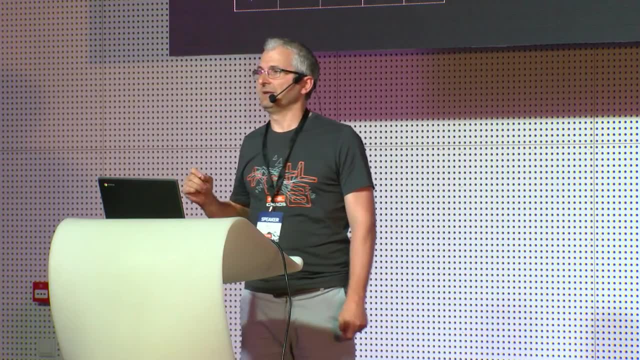 be available on all floating point types. On the right-hand side, we have an ISA that has no orthogonality whatsoever. Each and every operation works only on one data type and one data type only, Even though it actually makes a pretty good sense that if an operation 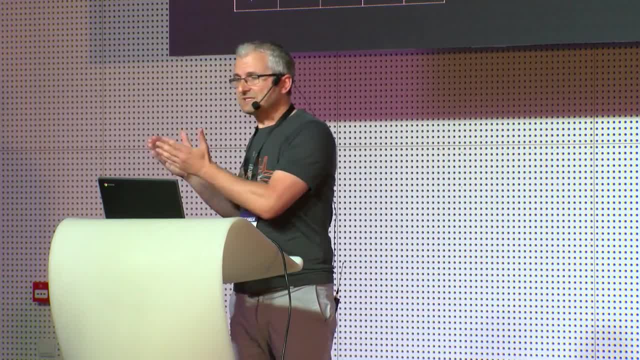 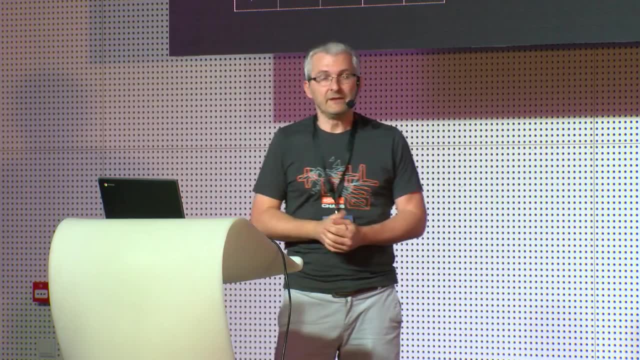 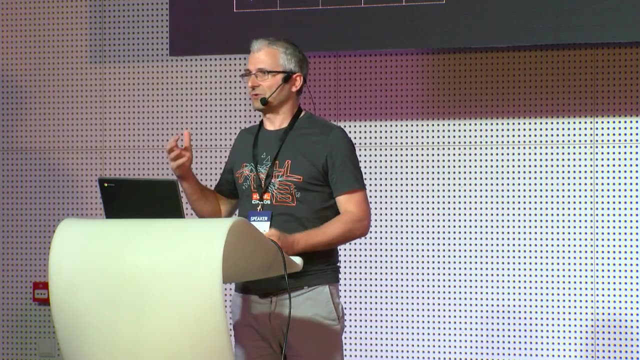 is useful for 32-bit integers, it might be also useful for 64-bit integers. Actually, for most arithmetic operations, that is a truism. So what are the disadvantages of architectures that are not well-typically orthogonal? The disadvantages is that each time that you write a high-level expression in a language, the 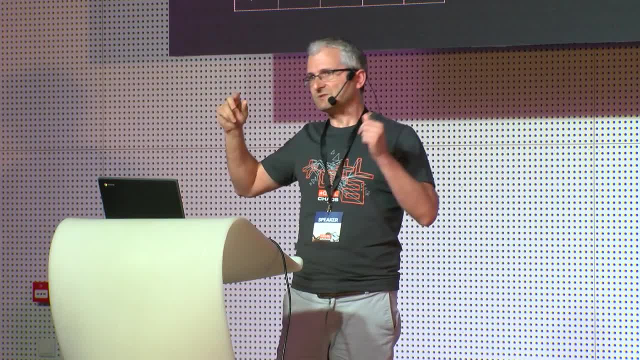 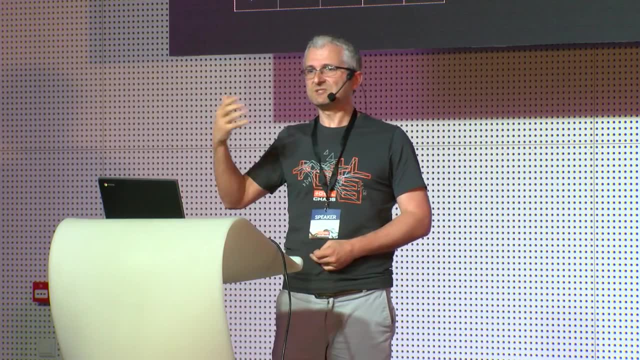 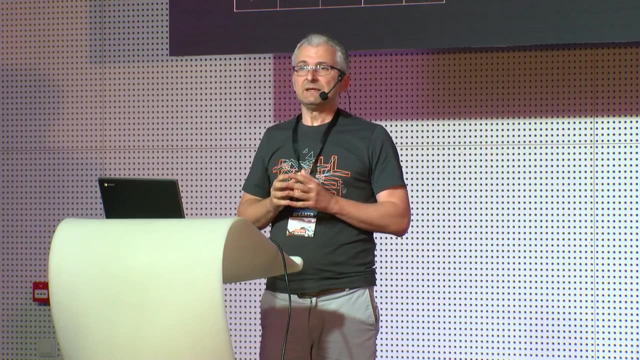 compiler has to convert your data to the type that the processor knows about and do some magic with it, With the data. do some small subroutine to process your data in the way that you would expect it to happen. Now this conversion back and forth, if it's only for the conversion. 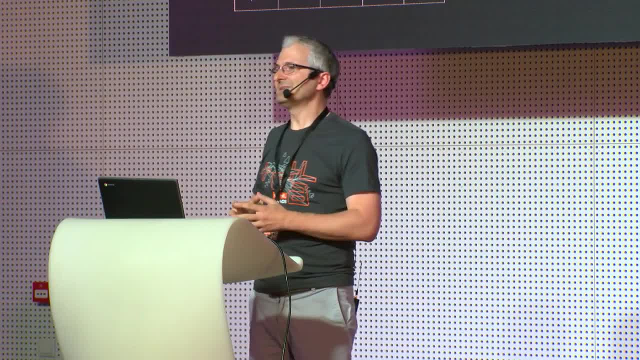 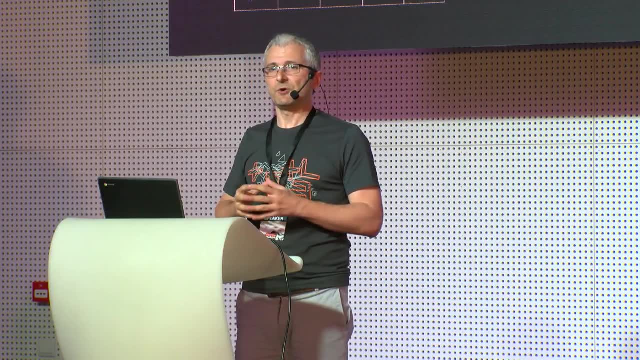 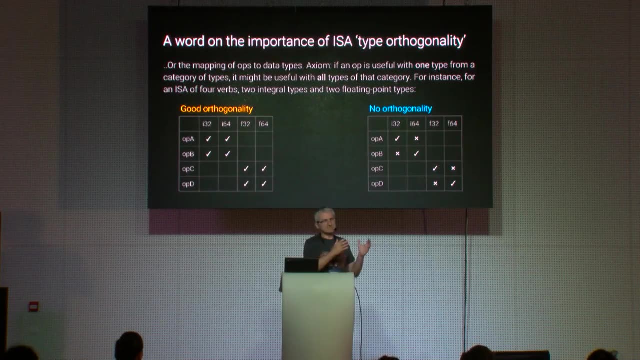 means the introduction of data dependencies in your code, And data dependencies are the arc enemy of instruction-level parallelism. The moment data dependencies enter your code, that moment your instruction-level parallelism drops. Of course I'm speaking of a general case. You could write specific code that exhibits: 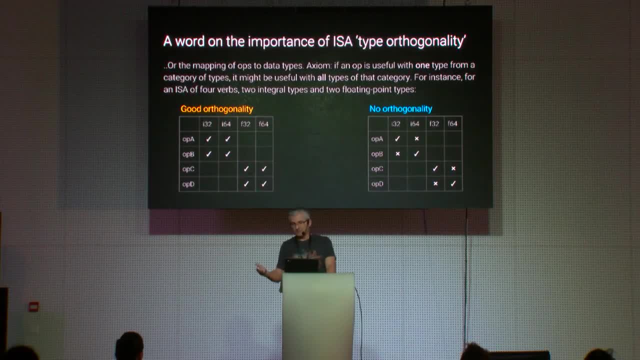 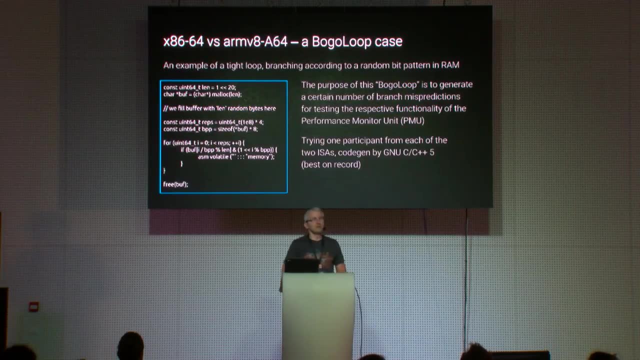 very high levels of data-level parallelism, even using non-orthogonal instruction sets. So let's move on to the first actual case study. The first case study is something that I've called Bogle loop, in reference to the famous Linux kernel Bogle MIPS. A Bogle loop. 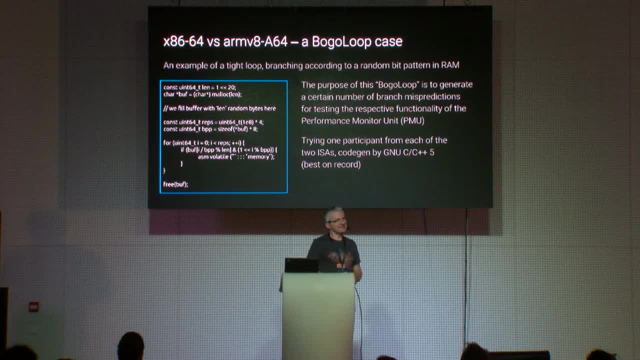 in our case, is a loop that does nothing useful and yet it has a desirable side effect. This Bogle loop of ours is actually a loop of 400,000 iterations. In this particular case, I've decided on this number. In the last case study, my result was the difference between the common picture elements. 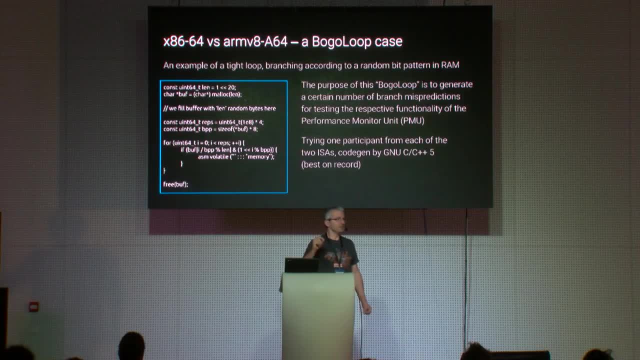 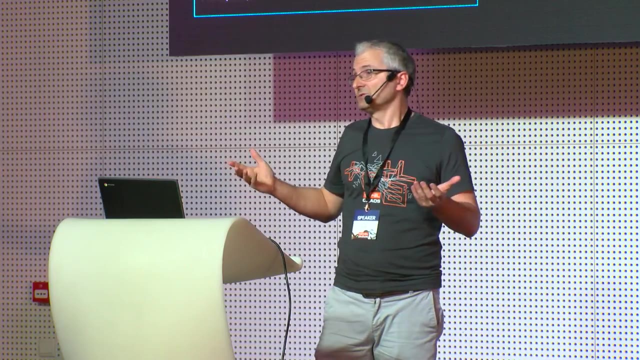 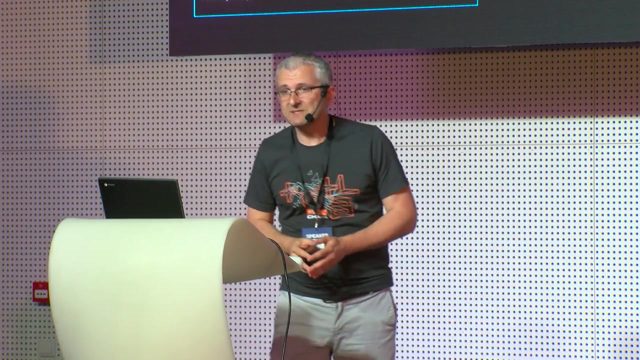 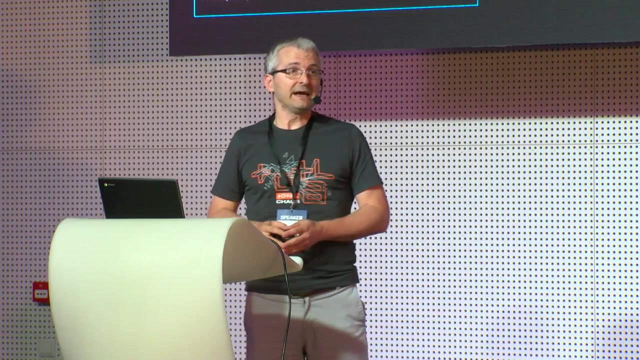 6 and 50, and 5.. Here I've selected two whole室 types of Bogle element that are not identifiable. Can you help me with? this is perfectly platform-independent, platform-agnostic, as long as you have a GCC-compatible compiler for the platform. 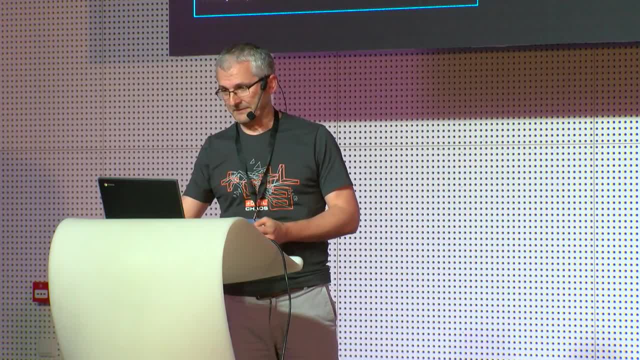 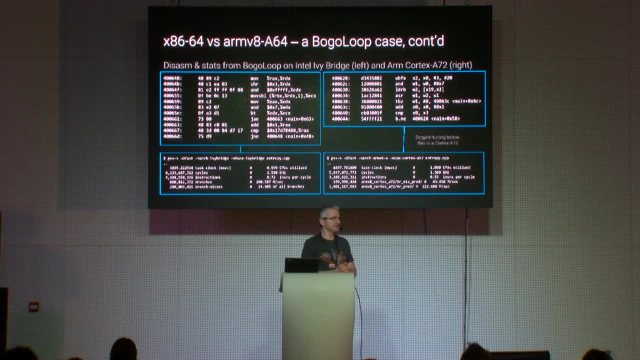 I'm looking at you, Microsoft. So let's get actually down to the nitty gritty details. On the left-hand side, we have the disassembly from the GCC5 version of the code on the Intel Ivory Bridge. On the right-hand side, we have the disassembly: 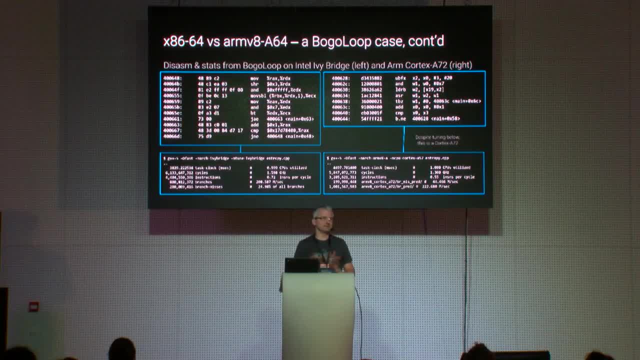 from an ARMv8 64-bit. The A64-bit is the name of the ARM instruction set introduced by ARMv8 for 64-bit mode. What is the first thing that makes an impression in you looking at this picture? Well, the left-hand side code is three instructions longer. 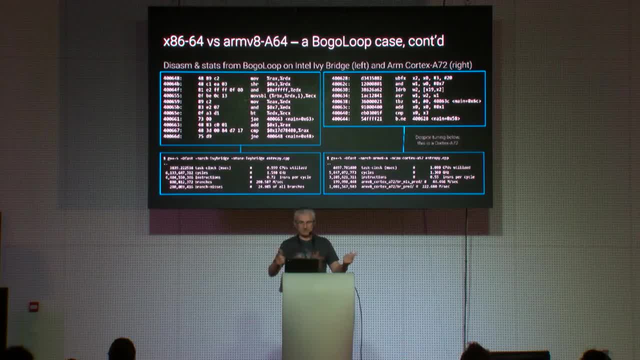 than the right-hand side code. Let's take a closer look at that. So the first group of instructions in the left-hand side code are three instructions that are semantic. They're literally equivalent to one instruction on the ARM And the semantics of that instruction. 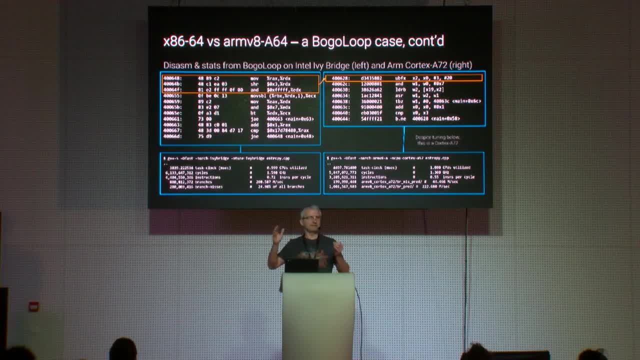 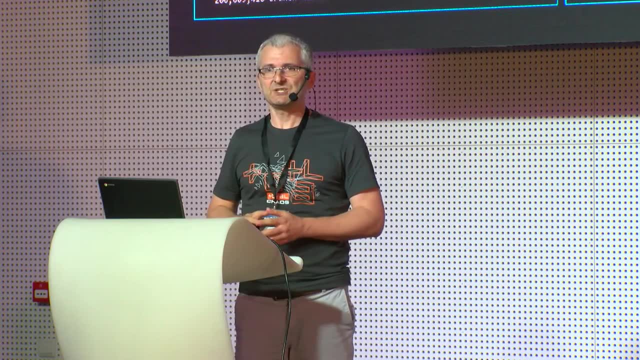 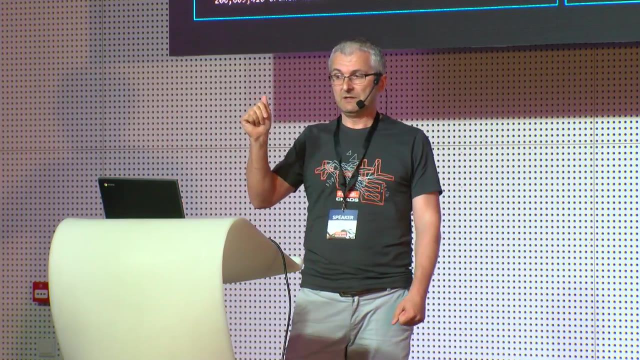 is: take a bit from this position in the register and extract that many bits from that position. Now ARM, along with many other RISC architectures, have a deliberate instruction that does that, And it does it pretty efficiently. They usually have a latency of one clock. 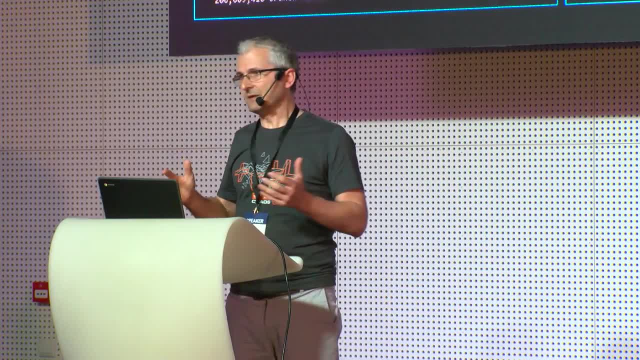 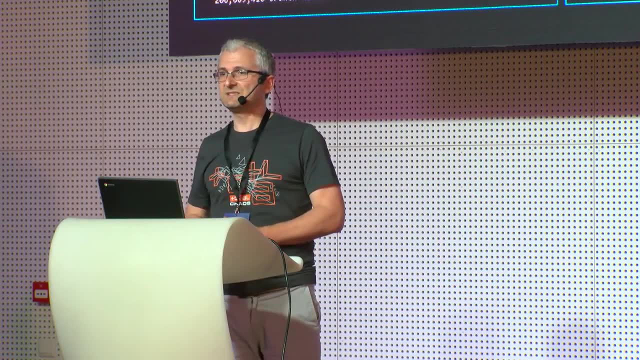 The three instructions on the left-hand side do the same on an Intel. It's semantic. It does exactly the same thing. Let's move on. Now we are at the group of instructions. that are, five instructions on the left-hand side and four instructions on the right-hand side. 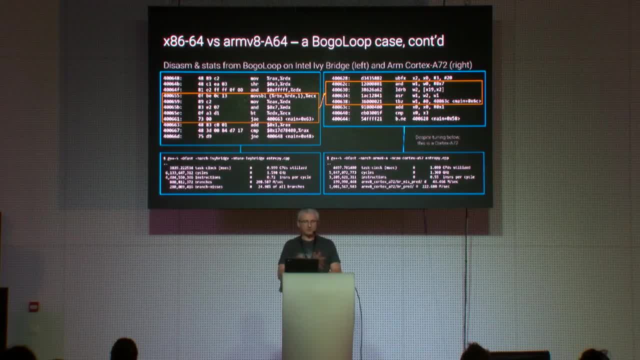 Again the right-hand side. so what do they do? They basically read a byte from memory And they check a particular bit position in that byte and then perform a useless jump based on that bit. The useless jump is the whole boggle loopness of our code. 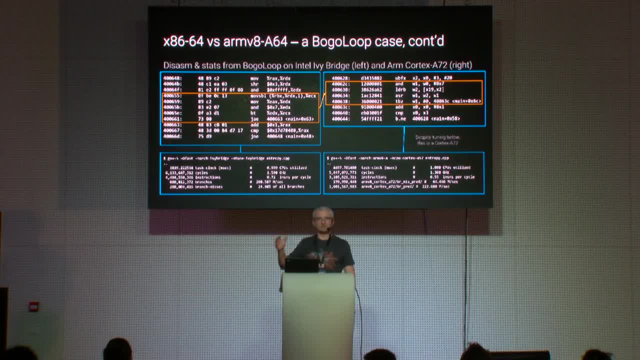 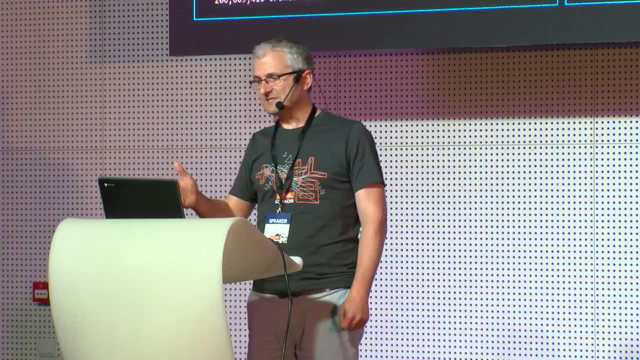 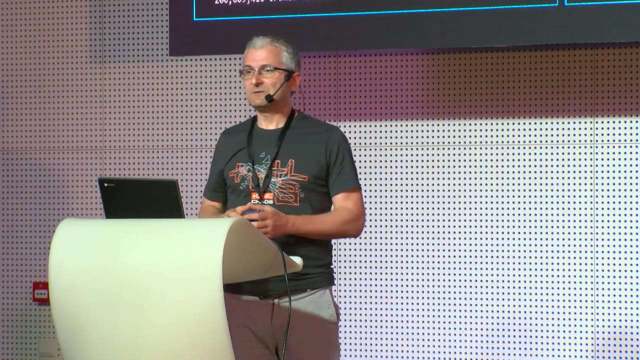 And this useless jump is the one that we expect the performance monitoring unit to actually measure: whether the jump was predicted or mispredicted. So what can we say about this code? We can say that the code is fairly similar in both architectures, But on the left-hand side, because there 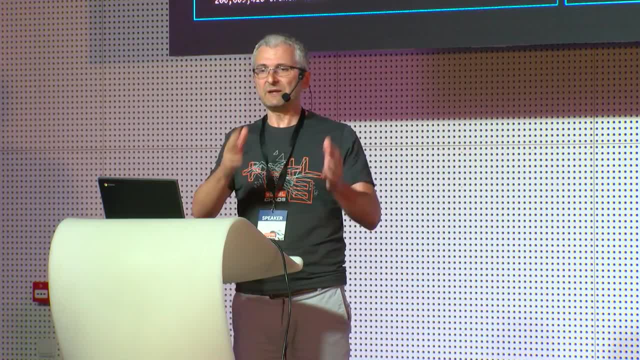 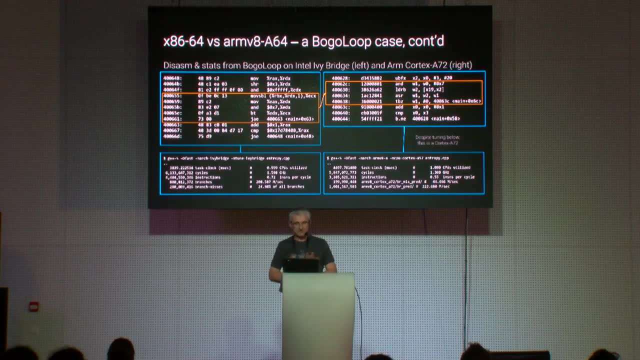 is an instruction on the Intel ISO that can do comparison and branch. here Intel actually loses one instruction until pii, Until I get our model, then branch. it also loses in another here, in another instruction where it has to do an explicit move. but let's say that that's not bothering us at the moment. on. 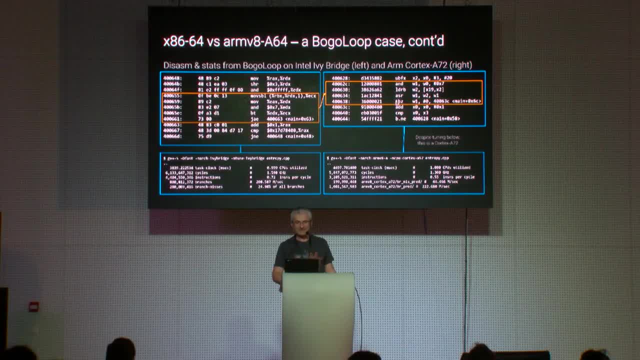 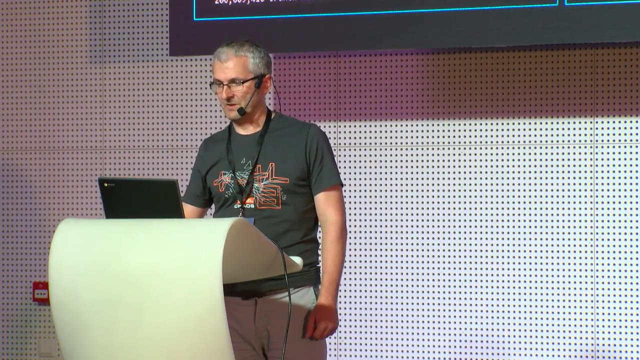 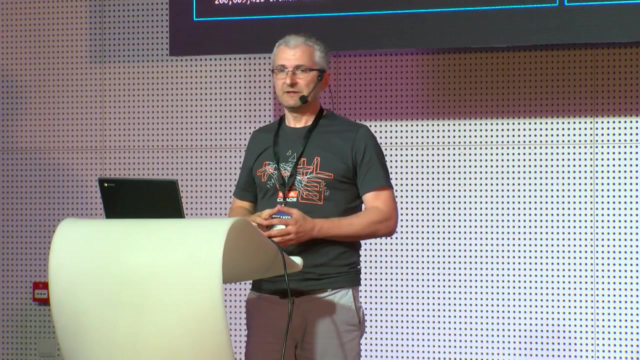 the right hand side, the arm can actually do a test and branch instruction. that is, it tests, in this particular case it tests a bit at position zero, where zero is a literal, and branches upon that upon, upon the result of that. and the third group of instructions is the actual loop, iteration, closure, the, the. 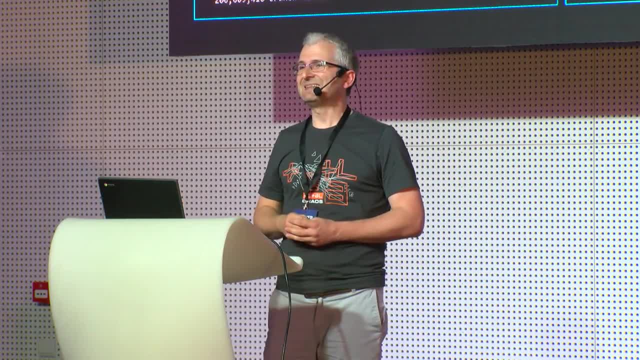 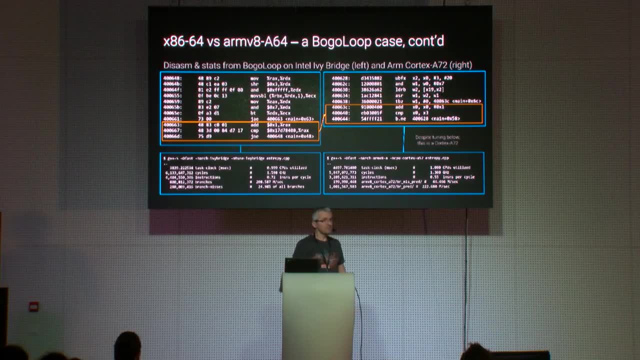 thing that counts our loops. here there is virtual identity between the left hand side and the right hand side, so at the bottom of that picture we can actually see the perf results. the, the Linux perf, is a very good profiler and event-based profiler that I use extensively at work. so here we see what. 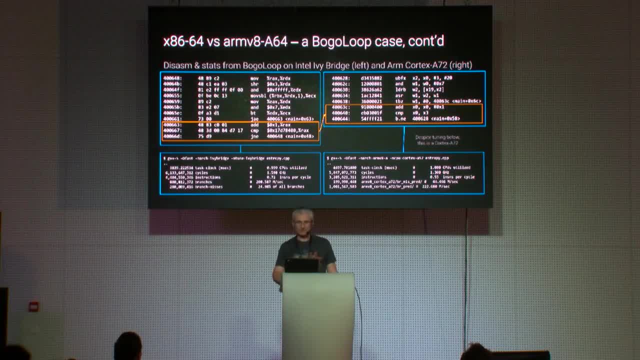 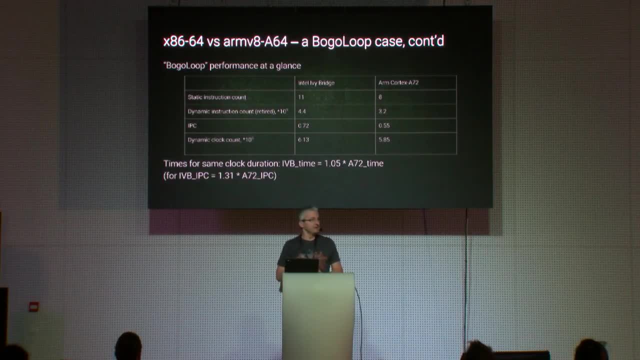 happened with the red, with the left hand side code and the right hand side code. in case you don't actually see the nitty-gritty print, I have prepared a digest table for you. so here we have an Intel Ivy Bridge versus a Cortex a 72. 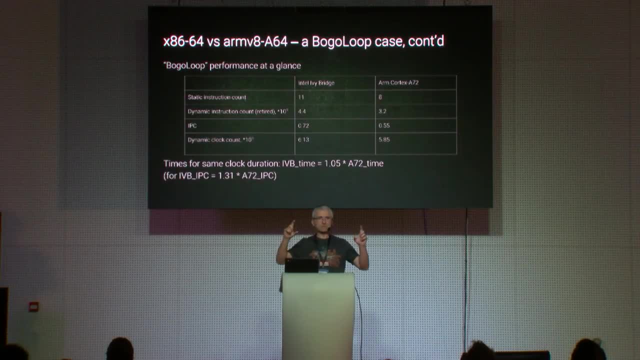 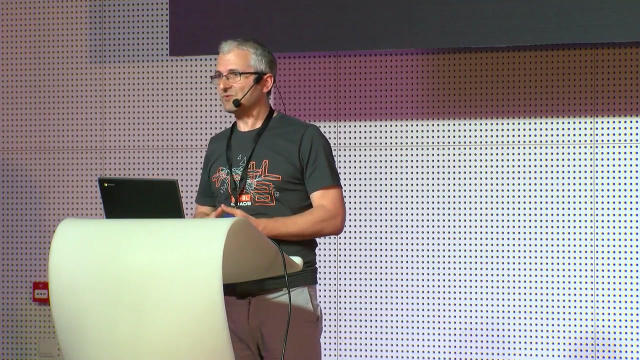 again, just by counting the instructions in our loops, we see that there are 11 static instructions in our Bogo loop on the Intel, versus 8 static instructions, and those are the kinds of instructions that we see in our Bogo loop. now, because I will loop iterates 400 million times, that translates roughly to four point. 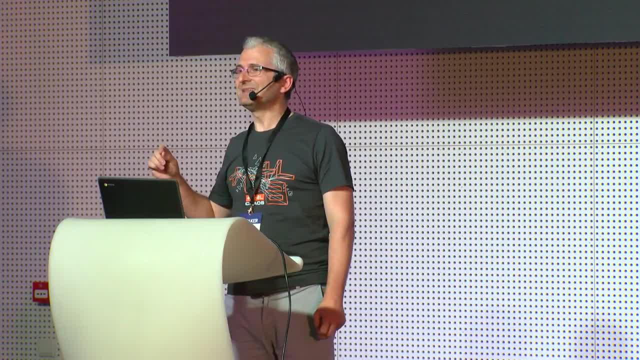 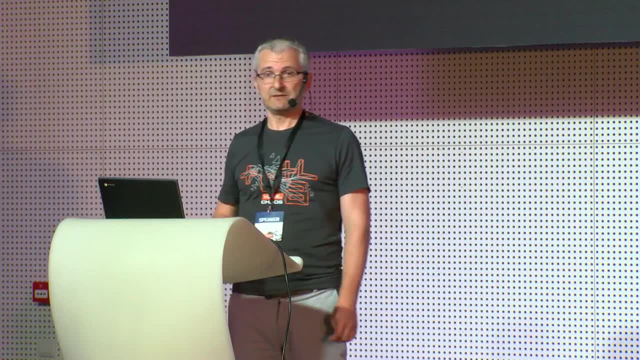 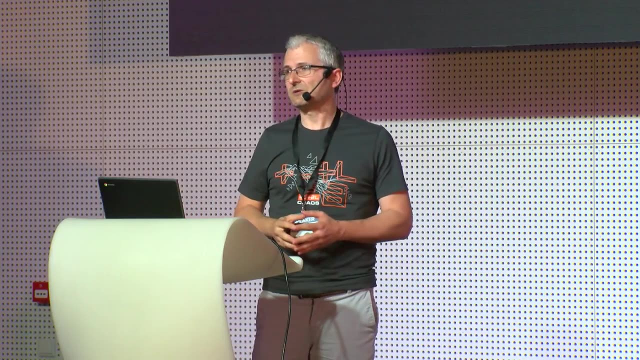 four, four billion instructions, dynamic instructions on the Intel, versus three point two billion dynamic instructions on the arm. now for computed instructions per clock metric, computed by perf, again, of 0.72 instructions per clock on the Intel and zero point fifty five instructions per clock on the arm we get. 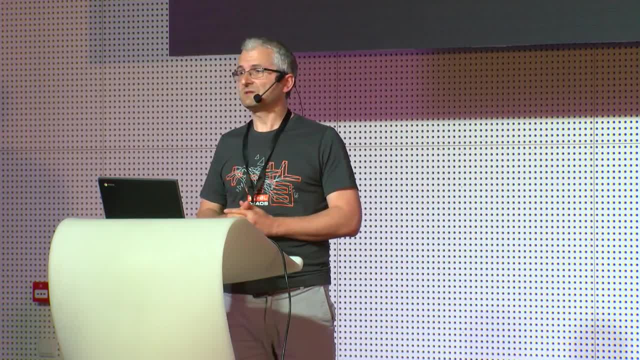 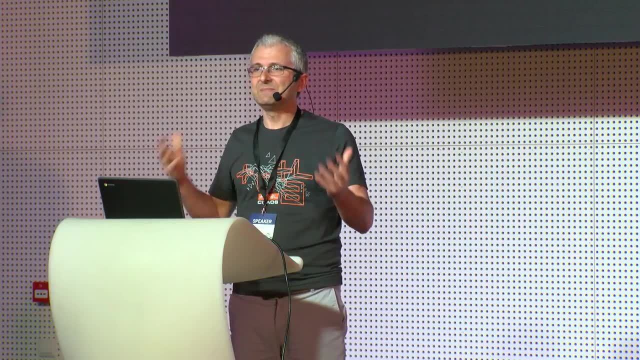 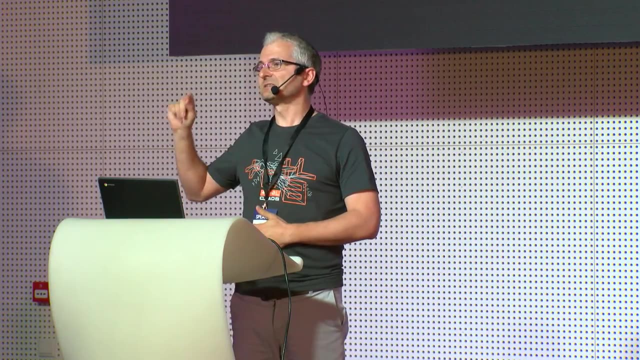 of dynamic clock count of 6.13 billion on the Intel and 5.85 billion on the ARM. What does that mean? That means that if these two processes were running on the exact same frequency, the Intel would be 5% slower than the ARM. 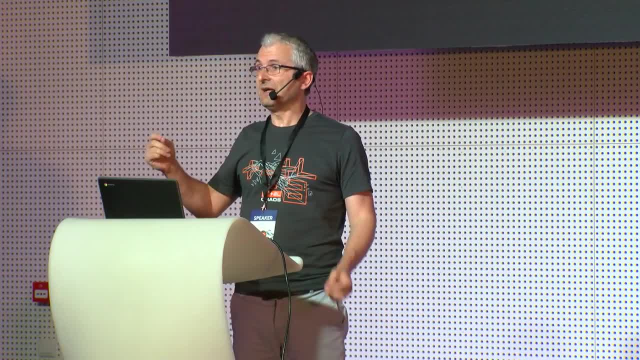 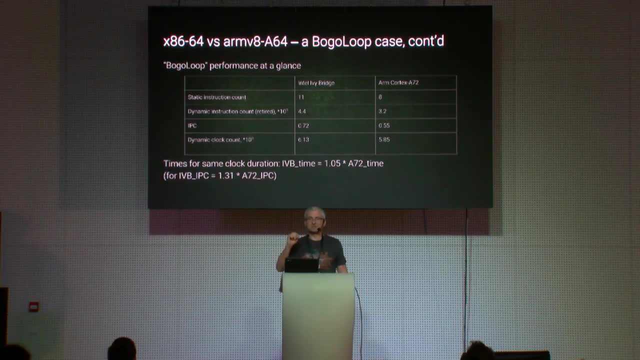 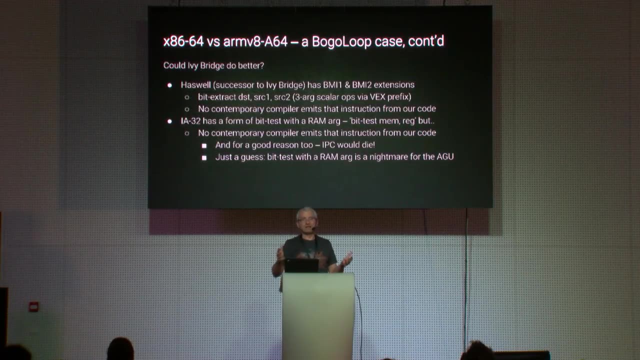 even though it has a 30% instructions per clock advantage over the ARM. How does that happen? It happens because the code is actually shorter And the instructions per clock difference is not that big. So here we could normally ask ourselves: could the Ivy Bridge have done any better? 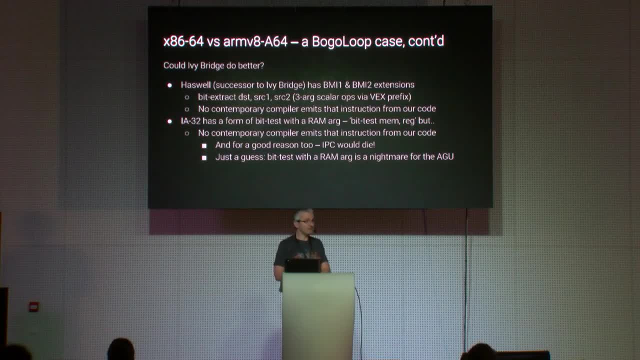 Is that the best that it can do Now? for the Ivy Bridge perhaps, but the immediate successor to Ivy Bridge, the Haswell, has a deliberate bit extraction operation So it can do exactly as the ARM does. It can extract a bit from a position and a certain count of bits. 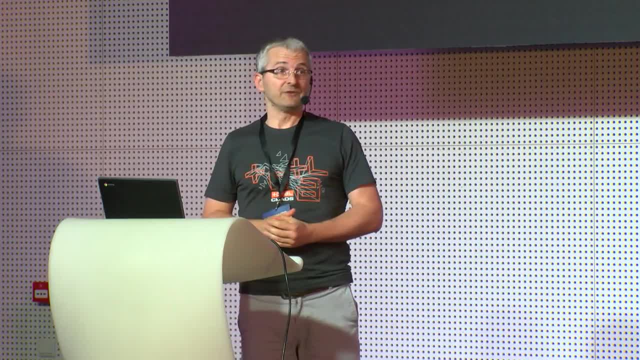 and put them in an ARM. So it can do exactly as the ARM does and put them in a certain count of bits and put them in an output register. Unfortunately, no of the contemporary compilers has generated a bit. extract instruction from our code. 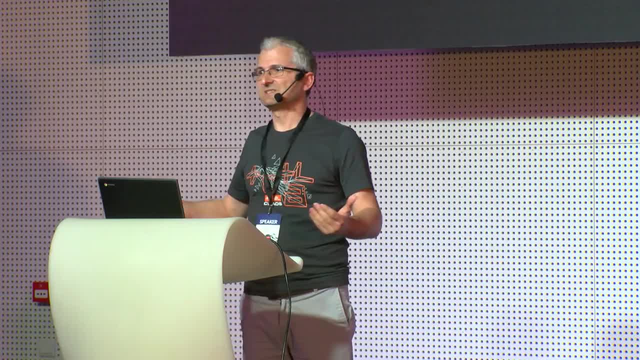 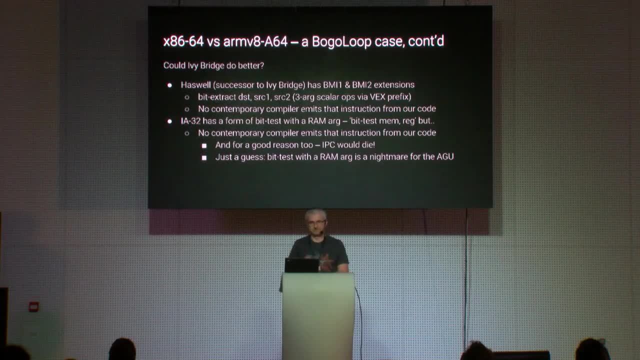 even though we have instructed it to use the full instruction set of the Haswell architecture, And by no present compiler, I mean the Intel compiler included. Okay, but that is about the Haswell. Can we actually still focus on the Ivy Bridge? 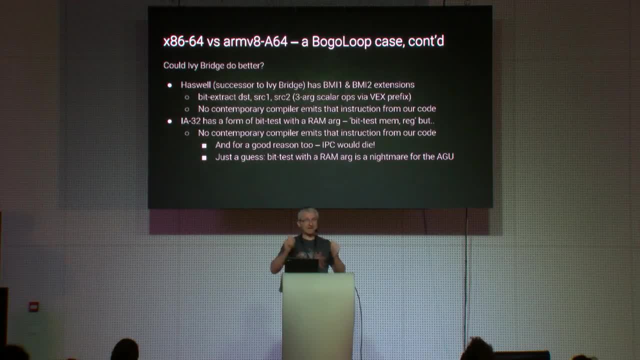 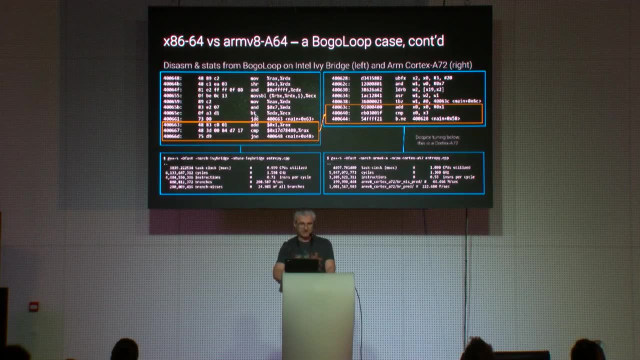 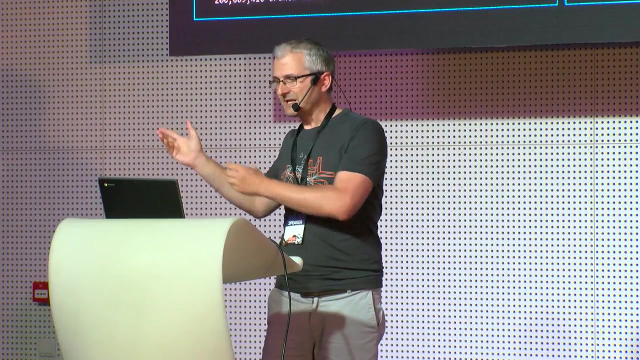 Well, the Ivy Bridge, by being a good CISC, ISA has a version of its bit test operation. Let me go back to the bit test operation. So this operation here it tests for a bit in the register by specifying which position we are interested in in the second argument. 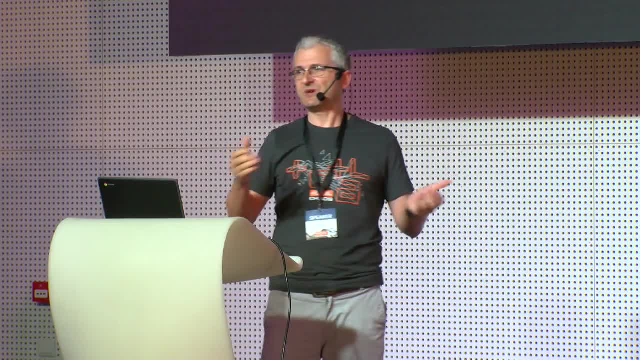 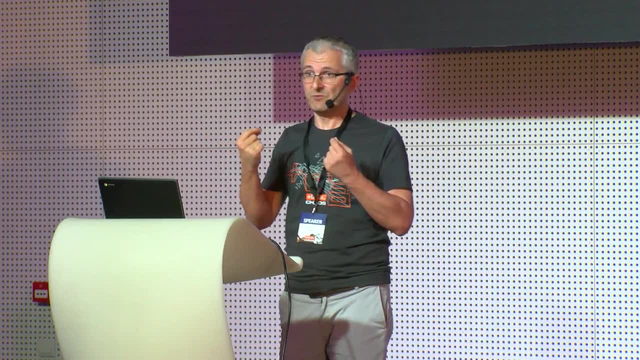 So actually the architecture has a version of this operation that can do this on memory operands. So we don't really have to read in the memory operand from memory the way we do in an explicit register. We can just test the byte in memory. 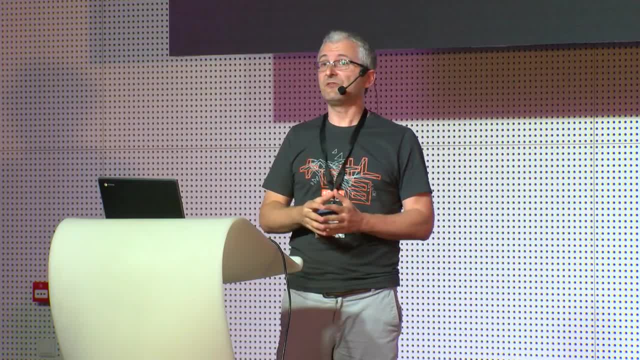 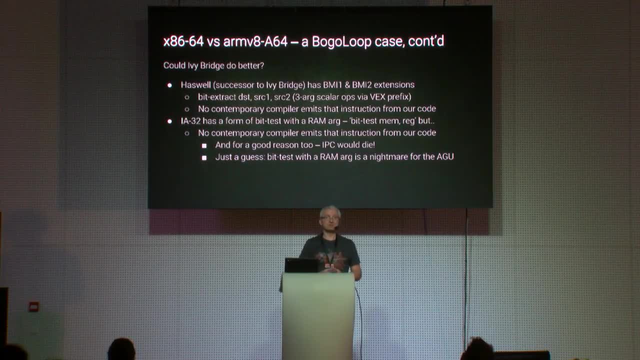 As it is in memory and perhaps take good use of microfusion. Unfortunately, what happens? What happens, is that no sane compiler would emit that instruction and no sane compiler would emit that instruction for a very, very good reason: That instruction absolutely kills the instructions. booklock metrics of the pipeline. 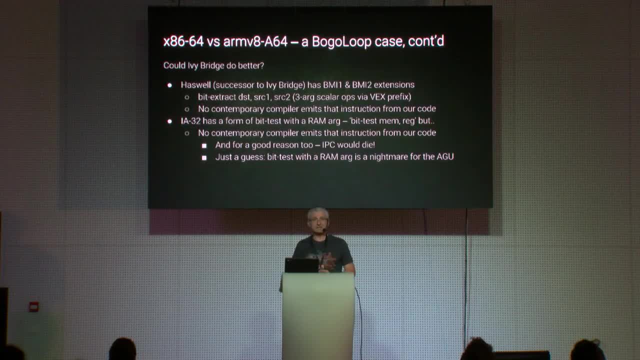 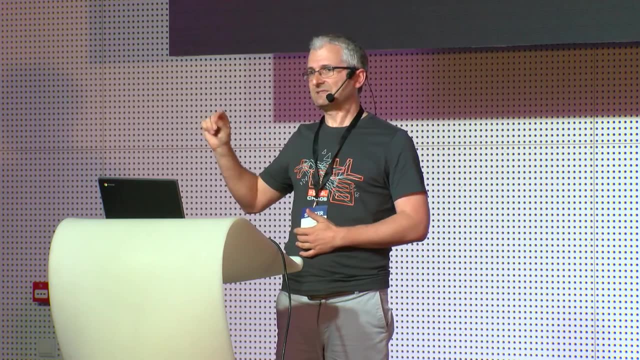 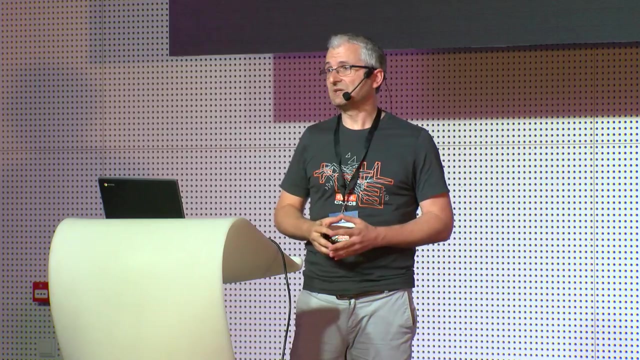 Now, without being a micro architecture architect, I would venture to guess that the version of the bit test operation that reads from memory and tests the bits from memory is an absolute nightmare for the address generation unit of the CPU pipeline. For those of you who are actually interested in microarchitectures and architectures, 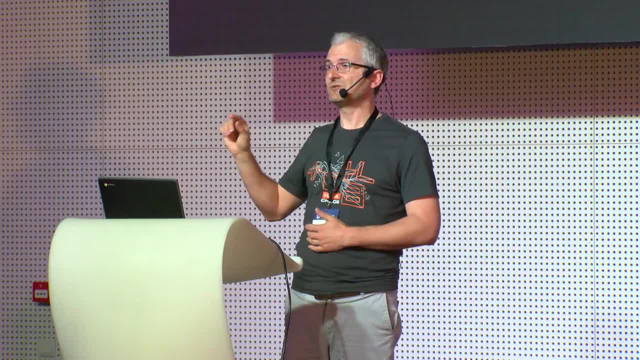 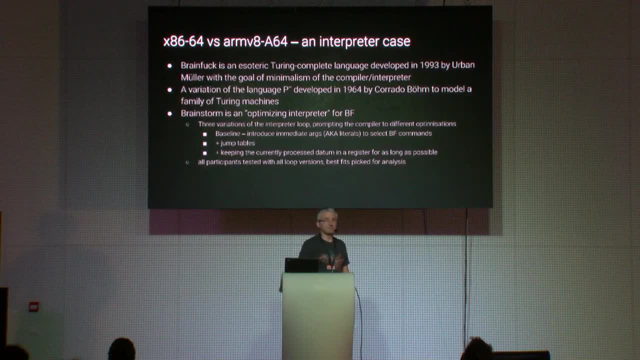 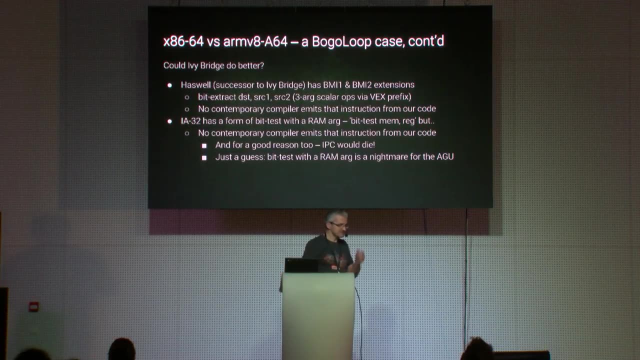 they should go and read the specification of that instruction in Intel manually to realize the full gravity of the situation of that instruction. So the next, actually the next, use case. I have to make a small disclaimer, excuse me. The disclaimer is that 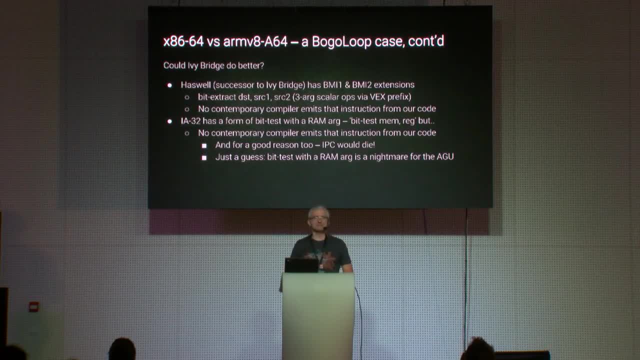 in the next use case, we will use a rather famous esoteric interpreted language which goes by a feisty name. Now, in order to avoid having the video of this talk mislabeled by some under-trained neural network on YouTube, I'll refrain from using the actual name of this language. 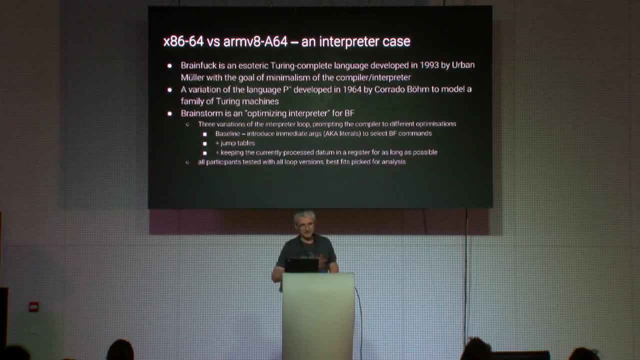 I'll just refer to it as brainfrac. So brainfrac is an esoteric, Turing complete language which was developed in early 90s by a smart fellow, Urban Muller, with the sole goal of minimalism for the compiler and the interpreter. 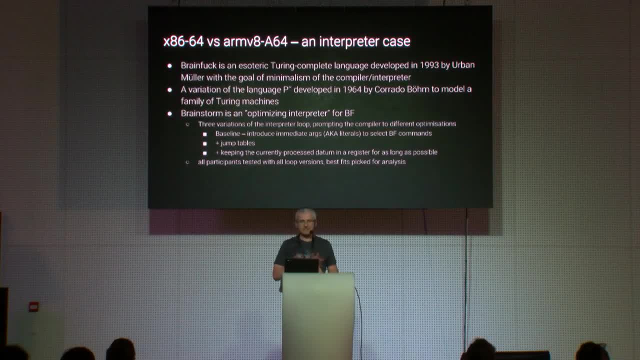 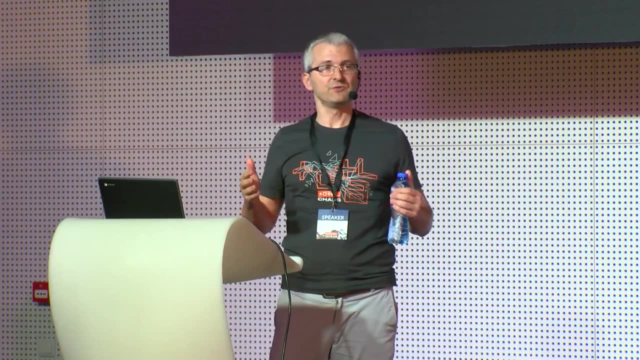 Actually, it's a variation of a language that was devised much earlier for academic purposes. The language was called P-second. It was invented by Corrado Bohm and was for the purpose of modeling a class of Turing machines. Ergo, brainfrac is completely Turing complete. 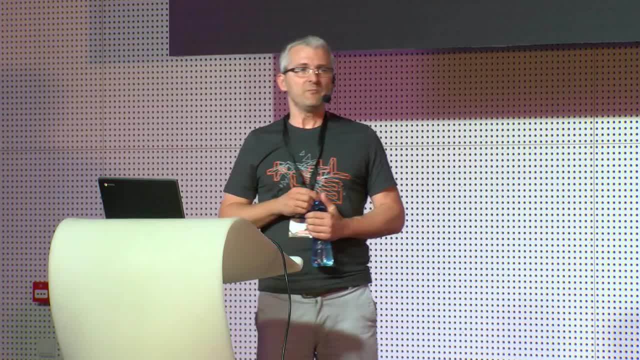 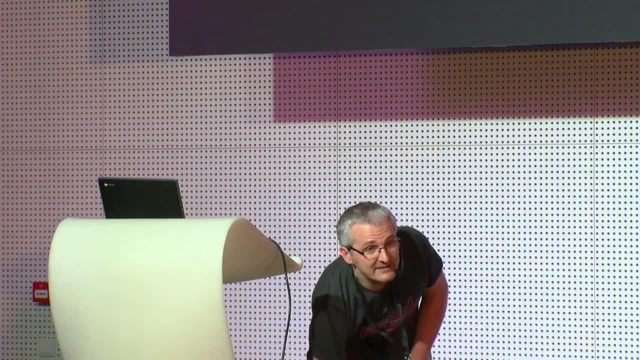 For the purpose of our tests, we are going to use a homemade brainfrac interpreter that goes under the name of Brainstorm And it is an optimizing interpreter, which means that it does certain set of transformations on the input command stream before actually interpreting it. 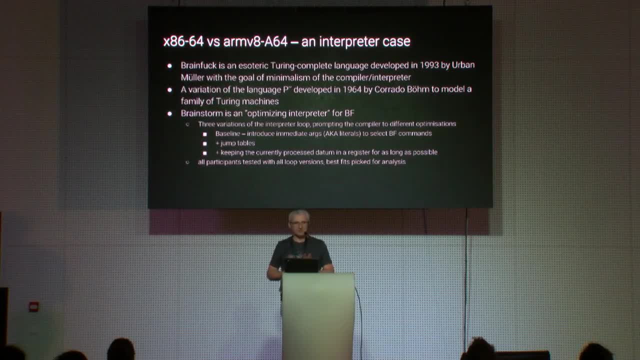 Now there are three variations of the interpreter loop, of our Brainstorm interpreter, and they are all made with the goal to push, to prompt the compiler into ever-slightly optimization techniques. First, there is a baseline optimization in which we actually introduced the notion of literals to the language. 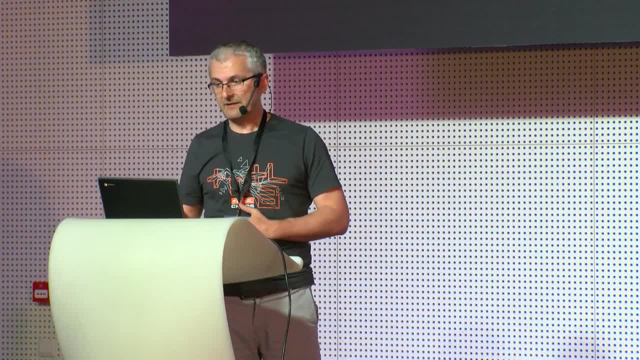 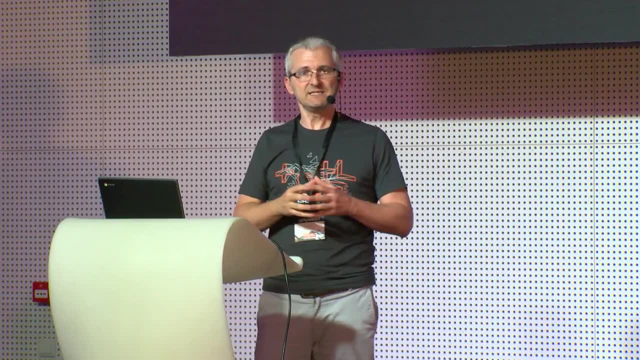 You see how that is done in a second. We do that only to select brainfrac commands. Now the second thing that is related to compiler optimizations is we push the compiler to be very aggressively generating jump tables. And in the third kind of optimization, 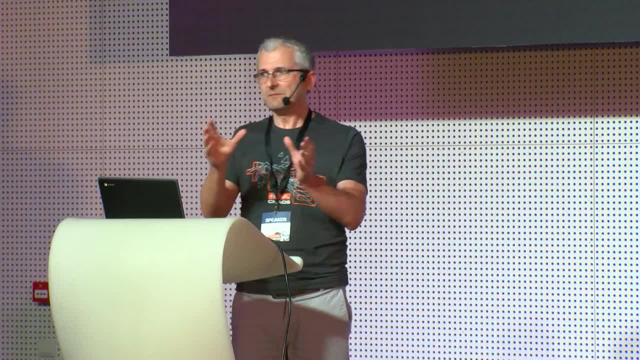 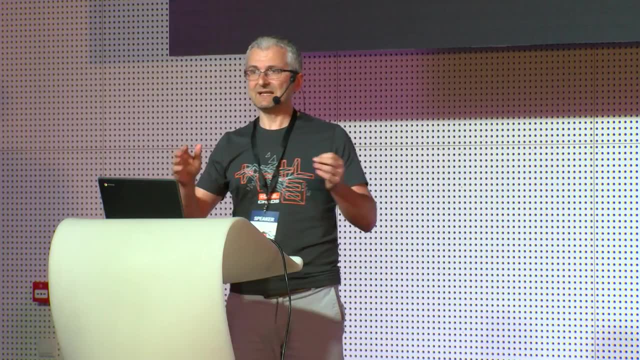 we are actually actively trying to keep our active datum that we work on at any given moment in a register for as long as possible. Now, all participants in that test were tested with all versions of the interpreter loop and the best possible matches were taken. 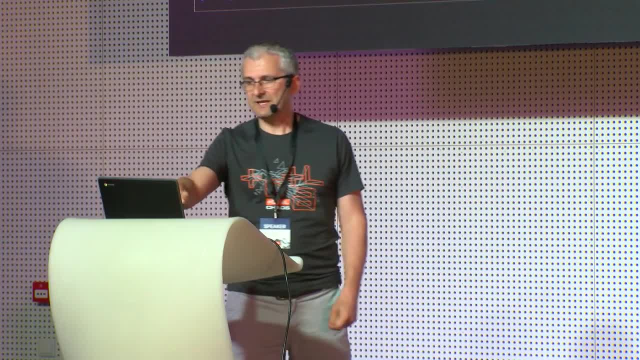 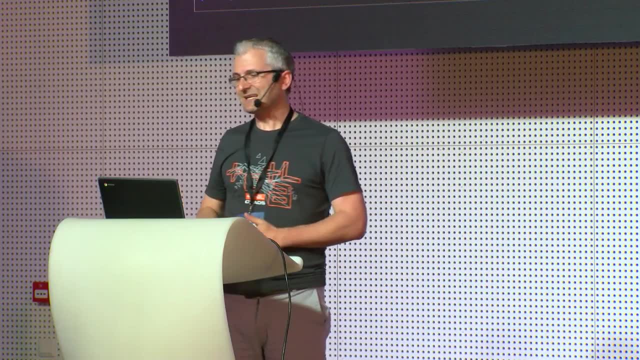 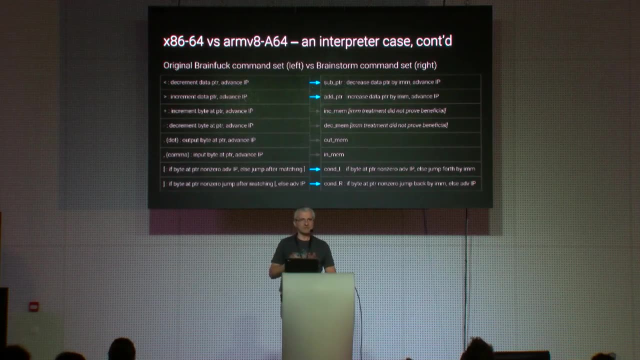 for further analysis. First, again, a clarification of what we changed, what we tweaked in the brainfrac semantics. We actually here, with the cyan highlight, we show the brainfrac commands that we have given the literals treatment, The commands to which we have introduced a literal argument. 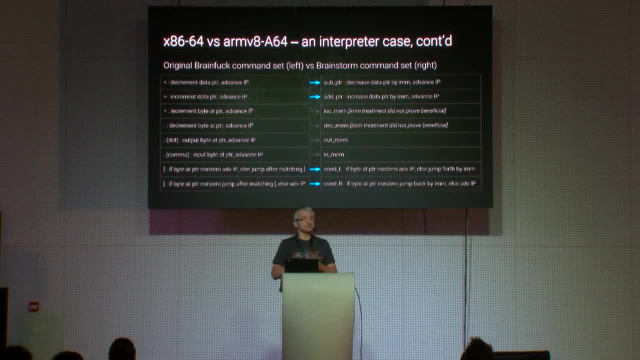 encoded in the command Because brainfrac does not have any kind of other addressing mode, rather than There is only one addressing mode in brainfrac, and this is access the data at this data pointer. Now here we introduce the actual notion of immediate in the operation. 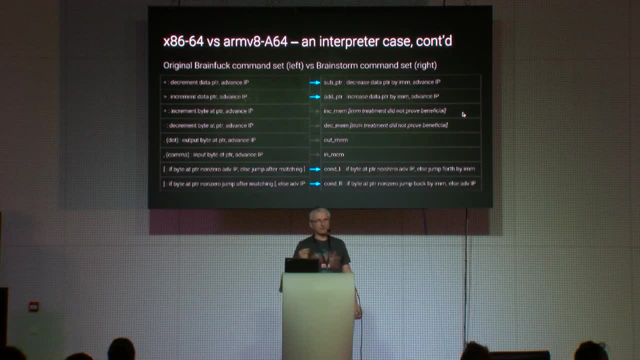 Here I've put a note that even though at first glance it makes sense to also give the immediate treatments to the brainfrac operations that increment the datum at the data pointer, actual tests show that this gives no performance benefit for the most of the test cases. 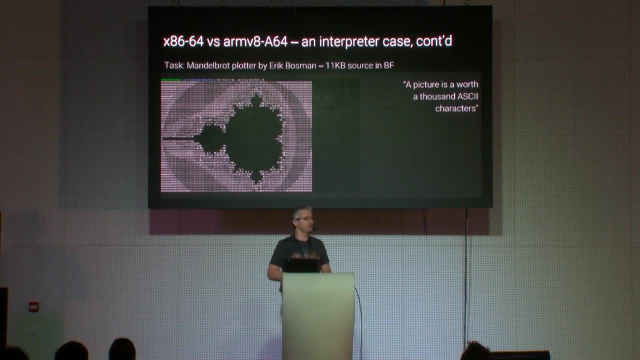 So what are we going to run on our interpreter? There is a very famous piece of code written by Eric Bosman which is an actual Mandelblot plotter, written in brainfrac. The source code of that program is 11 kilobytes. 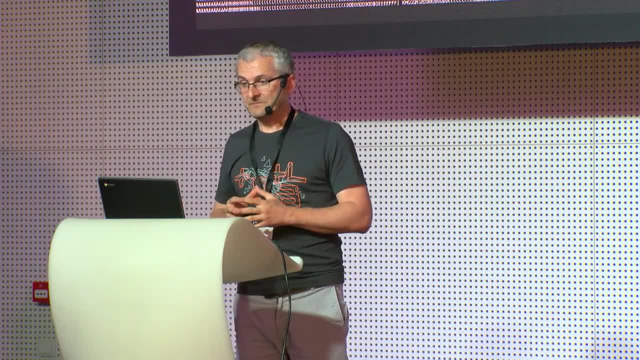 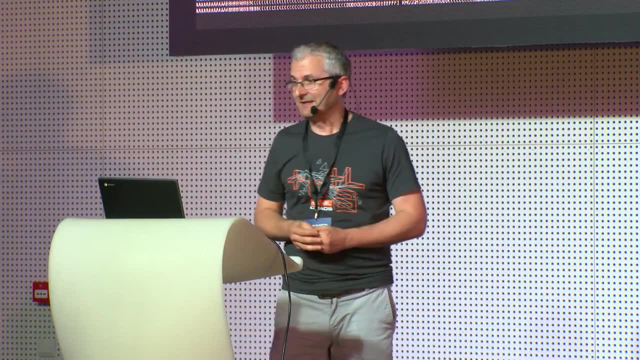 a very dense brainfrac code. It's a really beautiful piece of code. The output of that code is this ASCII art. As they say, a picture is worth a thousand ASCII characters. Uh, So I'll save you the disassembly. 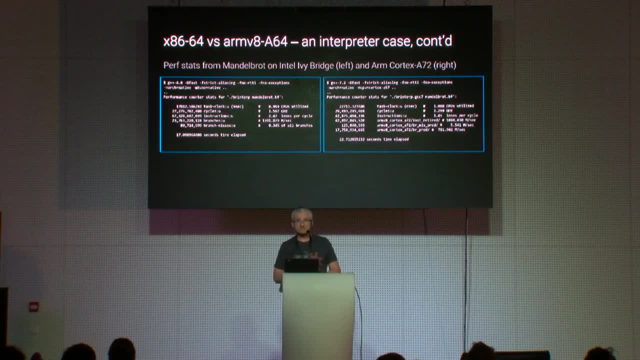 because the disassembly would be much longer and we cannot afford to do this in this session. but I'll just give you the perf stats from running this, running the best case scenarios on each of the two architectures that we are discussing today, And again I'll give you the digest table. 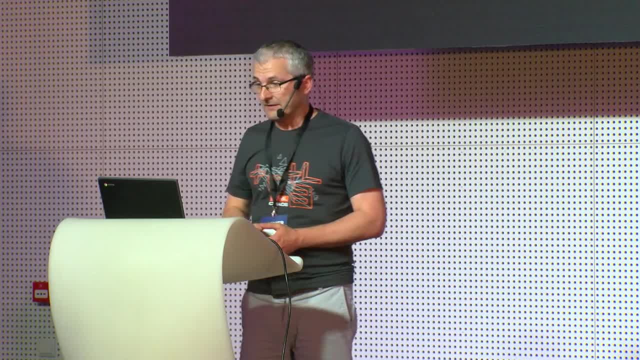 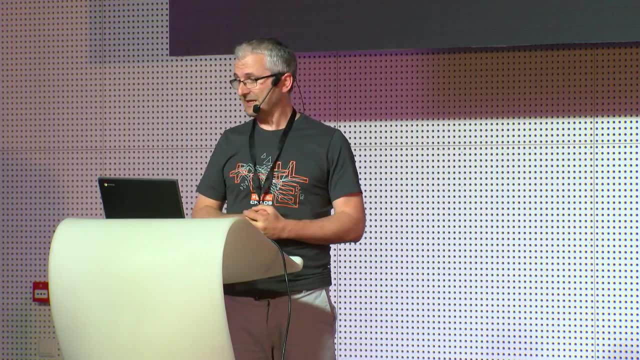 so that you don't have to stare at tiny prints For the interwavy bridge, we have a dynamic instruction count, that is, instructions that were actually executed for the plotting of that nice Mandelblot, Mandelblot, Mandelblot. 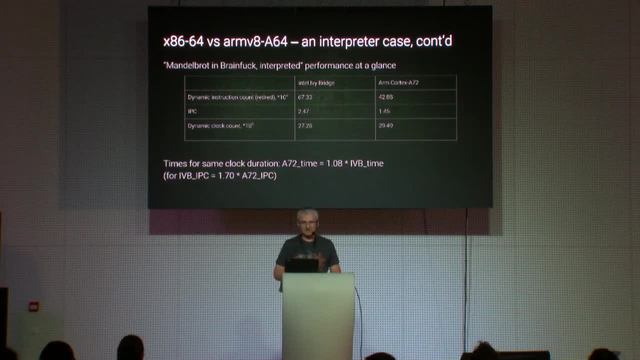 Amounting to 67.33 billion. Again, that was happening at the instructions per clock, equaling 2.47 instructions per clock and eventually amounting to 27 billion clocks. on the Ivy Bridge, On the ARM, we have 42.9 billion dynamic instructions. 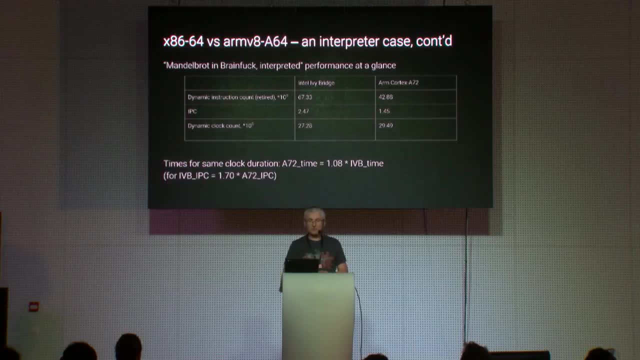 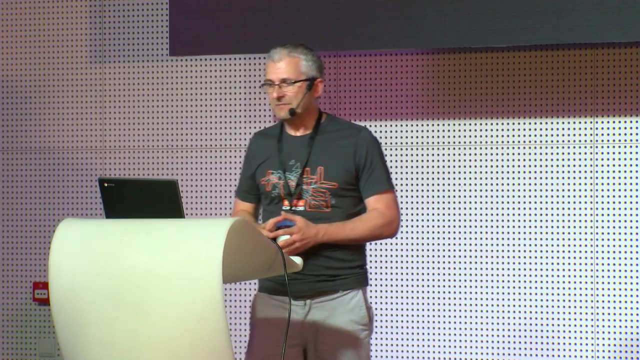 At an IPC of 1.45 instructions per clock, we end up with the dynamic clock count of 29.5 billion. Now, this time the ARM actually loses by 8% if we take the two processors at the same clock. 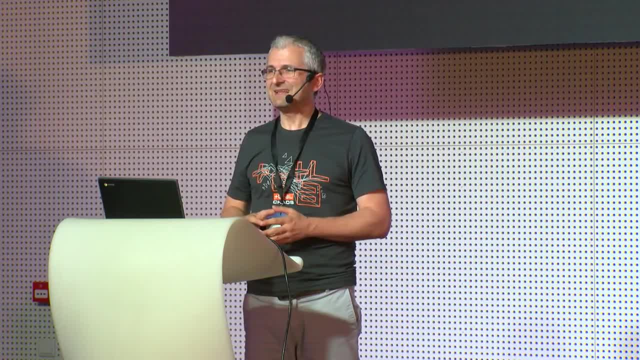 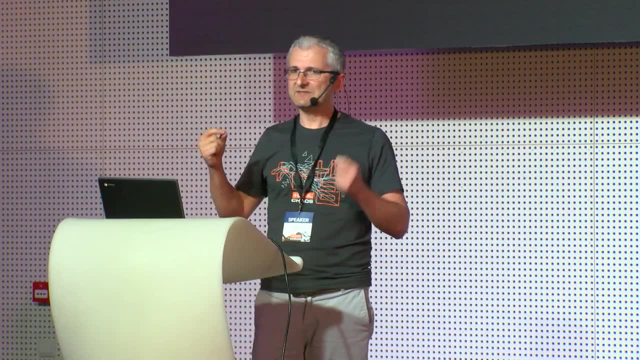 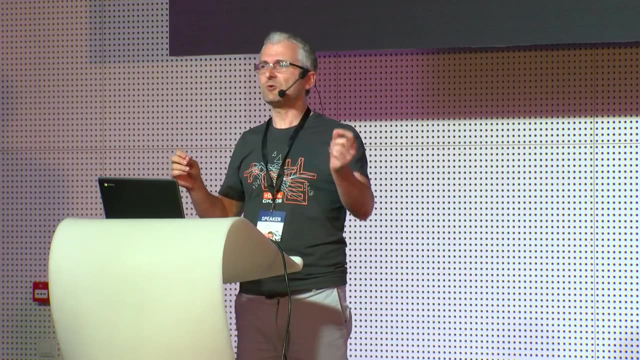 But it loses at 8%, given a disadvantage of instructions per clock of 70% in favor of the Intel. Do you have an idea what a disadvantage of 70% in instructions per clock amounts to? That's comparable to the disadvantage between an in-order CPU and an out-of-order CPU. 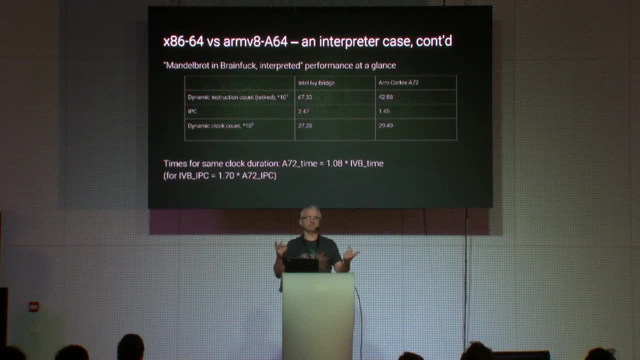 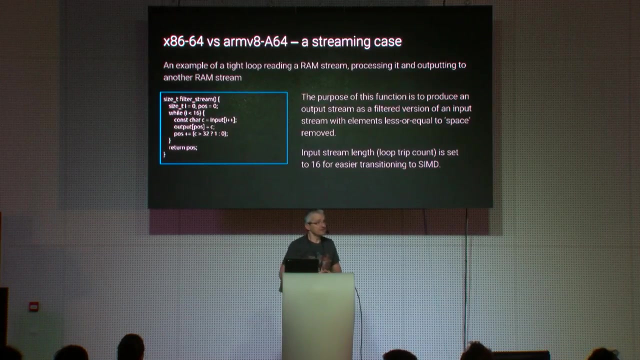 Or a single-issue CPU and a dual-issue CPU. This is a huge disadvantage in instructions per clock And at that huge disadvantage, the ARM is only 8% slower on this task. So let's move on to the next task. Again the final test case for our test study for today. 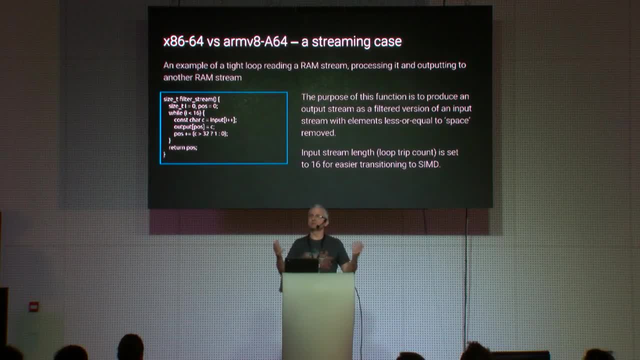 will be again a tight loop. Only this time this tight loop does something useful, in contrast to our first loop. So this loop actually does stream processing. It takes an ASCII stream of ASCIs and filters certain characters out of the stream. Now, what are these characters in this case? 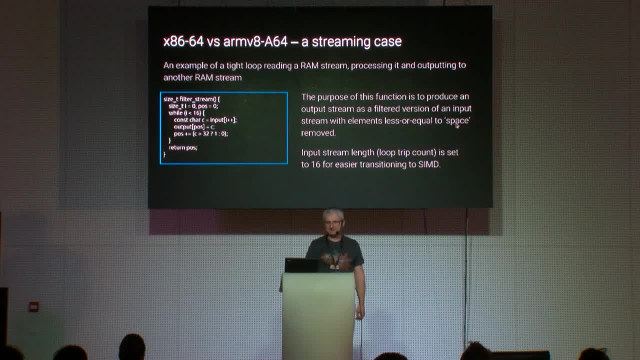 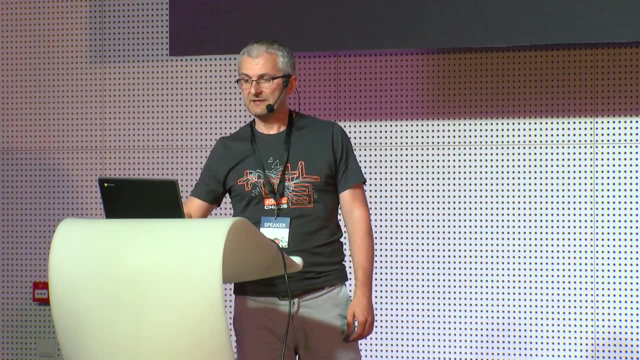 These are all characters that are less or equal to a space. That is ASCII code 32.. Now there is one peculiarity in this code. The peculiarity is that the trip count of our loop is actually fixed at 16.. 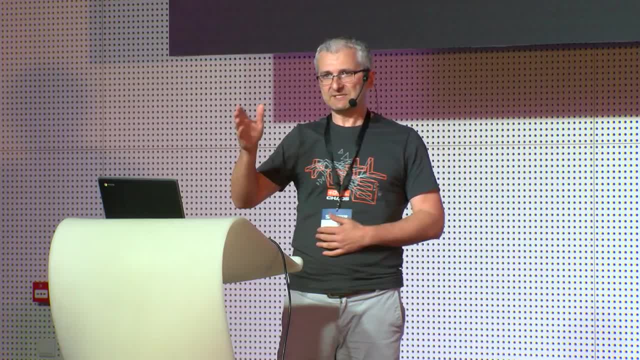 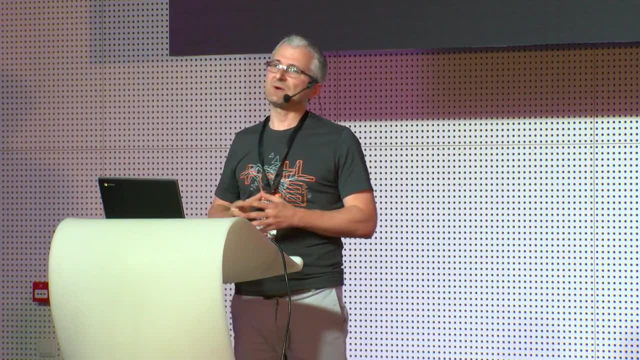 It's not because we expect all input streams to be limited to 16 characters- Sorry, Limited at 16 characters- But because we have written this code with the idea to further vectorize it, and it makes things easier to vectorize when you have such nice division of work. 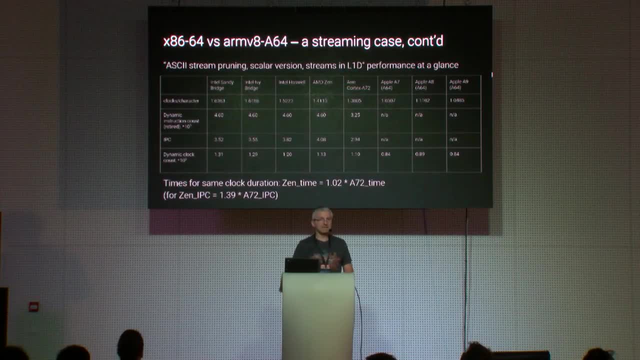 Now. I will save you this time all the disassembly and perf stats, but I'll give you more participants in the digest table. So we have four Intel architecture participants versus four ARM participants. We will introduce a metric here that basically says how many clocks. 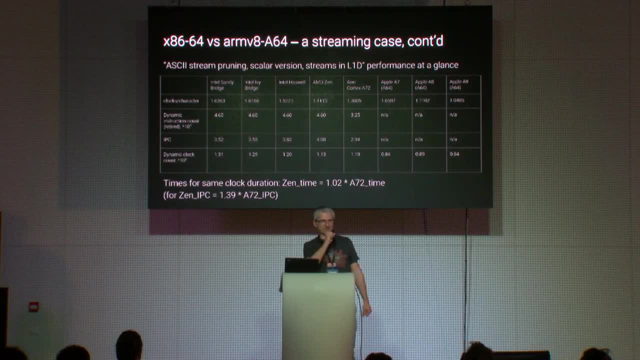 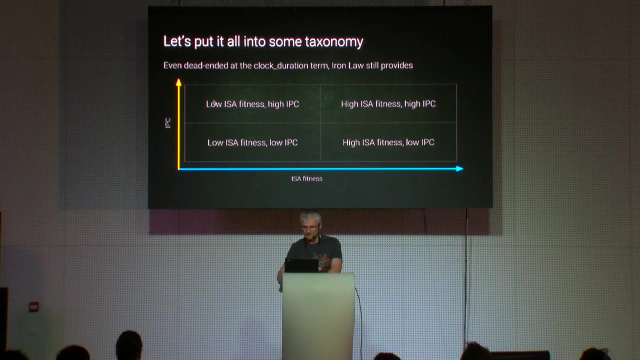 each participant took to process a character And you see that with the improvement of Intel microarchitectures, actually reaching finally to an AMD Zen microarchitecture, the clocks per instruction gradually- Sorry, The clocks per character, sorry- gradually drop, starting from 1.63 clocks per character. 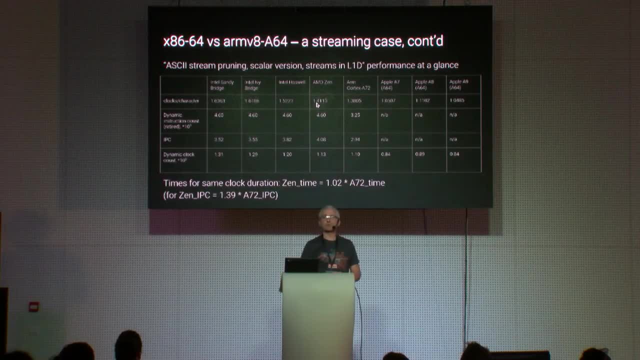 and at the Zen level it's already 1.41 clocks per character. The dynamic instruction counts in the Intel architecture part of the table are essentially the same when rounded to the second digit, the second decimal digit. Why? Because all the compilers that we run. 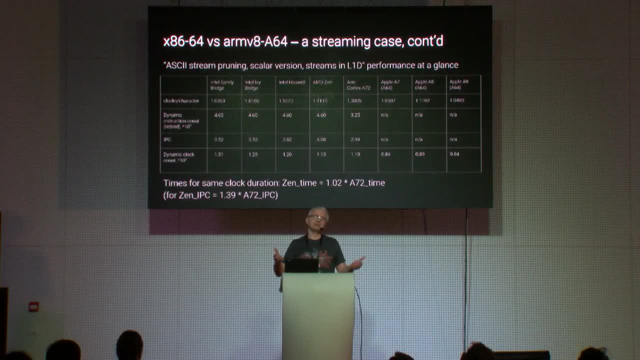 on those microarchitectures produced more or less identical code. So the dynamic instruction count is 4.6 billions for all of our tests. The instructions per count, on the other hand, again start with 3.52 on the IAM. 3.52 on the Ivy Bridge and gradually rise to the astonishing 4.1 on the AMD Zen. The AMD Zen does magnificently this test. An IPC above 4 is something pretty, pretty desirable. And the dynamic clocks again. 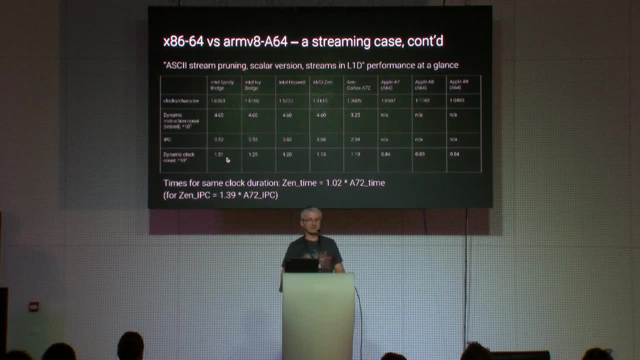 as a result of those instructions per clock start from 1.32 billion for the Ivy Bridge and drop down to 1.13 billion for the Zen. What happens in the right-hand side of the table? First, I would like to apologize. 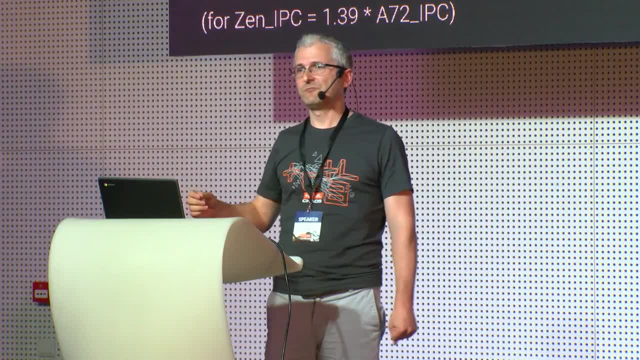 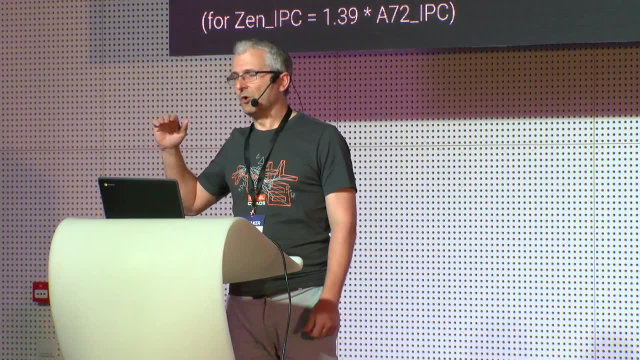 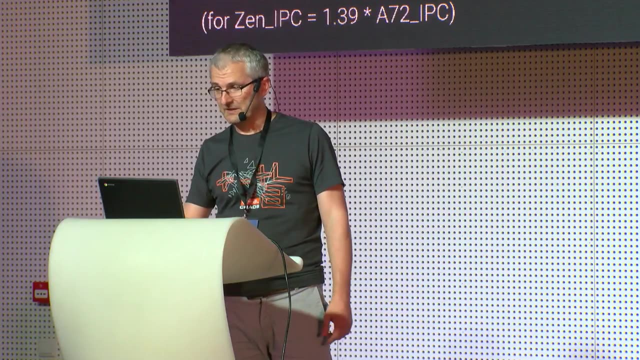 because for all the Apple participants in this table I didn't have proper profiler, so all the numbers here have been devised from the actual execution times and known clocks of the CPU. I didn't actually have the measured dynamic instruction counts, but I haven't tried to devise them. 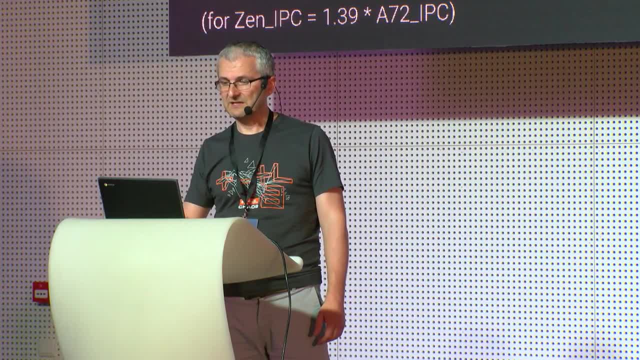 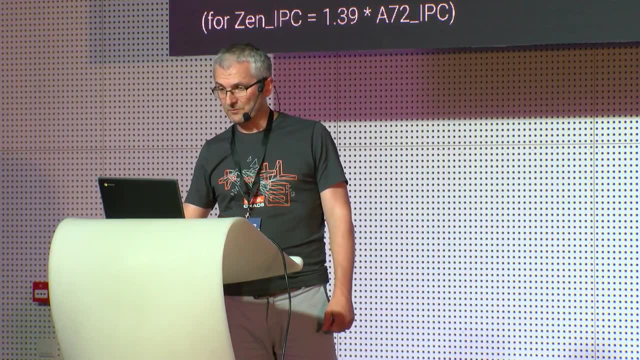 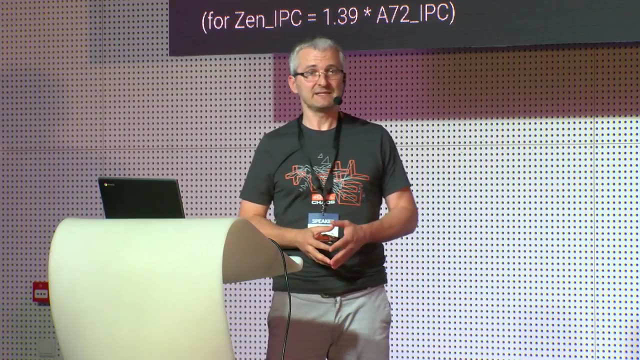 I have devised just the clocks per character metrics and the dynamic clock count, which is a simple function of multiplication of clock by a time span. So let's take a look at the ARM Cortex-A72.. For something that took 4.6 billion dynamic instructions. 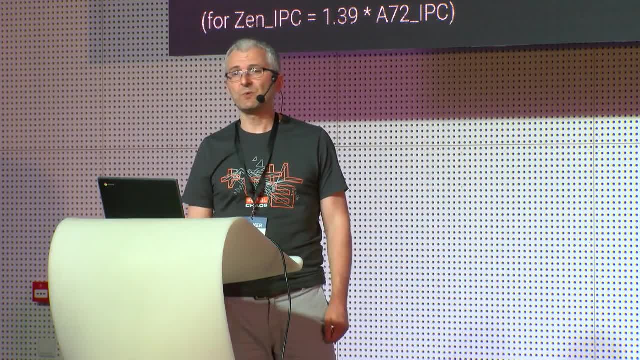 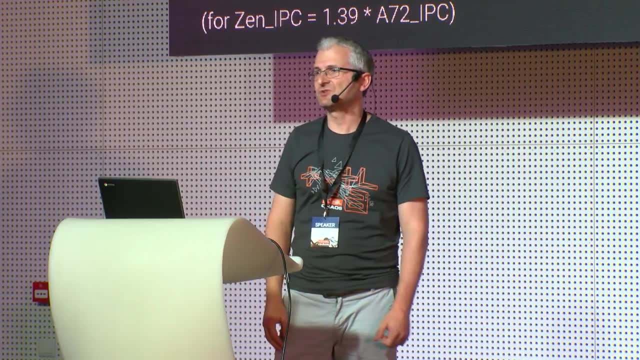 on the Intel side of the architectures it takes 3.25 billion instructions on the ARM side of the table Now, at an IPC of 2.94 instructions per clock, which is very close to the hypothetical maximum of the ARM, except for some special cases. 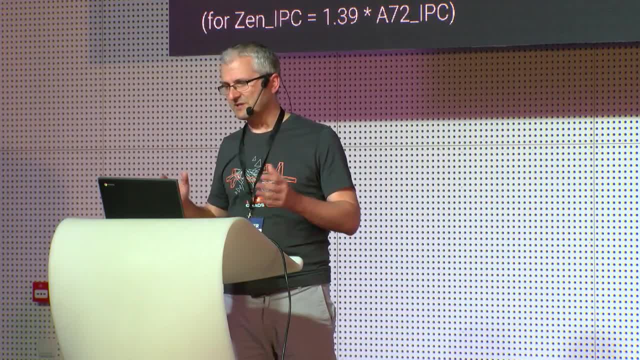 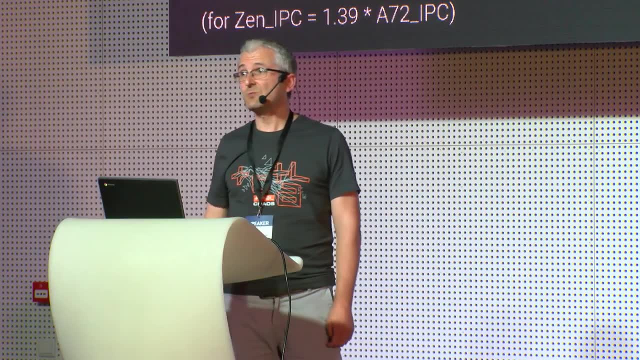 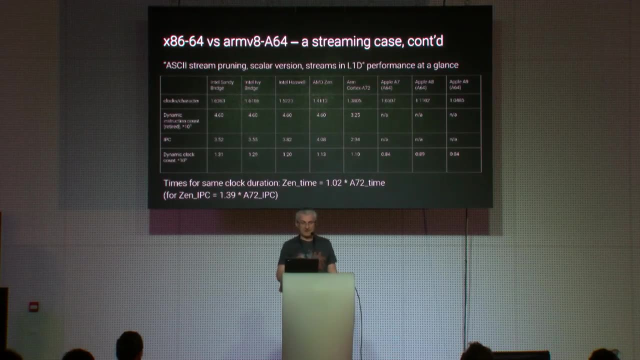 where I could deliver five instructions per clock, but those are really exceptional cases. we actually get a dynamic clock count of a billion and one tenth. A billion and one tenth is 2%. better than the best Intel microarchitecture. Not only it's better than the best. 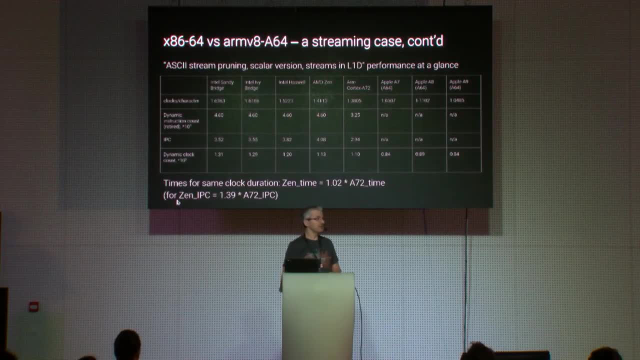 Intel microarchitecture, but it also comes at a 40% disadvantage in instructions per clock, So I think that this is a pretty good indicator. I mean, I will not even be discussing the Apple participants because, as I said, I don't have the correct data set on them. 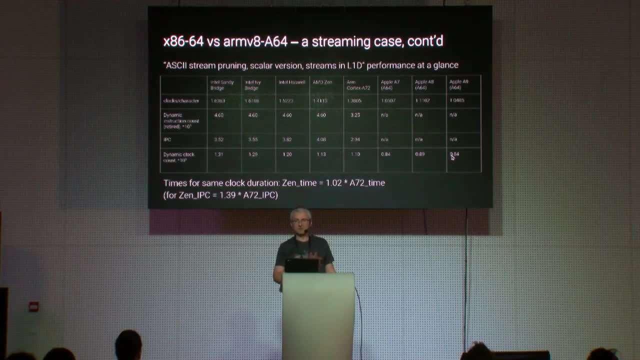 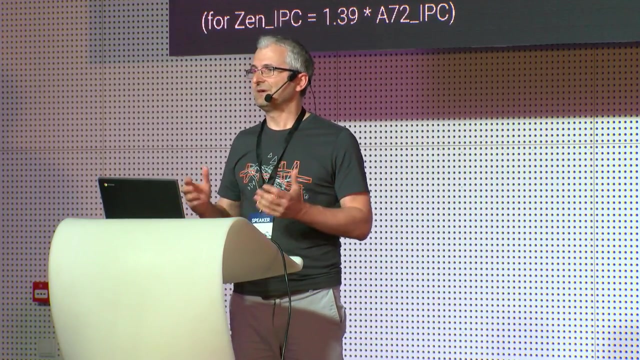 but you can imagine that with these numbers going down to below one billion clocks for the task they are performing pretty damn well. So what can we say about general instructions? I mean the general importance of ISA fitness for a purpose. It actually makes a pretty damn good sense. 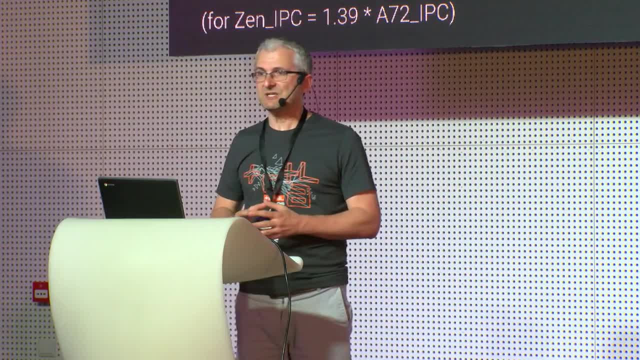 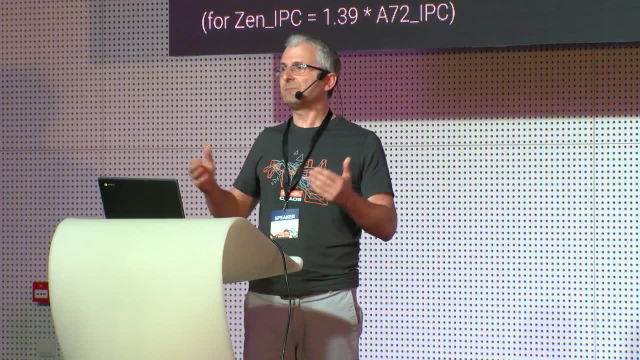 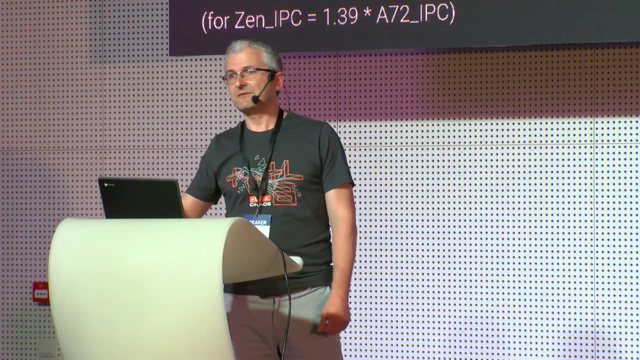 It makes sense that architecture- sorry, ISA architecture, I mean all these architects- put a very good effort into providing an instruction set architecture that is up to date with our understanding of modern general purpose programming, because all of these test cases were randomly picked, frankly. 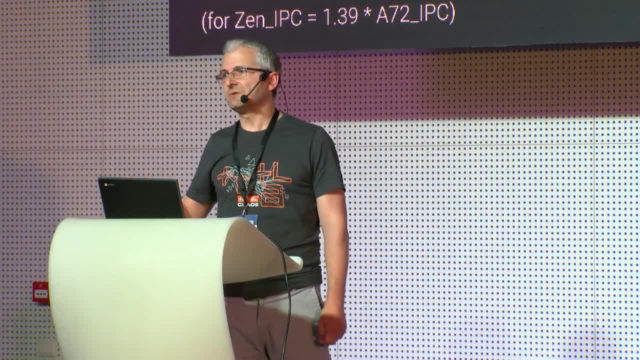 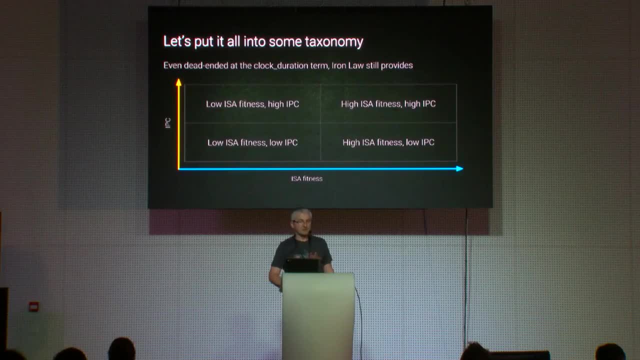 I was doing some research on my own on the site and I just noticed this trend in my results. So what can we say about the iron law of performance? Can we just produce some taxonomy that gives us a general idea of how we can improve performance? 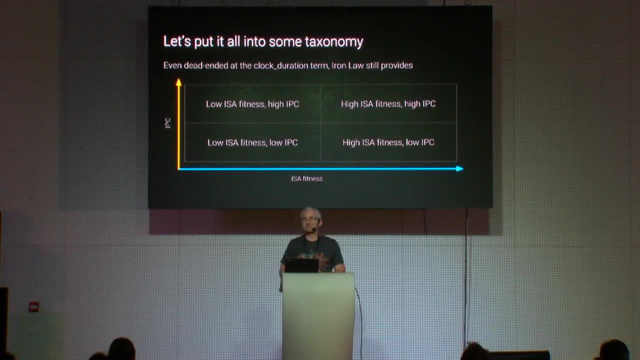 given that one of the terms of the iron law of performance has dead ended, And this is the clock term. Well, we actually can If we take a graph that we put on the horizontal the ISA fitness and on the vertical the instructions per clock. 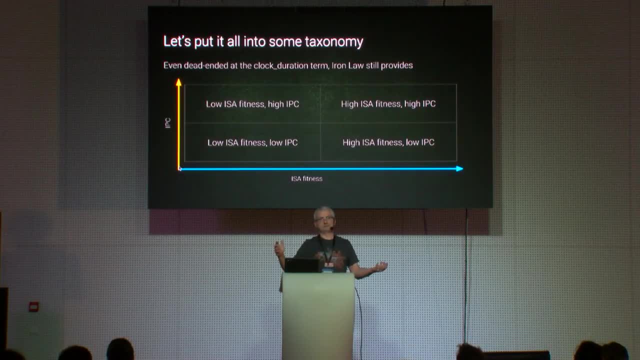 then here at the origin, we have zero performance, or performance close to zero, and here, at the opposite end of the spectrum, we have optimal performance for sequential programming. So the opposite end of the spectrum is where you want to be. 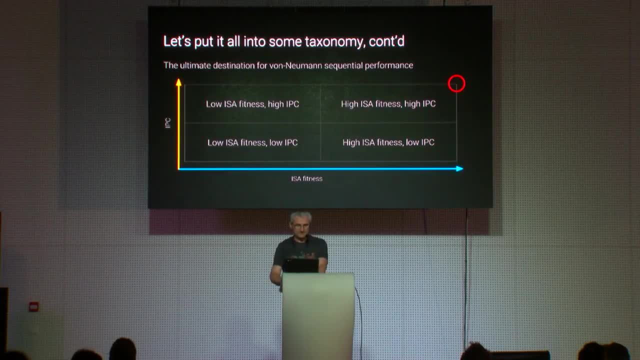 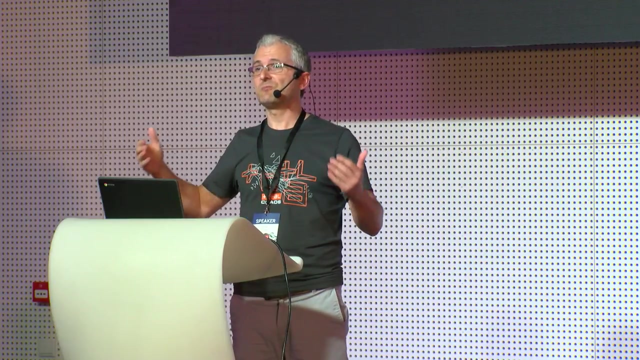 in terms of single-thread performance. Now, when speaking of massively parallel architectures, though, it perhaps makes sense to slightly scale down on the instructions per clock, because instructions per clock just give us instruction-level parallelism In massively parallel processors. we have other, more beneficial forms of parallelism. 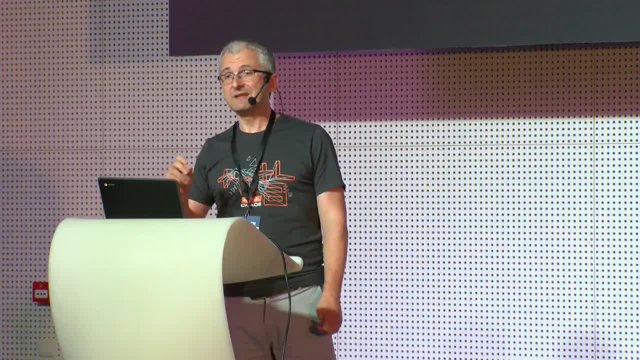 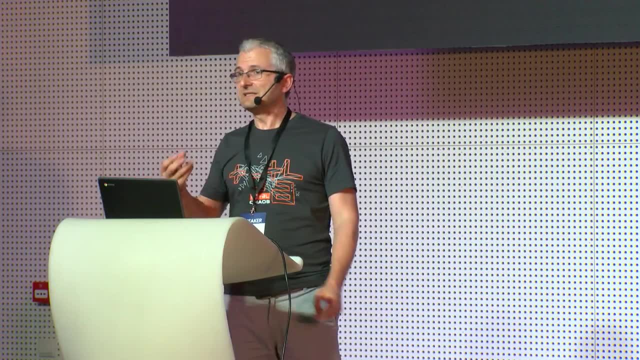 that we could take advantage of. So if we can actually scale down a bit the instruction-level parallelism as a trade-off for better task-level parallelism- basically a simpler course that we can put more of them on a single die- we could actually end up with a net benefit.